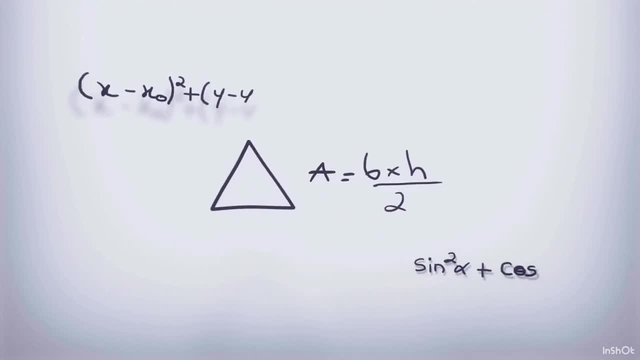 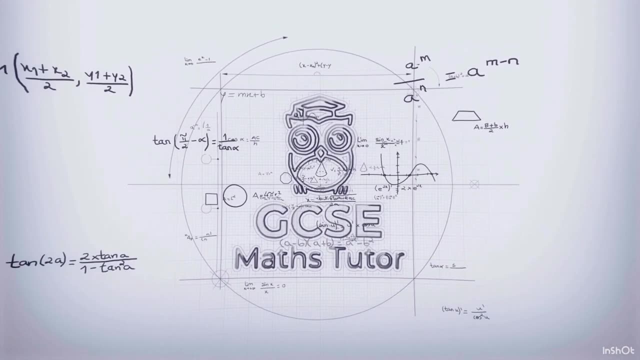 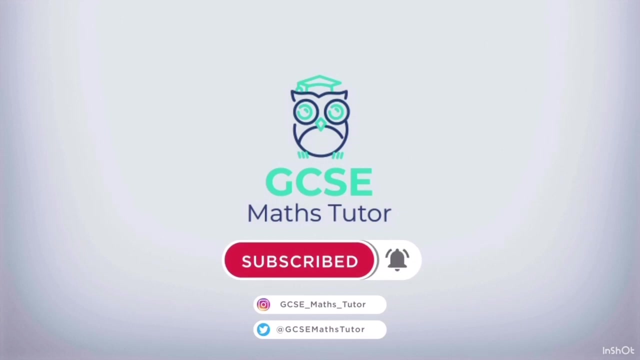 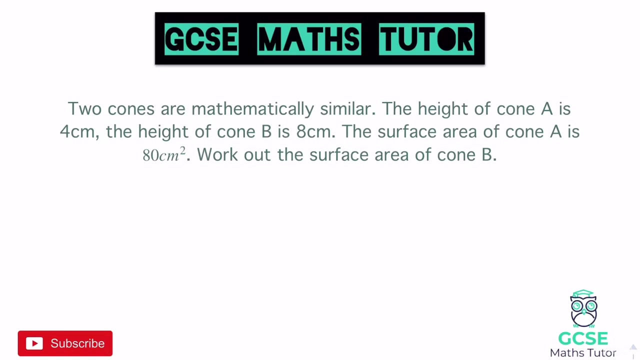 Right, so we're going to have a look at similar shapes, looking at area and volume. I'm not going to be having a look at any of the just standard length similar shape questions here, but we are just going to be focusing on when we're using area and volume and what happens. 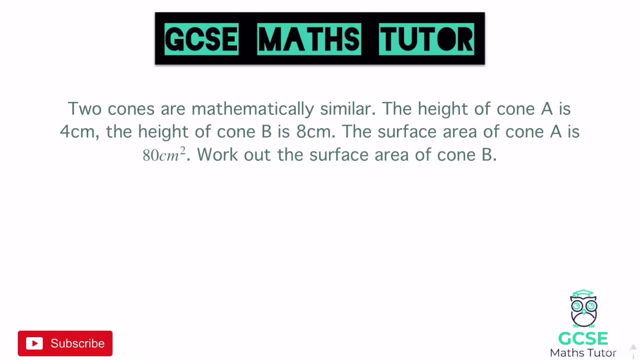 to the scale factors within these. Okay, so we're going to get started with this question. So grab a piece of paper, grab a pen, make some notes. I'm going to kick this off with this one. So two cones are mathematically similar. The height of cone A is four centimetres and the height of cone 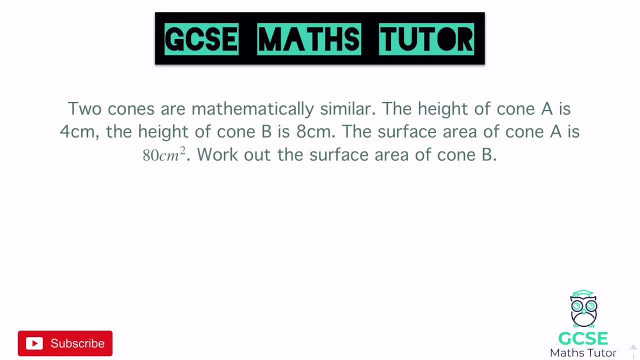 B is eight centimetres. Then it says the surface area of cone A is 80 centimetres squared. Look at the surface area of cone B Now. it may or may not give you a diagram for these. If it doesn't. 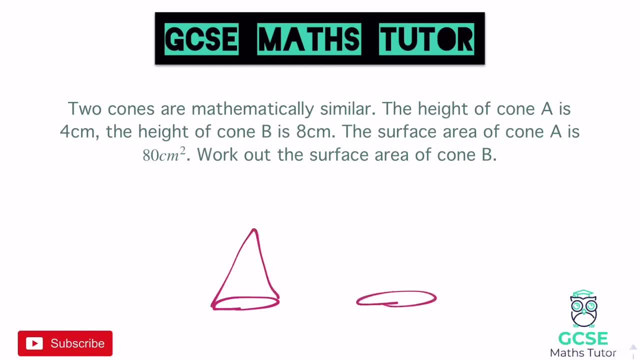 it can help just to do a little drawing. Okay, they don't have to be perfect, Just some little cones that we can label A and B and start to just visualise this a little bit. Now it says the height of A, which would be this, is four centimetres and the height of B, which is here, is eight. 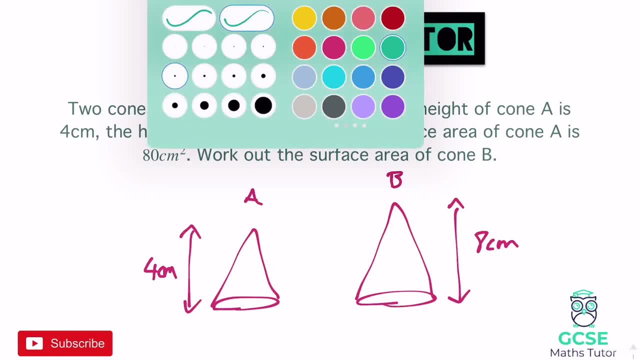 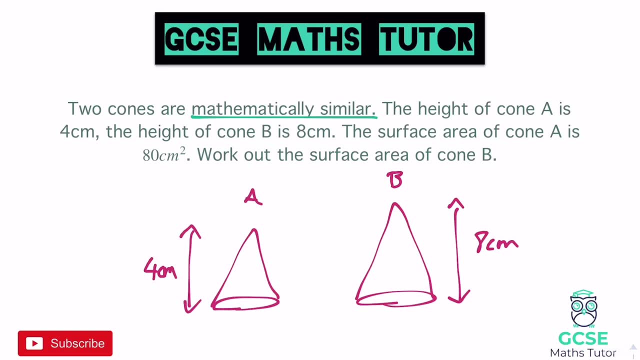 centimetres. Now, whenever you're trying to find similar shapes, this wording mathematically similar means that one is an enlargement of the other And when something's been enlarged, it's been enlarged by a scale factor. And the way to find that scale factor is identify the 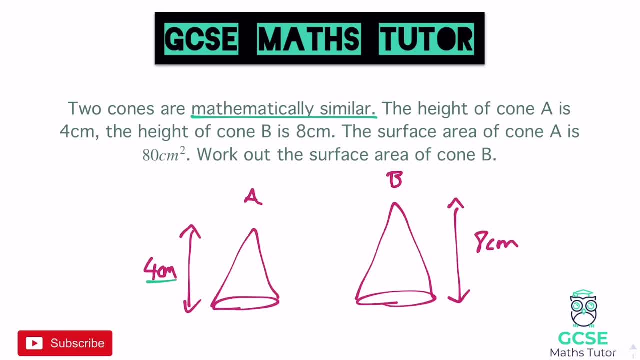 common lengths on both, which in this case is the height, here four and eight, And you do, the big one divided by the little one, or the big length there divided by the little lengths, So eight being the big lengths divided by four the smaller one. 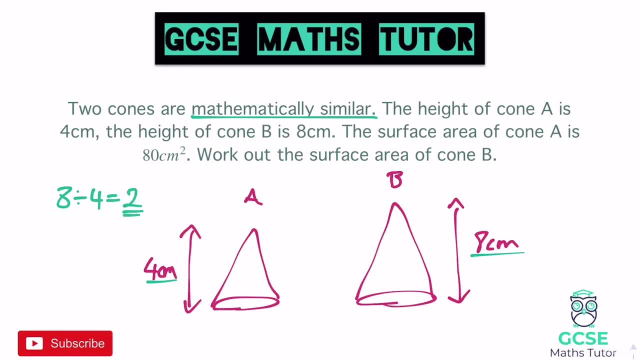 Gives us an answer of two, And that is our scale factor. Now, when it comes to looking at lengths, areas and volumes, we refer to these scale factors- or I certainly do- in different ways. Now I call this one my length scale factor. So I always write down LSF. just something for. 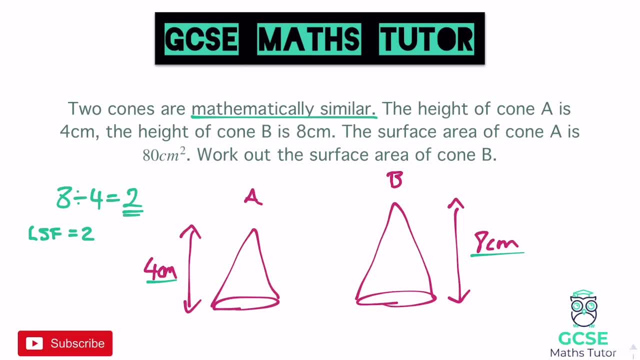 length scale factor, and that equals two. Now, when I'm dealing with these questions, we're either going to be looking for an area scale factor, which I call ASF, or a volume scale factor, which you can probably guess V. Now, in this question it does actually mention. let's just have another quick look. it says the: 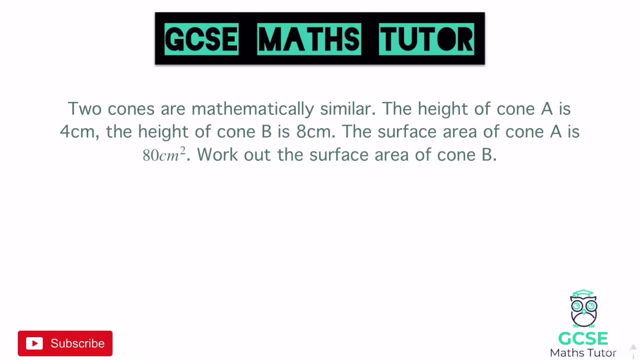 to the scale factors within these. Okay, so we're going to get started with this question. So grab a piece of paper, grab a pen, make some notes. I'm going to kick this off with this one. So two cones are mathematically similar. The height of cone A is four centimetres and the height of cone 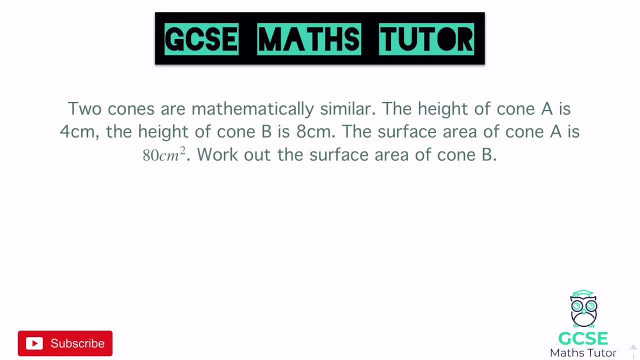 B is eight centimetres. Then it says the surface area of cone A is 80 centimetres squared. Look at the surface area of cone B Now. it may or may not give you a diagram for these. If it doesn't. 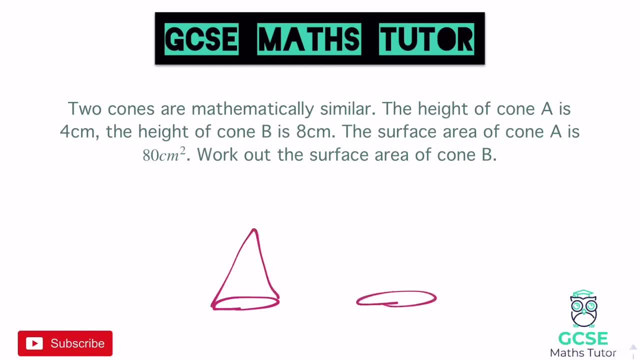 it can help just to do a little drawing. Okay, they don't have to be perfect, Just some little cones that we can label A and B and start to just visualise this a little bit. Now it says the height of A, which would be this, is four centimetres and the height of B, which is here, is eight. 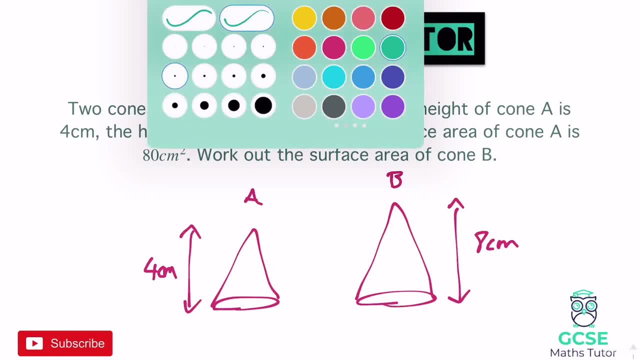 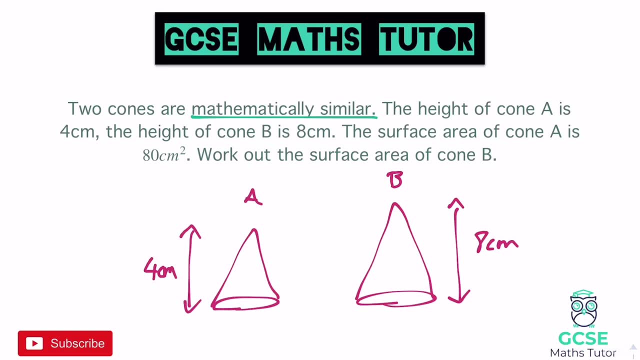 centimetres. Now, whenever you're trying to find similar shapes, this wording mathematically similar means that one is an enlargement of the other And when something's been enlarged, it's been enlarged by a scale factor. And the way to find that scale factor is identify the 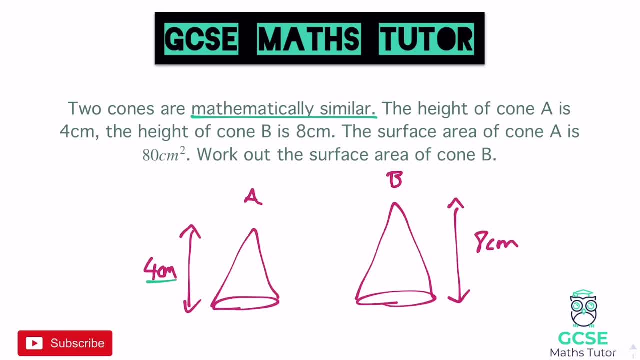 common lengths on both, which in this case is the height, here four and eight, And you do, the big one divided by the little one, or the big length there divided by the little lengths, So eight being the big lengths divided by four the smaller one. 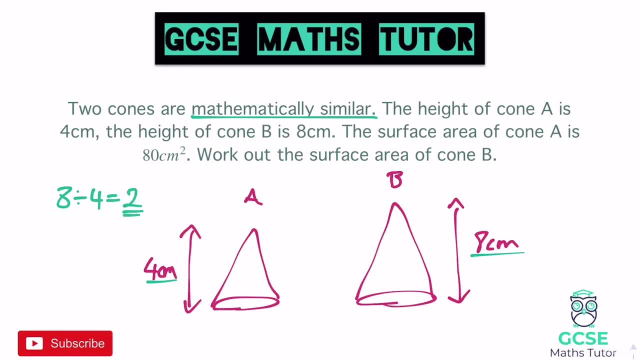 Gives us an answer of two, And that is our scale factor. Now, when it comes to looking at lengths, areas and volumes, we refer to these scale factors- or I certainly do- in different ways. Now I call this one my length scale factor. So I always write down LSF. just something for. 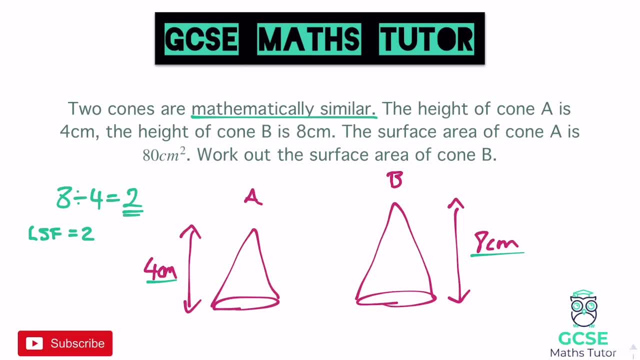 length scale factor, and that equals two. Now, when I'm dealing with these questions, we're either going to be looking for an area scale factor, which I call ASF, or a volume scale factor, which you can probably guess V. Now, in this question it does actually mention. let's just have another quick look. it says the: 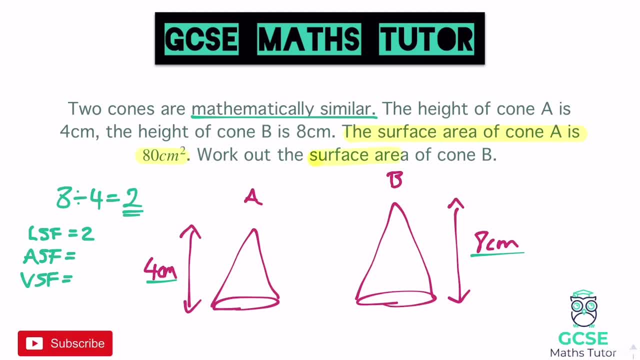 surface area of A is 80, work out the surface area of B. So we are actually trying to work out an area here. so I don't actually need the volume scale factor, but I do need the area scale factor. Now to get from length to area, the scale factor itself, the only thing we have to do is take the 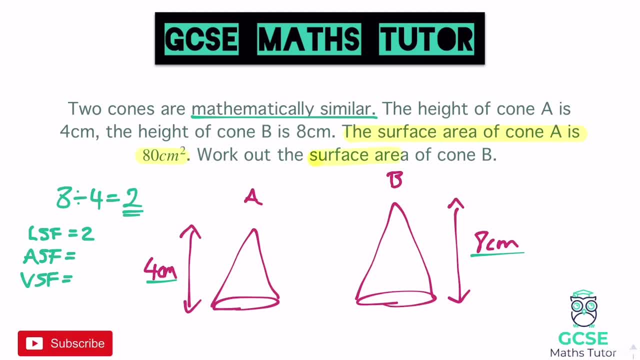 surface area of A is 80, work out the surface area of B. So we are actually trying to work out an area here. so I don't actually need the volume scale factor, but I do need the area scale factor. Now to get from length to area, the scale factor itself, the only thing we have to do is take the 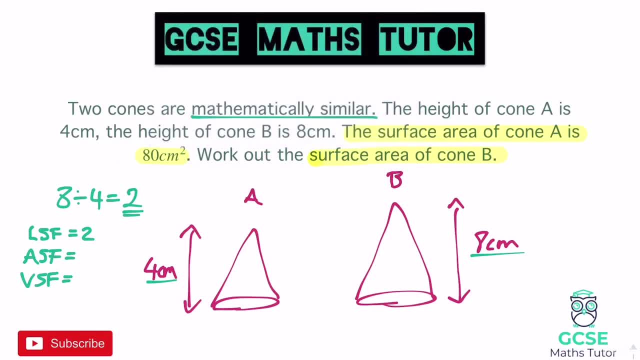 length scale factor and square it. Just think about the units there. squared is in the units, So to get from length to area, the length scale factor is in the units. So to get from length to area, we just need to square that. There we go, So it would be two squared and two squared. 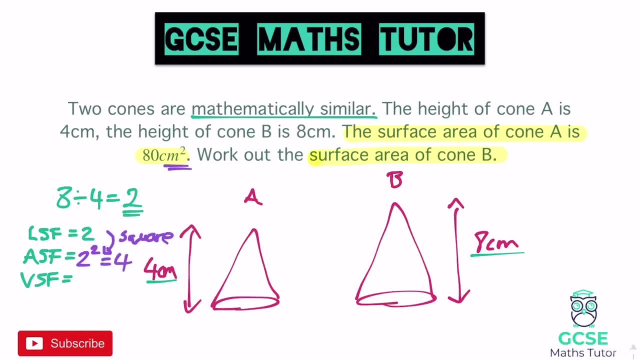 is four. So my area scale factor that we're going to use is four, And that would also work if I wanted to go down to volume. Think about the units in volume centimetre cubed, you would cube the scale factor, So it would be two cubed, The volume scale factor will. 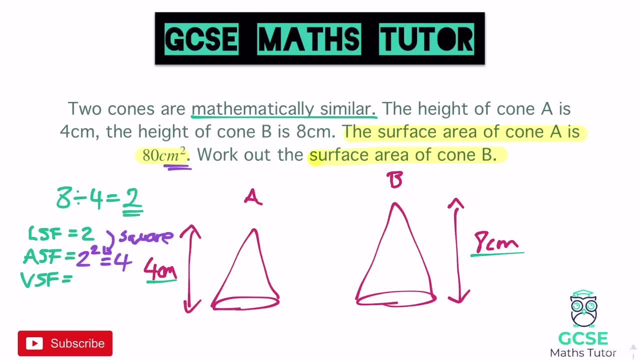 be eight. So all we got to do is move between the scale factors. for the one we want, As we're, we're trying to work out a surface area here- we have to use the area scale factor. So it says here that the surface area of A, which is my smaller cone here, let's just label this the 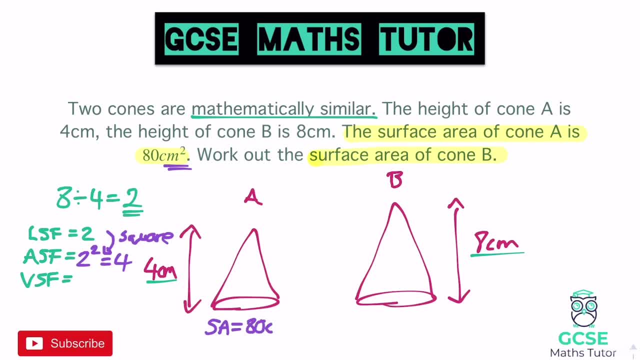 surface area equals 80 centimetres squared and we are going to try and find out what the surface area of B is. Now, B is the larger shape. so to get from A to B I'm going to multiply by the scale factor. so multiply by 4 that area scale factor and 80 times 4, and again you may or may not have. 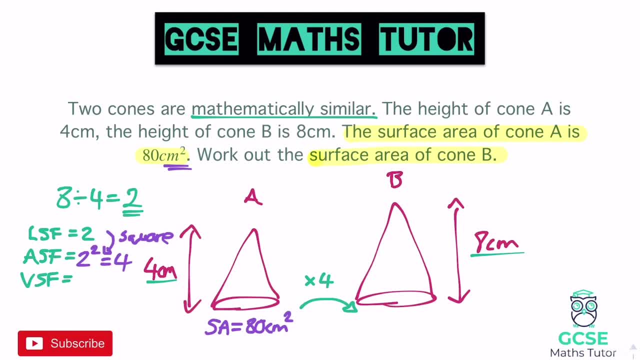 a calculator for some of these, Some of these. you're definitely going to have one, but we could do that without a calculator. 80 times 4 is 320 centimetres squared, and that there is our final answer: 320 centimetres squared. Okay, so we're going to have a look at a few of these, but the 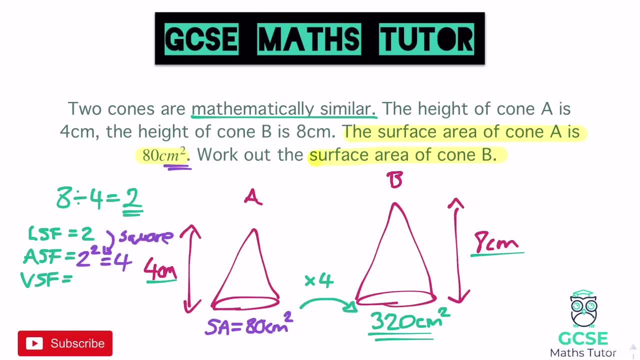 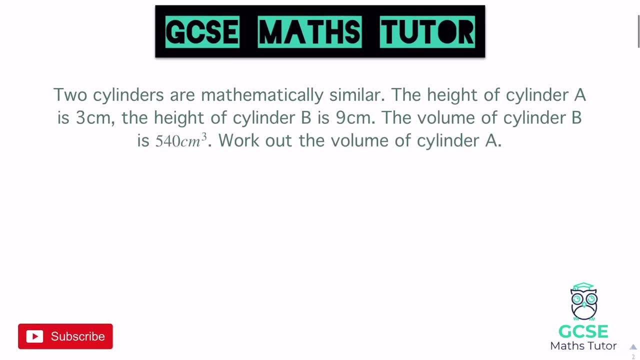 essential part there is obviously finding the big and dividing it by the little. In this case it was length, so 8 divided by 4.. Give us a length scale factor of 2 and then converting that into an area or a volume scale factor by squaring or cubing your length scale factor. Let's have a look at one more. Okay, so in 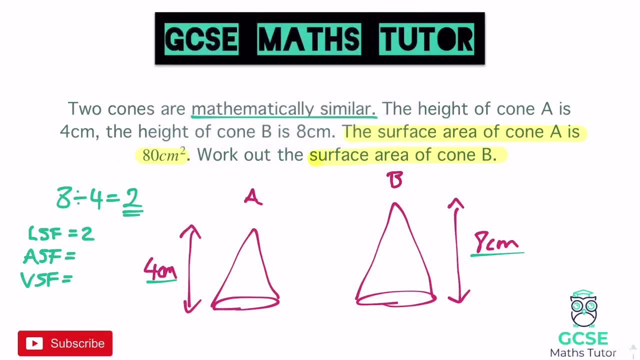 length scale factor and square it. Just think about the units there. squared is in the units. So to get from length to area, the length scale factor is in the units. So to get from length to area, we just need to square that. There we go, so it'll be two squared, and two squared is four. 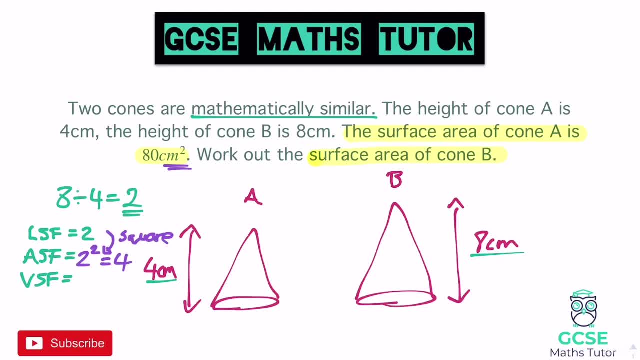 So my area scale factor that we're going to use is four, And that would also work if I wanted to go down to volume. Think about the units in volume centimetre cubed. you would cube the scale factor, So it'd be two. cubed, the volume scale factor will be eight. So all we've got to do is move. 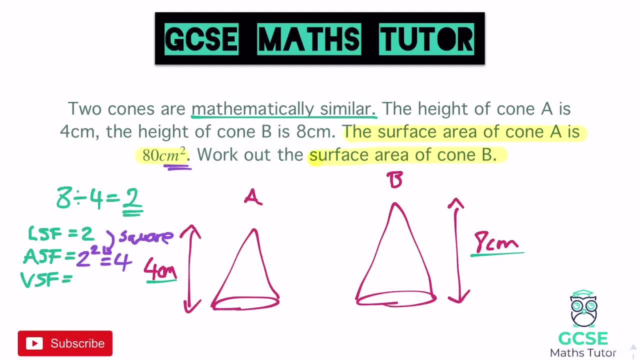 between the scale factors for the one we want. So we've got to move between the scale factors for the one we want and so we're trying to work out a surface area. here we have to use the area scale factor, okay, so it says here that the 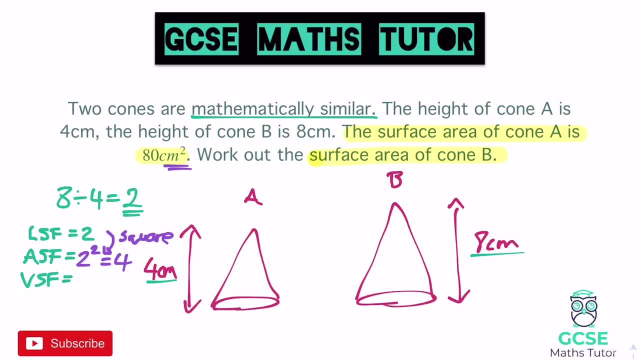 surface area of a, which is my smaller cone here. let's just label this. the surface area equals 80 centimeters squared, and we are going to try and find out what the surface area of b is now. b is the larger shape, so to get from a to b, i'm going to multiply by the scale factor. 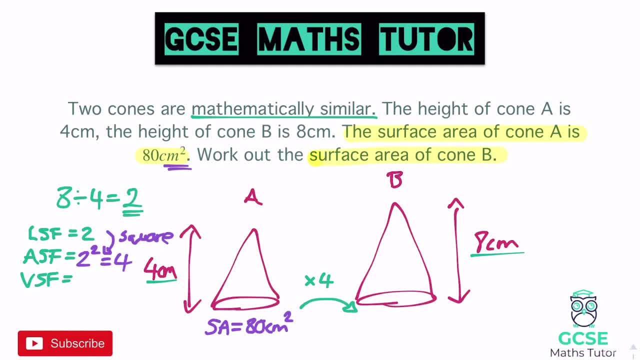 so multiply by four that area scale factor, and 80 times four. and again, you may or may not have a calculator for some of these. some of these you're definitely going to have one. we could do that without a calculator. 80 times four is 320 centimeters squared. and that there is our final. 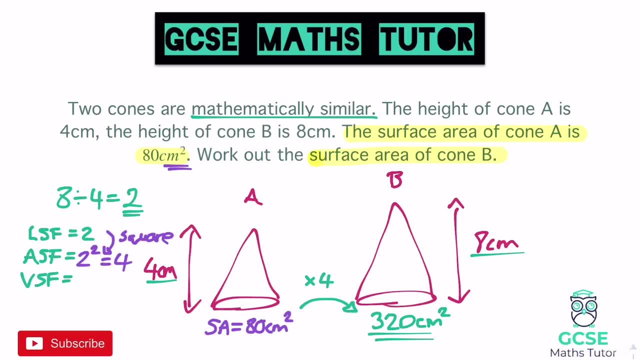 answer: 320 centimeters squared. okay, so we're going to have a look at a few of these, but the essential part there is obviously finding the big and dividing it by the little. in this case it was length. so eight divided by four gives us a length scale factor of two, and then converting that into an area or a volume scale factor by 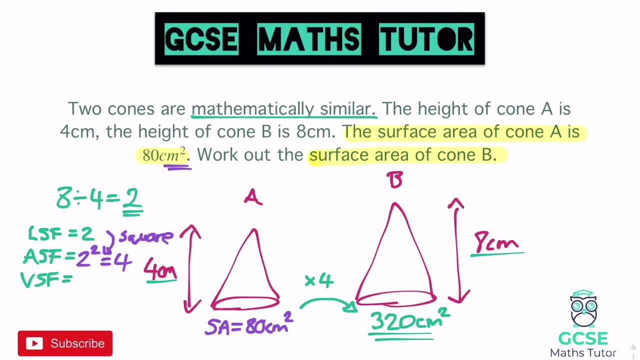 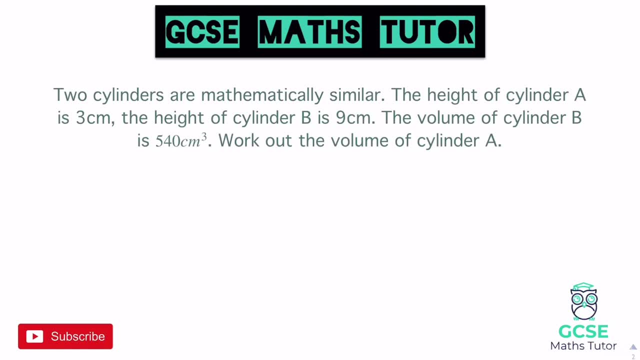 squaring or cubing your length scale factor. let's have a look at one more. okay, so in this question it says two cylinders are mathematically similar. the height of cylinder a is three and the height of cylinder b is nine. the volume of cylinder b is 540 centimeter cubed. work out the volume of 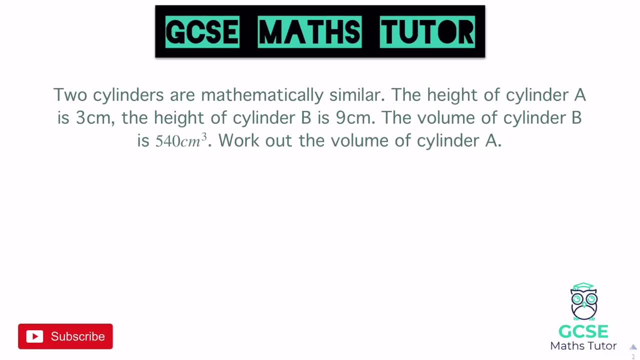 cylinder a. so again, there's no pictures again which it may or may not give to you, but i can easily draw one, and it doesn't have to be perfect. so let's call this cylinder a and let's call this one cylinder b, which i'm going to draw just a little. 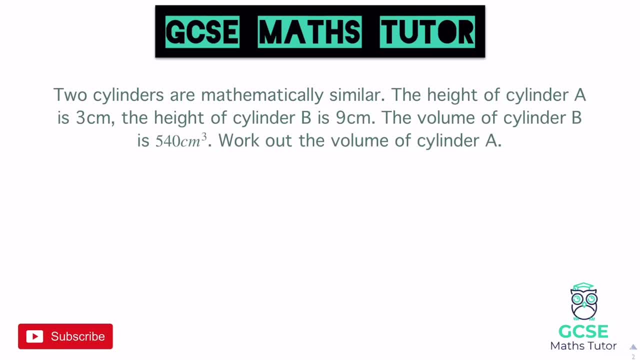 this question. it says two cylinders are mathematically similar. The height of cylinder A is 3 and the height of cylinder B is 9.. The volume of cylinder B is 540 centimetre cubed. Work out the volume of cylinder A. So again there's no pictures again which it may or may not give to. 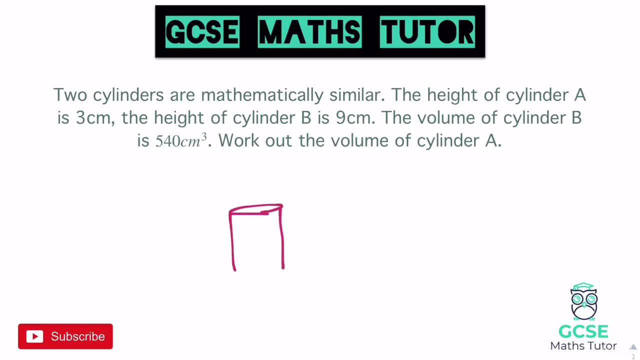 you, but I can easily draw one, and it doesn't have to be perfect. Let's call this cylinder A and let's call this one cylinder B, which I'm going to draw just a little bit bigger there, because I can see that the height of that is 9 rather than 3.. Again, this isn't a. 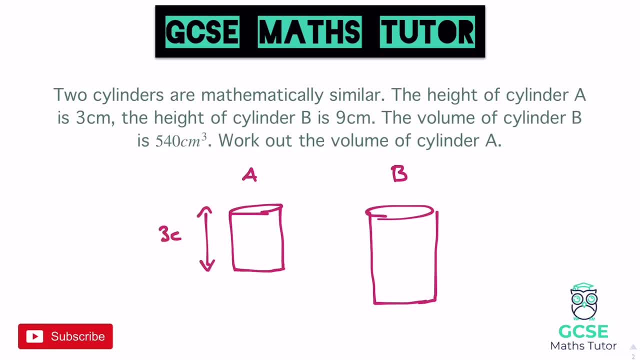 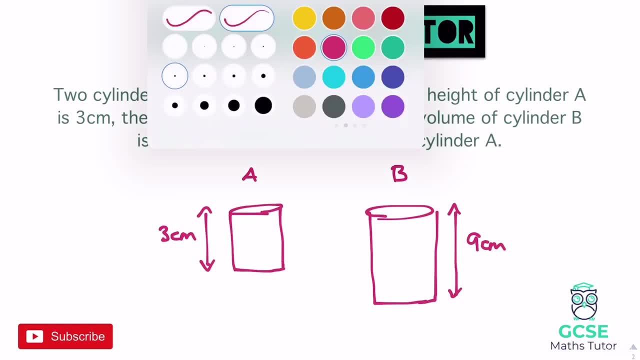 scale. it's just to give you a little visual idea. So this is 3 centimetres as the height of A and this is 9 centimetres for the height of B. Now it does also give us another piece of information, so let's write that on. It says 540 centimetre cubed. 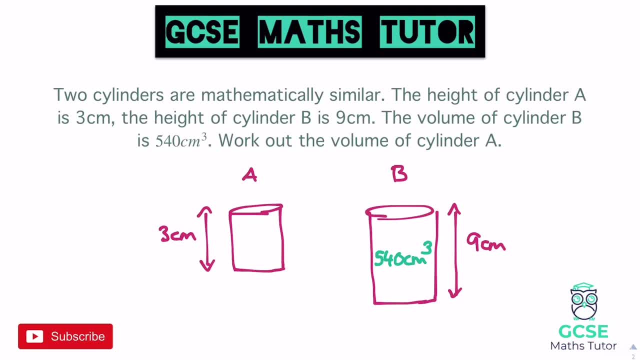 For the volume of B there. okay, just making sure you label that appropriately. Okay, it's always a good idea to highlight some of the information: Height of A is 3, height of B is 9 and then the volume of B is 540.. We're going to work out the volume of A. So, again, we just need to work out. 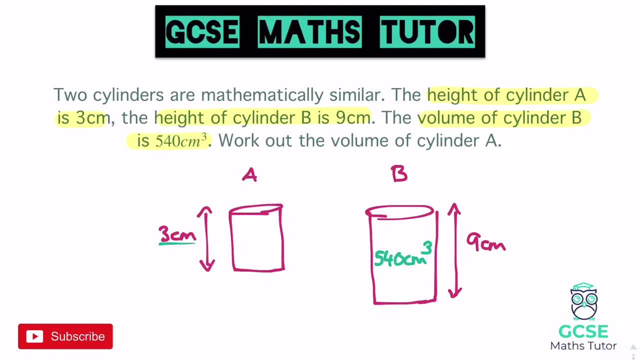 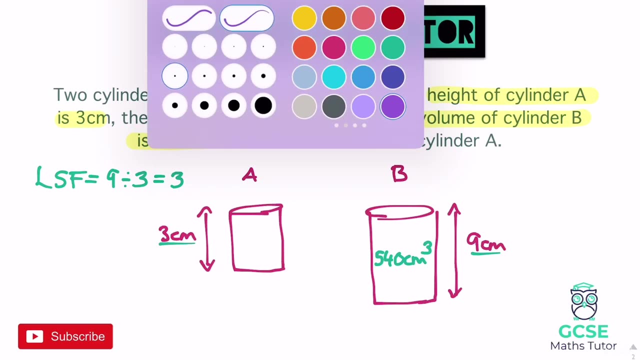 what our scale factor is. Now again, we've got 3 and 9 there being the heights, so I can work out my length scale factor by doing 9 divided by 3.. Again, the bigger one divided by the smaller one And 9 divided by 3 is 3.. Now, again, on this case I'm going to be thinking about, do I want my area? 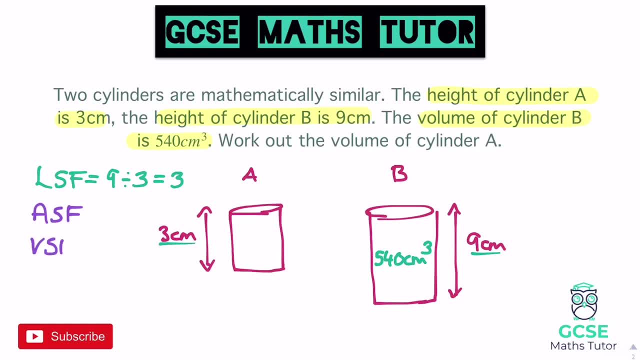 scale factor or do I want my volume scale factor? Now the question here is asking us to work out a volume so I can ignore area, and to get from length to volume. in this case, here we would cube it Again, just thinking about the units. within that it's centimetre cubed. so to get from length to 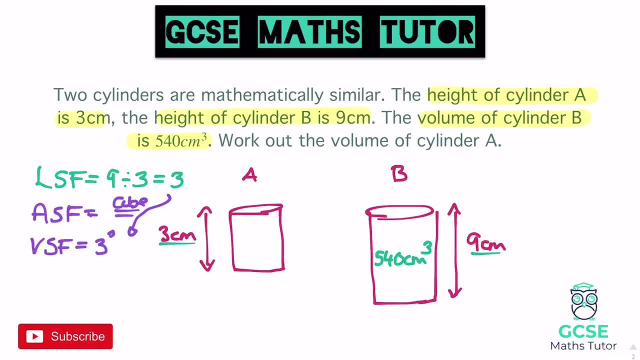 volume. you would cube it. So our volume scale factor is going to be 3 cubed And 3 cubed. we can actually work that out: 3 cubed 3 times 3 times 3 is 27.. So that's the scale. 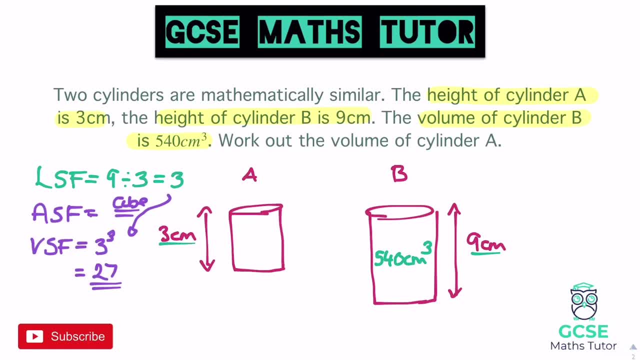 factor we're going to use here when we're looking at volume, Right? so we are working out the volume of A, so I'm going from the big one down to the little one, So I'm not going to multiply this time, because the volume is definitely getting smaller and all I have to do differently here is 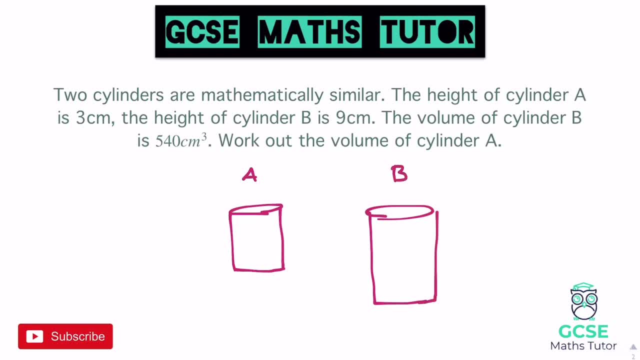 bit bigger there, because i can see that the height of that is nine rather than three. again, this isn't a scale, it's just to give you a little visual idea. so this is three centimeters, is the height of a, and this is nine centimeters for the height of b. now it does also give us another piece of 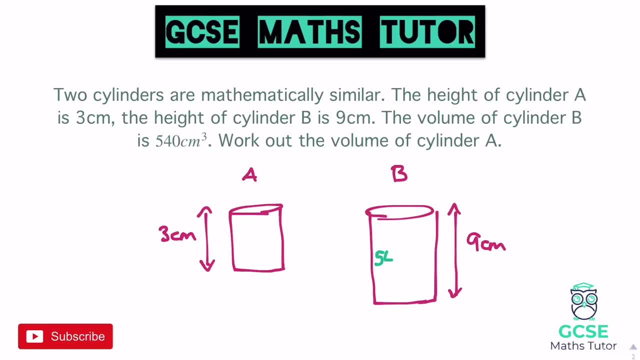 information. so let's write that on. it says 540 centimeter cubed for the volume of b there. okay, just making sure you label that appropriately. okay, it's always a good idea to highlight some of the information. height of a is three, height of b is nine and then: 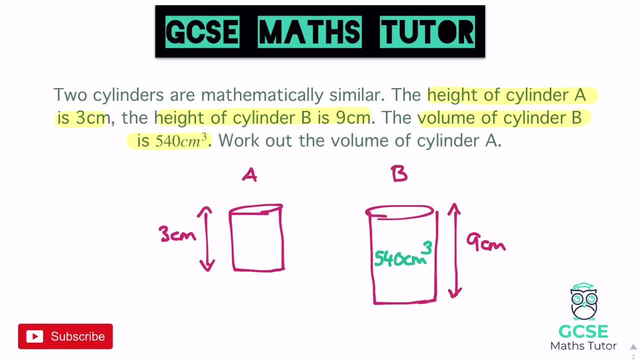 the volume of b is 540 and we're going to work out the volume of a. so, again, we just need to work out what our scale factor is. now, again, we've got three and nine there being the heights, so i can work out my length scale factor by doing nine divided by three. again the bigger one divided by the smaller. 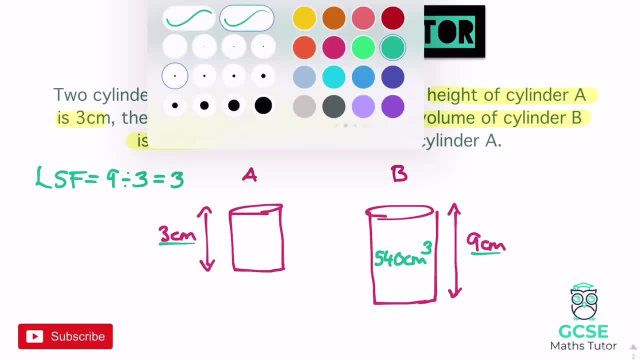 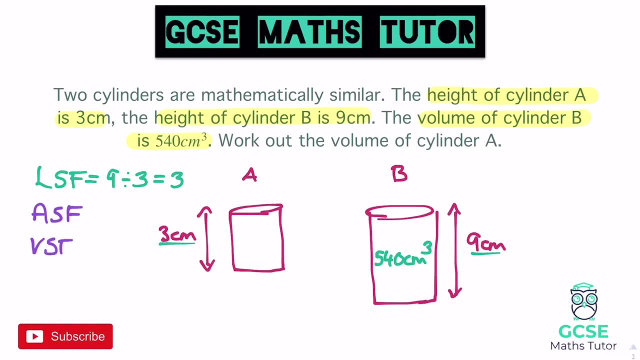 and nine divided by three is three. now, again on this case i'm going to be thinking about: do i want my area scale factor or do i want my volume scale factor? now, the question here is asking us to work out a volume so i can- i can ignore area and to get from length to volume, in this case. here we would. 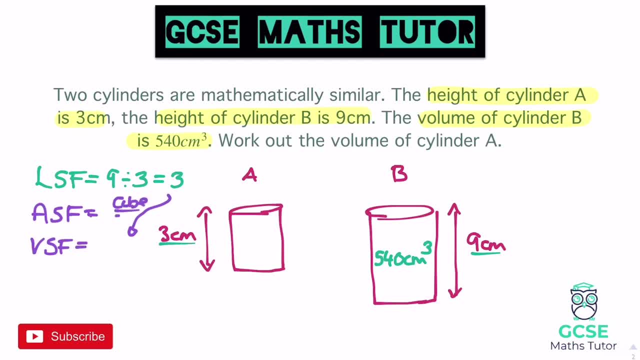 cube it again. just thinking about the units within that, it's centimeter cubed. so to get from length to volume, you would cube it. so our volume scale factor is going to be three cubed, three cubed. we can actually work that out. three cubed three times, three times three is 27, so that's. 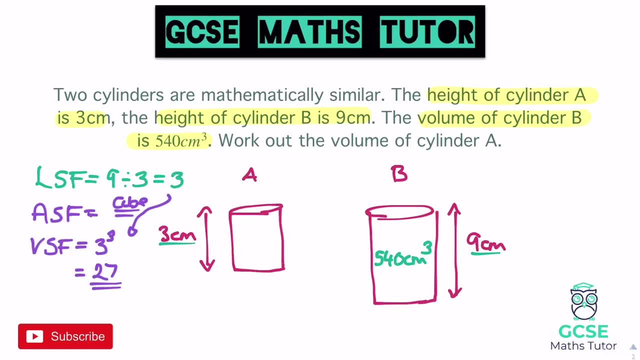 the scale factor we're going to use here when we're looking at volume. right, so we are working out the volume of a, so i'm going from the big one down to the little one, so i'm not going to multiply this time, because the volume is definitely getting smaller and i all i have to do differently here is. 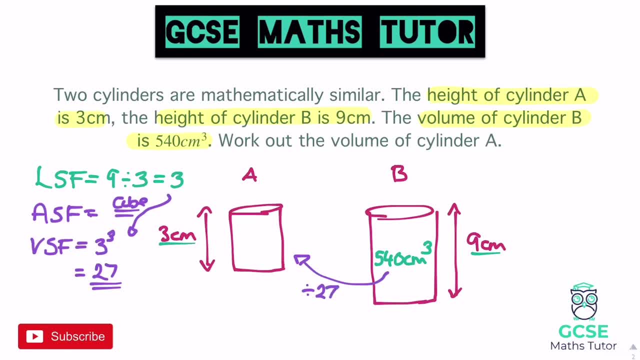 i just divide by the scale factor, so i divide by 27 because thinking about what i said earlier about it being an enlargement, it just means the volume is getting 27 times bigger. so if we're going back down to the smaller one, it has to get 27 times smaller. now, 540 divided by 27 without a calculator isn't too bad. 27 goes into. 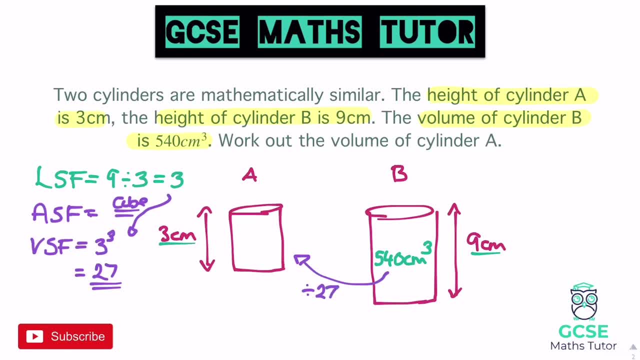 I just divide by the scale factor. So I divide by 27 because, thinking about what I said earlier about it being an enlargement, it just means the volume is getting 27 times bigger. So if we're going back down to the smaller one, we're going to divide by 27.. So that's the scale factor. 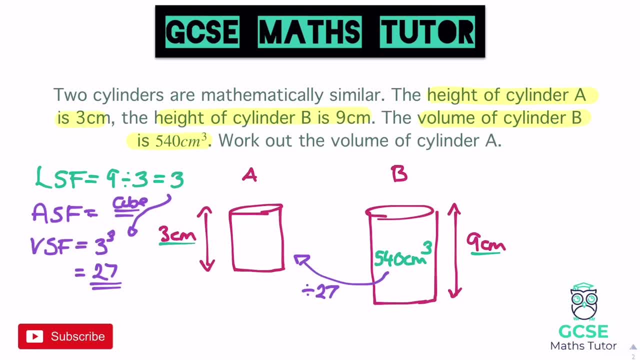 The smaller one has to get 27 times smaller. Now, 540 divided by 27 without a calculator isn't too bad. 27 goes into 54 twice, so it goes into 540 20 times. So my answer for this one is going: 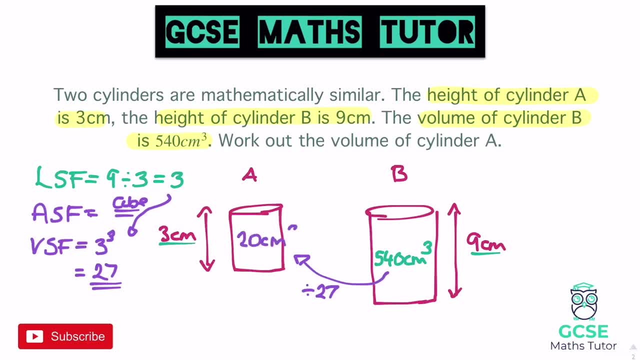 to be 20 centimetres cubed and that's our final answer there. So let's just write that down here this time. So my final answer is 20 centimetre cubed being the volume of A there. Okay, so just a different way of looking at it, obviously, moving from length to volume instead of length to area. 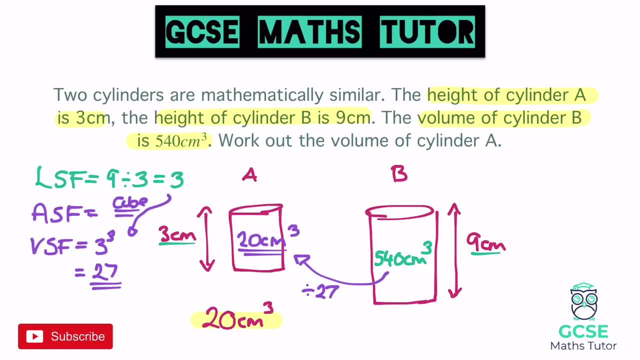 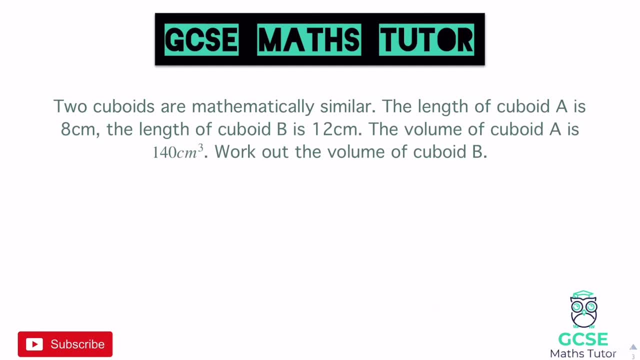 but that is essentially all that we need to do with these types of questions. Let's have a look at one more. Okay, so this says two cuboids are mathematically similar. The length of cuboid A is 8 and the length of cuboid B is 12.. The volume of cuboid A is 140.. Work out the volume of cuboid. 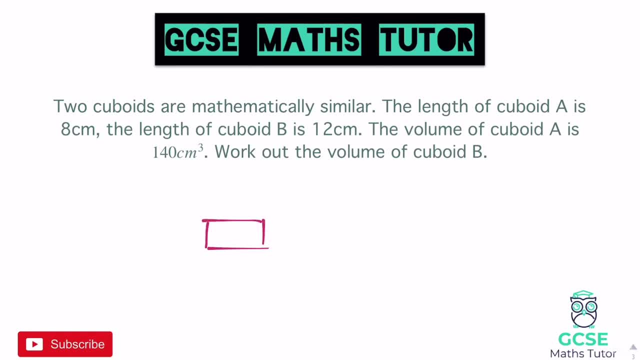 B. So again we can draw a little diagram. Okay, just a nice little simple cuboid. There we go, and let's call that A, and it says the length of that one is 8.. Length could be any of these dimensions, really, but let's just go with that one, and then we've got. 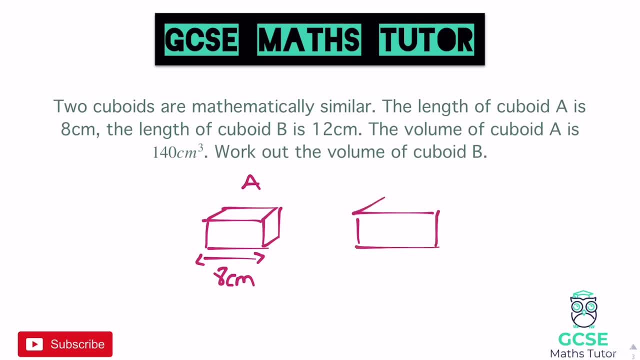 another cuboid which is a bigger one. There we go, nice little easy cuboid to draw and let's call that B and it says the length of that one is 12.. Right, so again we've got these similar lengths there. so we've got 8 and 12.. So to get my length scale factor I just need to do 12, the bigger one. 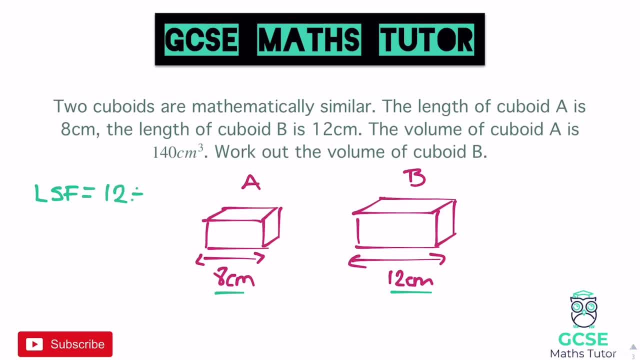 divided by 8.. If we have a calculator, that's nice and easy, Obviously, if you are unsure about this, you can always just write it as a fraction, 12 over 8, and simplify it. So 12 over 8, they both divide by 4, which is 3 over 2, which is 1.5.. So my length scale factor is 1.5.. Now again, we just 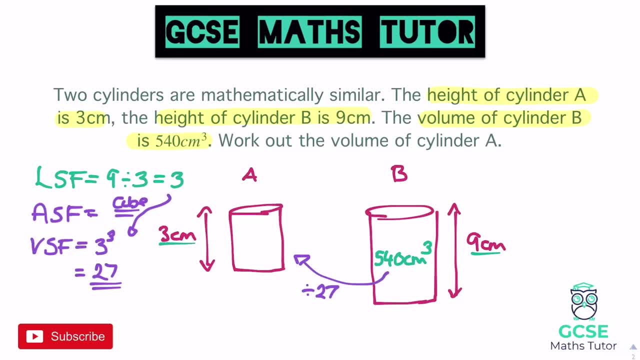 54 twice, so it goes into 540 20 times. so my answer for this one is going to be 20 centimeters cubed and that's our final answer there. so let's just write that down here this time. so my final answer is 20 centimeter cubed being the volume of a there. okay, so just a. 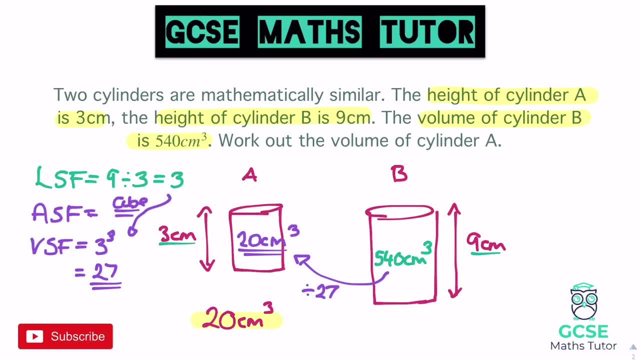 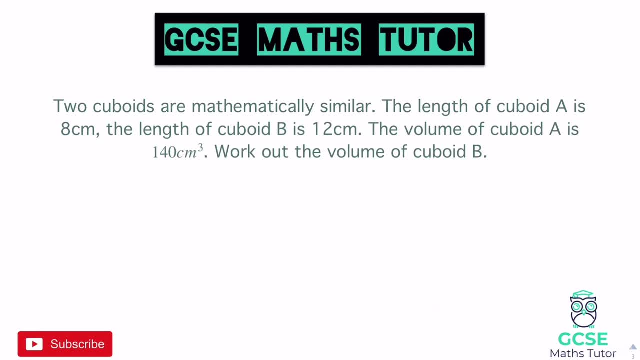 different way of looking at it, obviously, moving from length to volume instead of length to area, but that is essentially all that we need to do with these types of questions. let's have a look at one more. okay, so this says two cuboids are mathematically similar. the length of cuboid a is 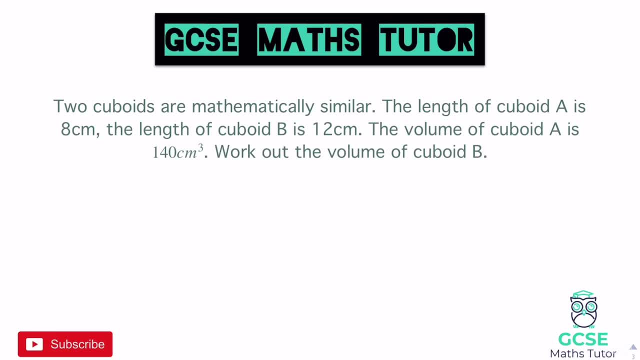 8 and the length of cuboid b is 12. the volume of cuboid a is 140. work out the volume of cuboid b so again we can draw a little diagram. okay, just a nice little simple cuboid. there we go and let's call that a and it says the length of that one is: 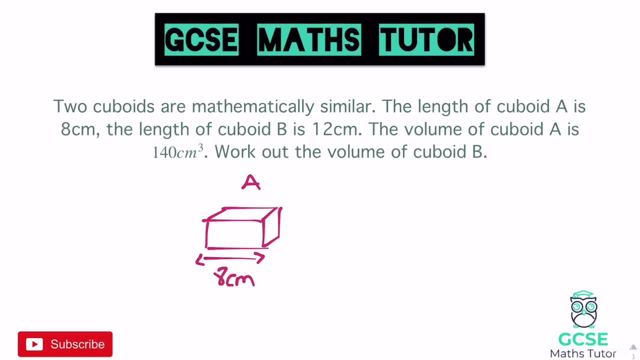 length could be any of these dimensions really, but let's just go with that one. and then we've got another cuboid which is a bigger one. there we go, nice little easy cuboid to draw, and let's call that b, and it says the length of that one is 12, right? so again we've 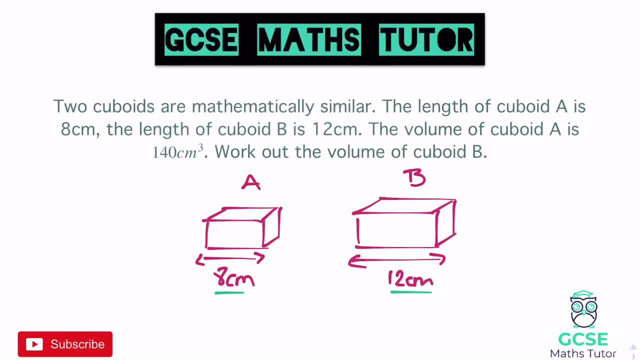 got these similar lengths there, so we've got 8 and 12. so to get my length scale factor i just need to do 12 the bigger one almost wrote 8 there. let's get rid of that: 12 the bigger one divided by 8. if we have a calculator, that's nice and easy, obviously. if you are unsure, 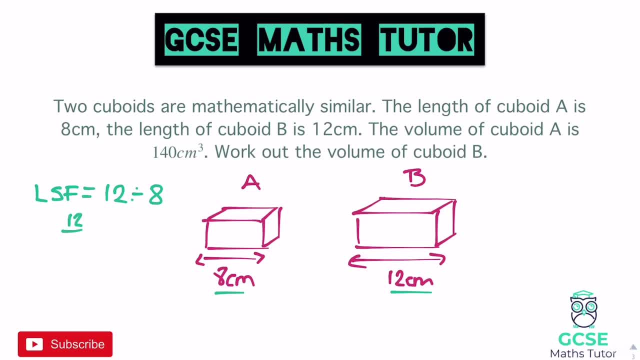 about this. you can always just write it as a fraction, 12 over 8, and simplify it. so 12 over 8. they both divide by 4, which is 3 over 2, which is 1.5. so my length scale factor is 1.5. now again: 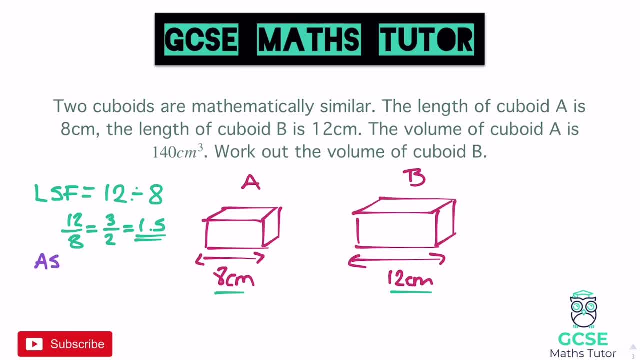 we just need to think: do we need our area scale factor or do we want the volume scale factor? and let's have a quick look at the question. ok, so it says in the question: work out the volume of b. and it says the volume of a is: 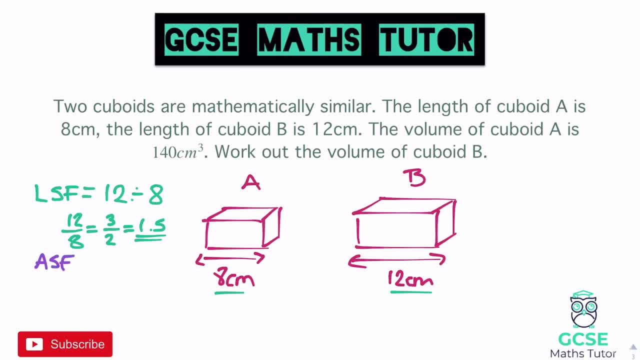 need to think: do we need our area scale factor or do we want the volume scale factor? and let's have a look at the question. Okay, so it says in the question: work out the volume of B and it says the volume of A is 140. So I want to get to volume. So, again getting to volume, we cube it, So 1.5 cubed. 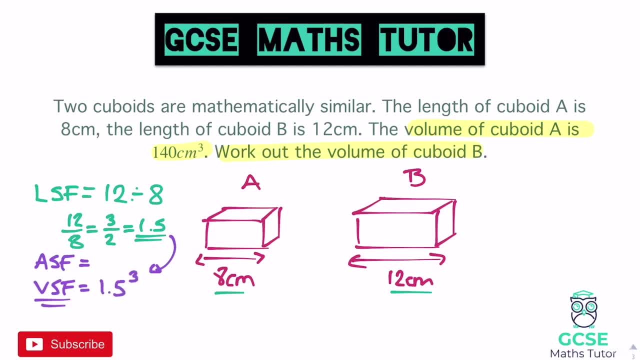 and again, this would be a calculator question. So I'm going to do this on the calculator: 1.5 cubed, which gives me not a very nice number, but it's not too bad: 3.375.. Right, there we go, So let's. 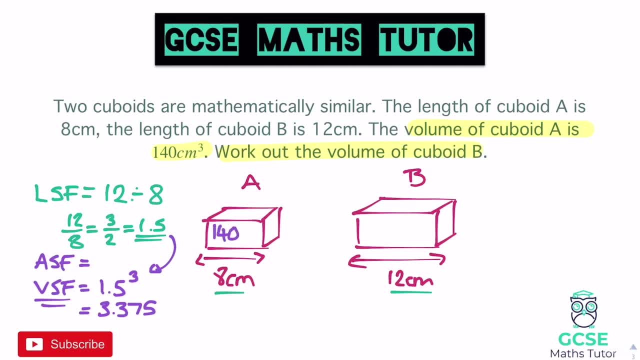 label it on here. the volume of A is 140.. Centimetre cubed and we want to go up to the bigger shape, So we're going to multiply by that scale factor. So multiply by 3.375.. On the calculator, 3.375 multiplied by 140 gives me: 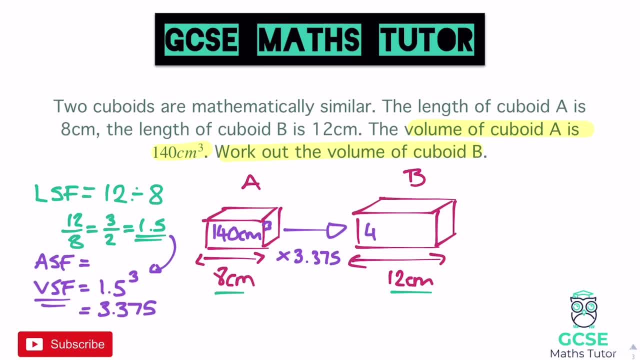 let's write it over here. Let's write it inside the shape: actually: 472.5 centimetres cubed. Okay, we can get the nicest of scale factors there with three decimal places, But we've got a final answer there of 472.5 centimetre cubed, Okay. so all you need to remember for the moment is get your length. 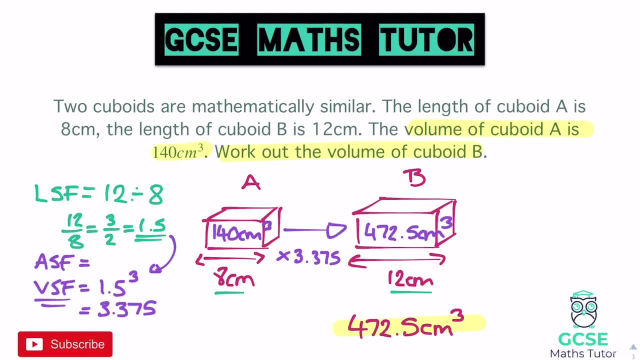 scale factor: big divided by little. Square it if you're dealing with area or surface area and cube it if you are dealing with volume. Then you just need to decide to multiply or divide, depending on whether you're going bigger or smaller, And think logically as well, because obviously the volume of 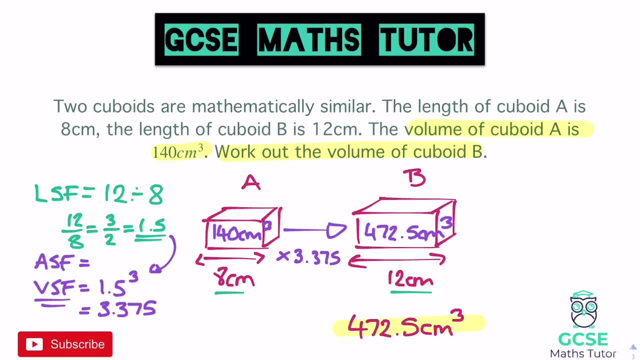 the smaller shape is 140. So if you did accidentally divide by the scale factor, you're going to get a scale factor when you should have multiplied. You should hopefully spot that, because the volume of the larger shape cannot be smaller than the volume of the smaller shape. there I think I said 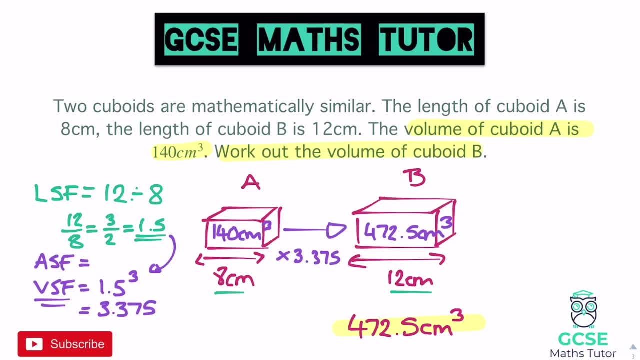 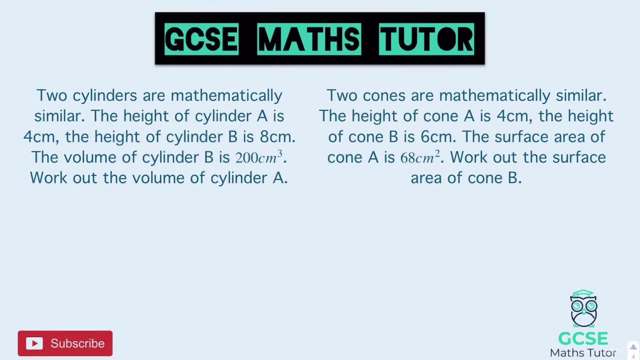 that the right way around? Yeah, the volume of the larger shape cannot be smaller than the volume of the smaller shape. Okay, right, so here's a couple for you to have a go at. Okay, so two questions there. Have a go at both of these. Pause the video there and we'll go over the answers in a sec. 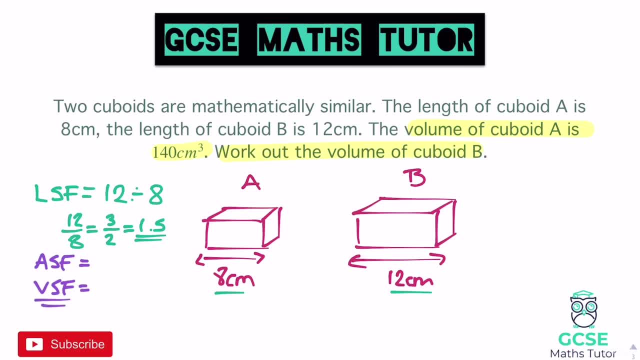 140. so i want to get to volume. so again getting to volume, we cube it. so 1.5 cubed, and again, this would be a calculator question. so i'm going to do this on the calculator: 1.5 cubed, which gives me not a very nice number, but it's not too bad: 3.375, right there we go. so 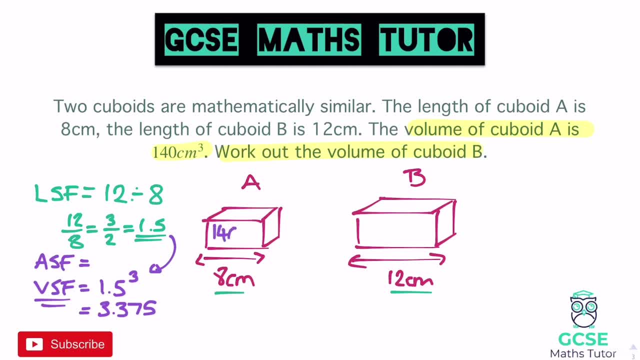 let's label it on here: the volume of a is 140 centimetre cubed and we want to go up to the bigger shape, so we're going to multiply by that scale factor. so multiply by 3.375 on the calculator. 3.375 multiplied by 140 gives: 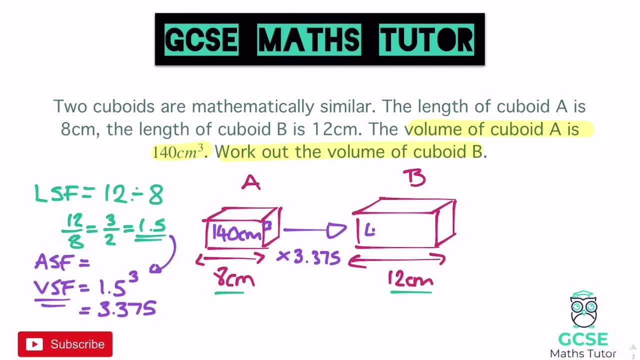 me. let's write it over here, let's write it inside the shape: actually 472.5 centimetres cubed. ok, so there we go. we didn't get the number 3.375, so we're going to go up to the bigger shape. so we're going to multiply by that scale factor, so multiply by 3.375 on the calculator. 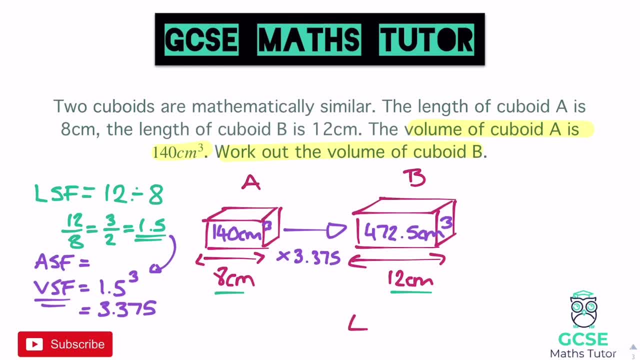 we get the nicest of scale factors there with three decimal places, but we've got our final answer there of 472.5 centimetre cubed. ok, so all you need to remember for the moment is get your length scale factor big divided by little. square it if you're dealing with. 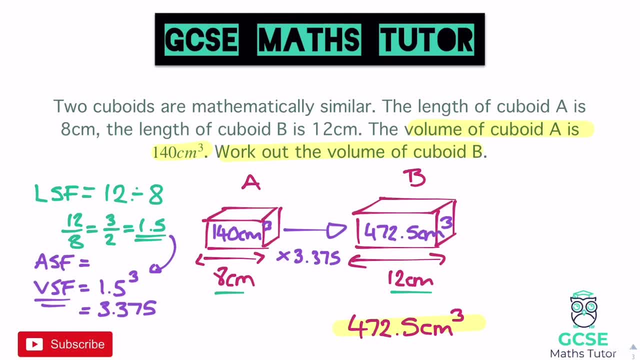 area or surface area and cube it. if you are dealing with volume, then you just need to decide to multiply or divide, depending on whether you're going bigger or smaller, and think logically as well, because obviously the volume of the smaller shape is 140. so if you did accidentally divide by the scale factor, you'd get the nicest of scale factors. 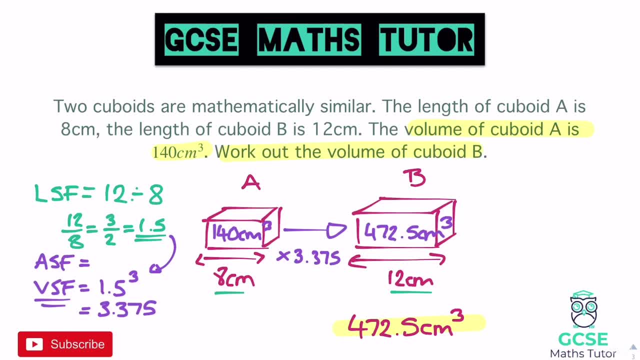 there with three decimal places, but we've got a final answer there of 472.5 centimetre cubed. ok, so if you didn't get your length scale factor, big divided by little, square it. if you're dealing with volume, then you should probably spot that, because the volume of the 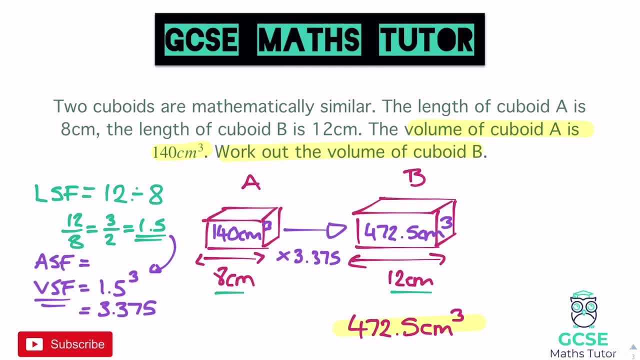 larger shape cannot be smaller than the volume of the smaller shape. there I think I said that the right way around: the volume of the larger shape cannot be smaller than the volume of the smaller shape. ok, right, so here's a couple for you to have a go at. ok, so two questions. 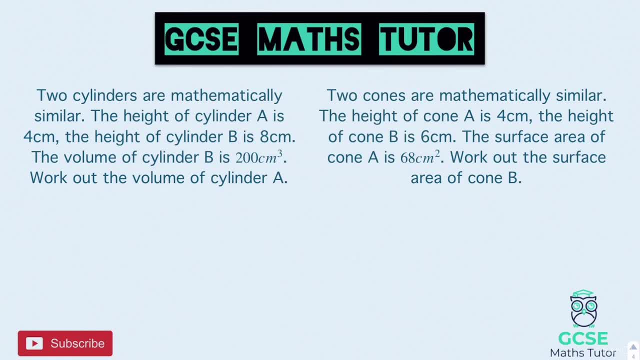 there. have a go at both of these. pause the video there and we'll go over the answers in a sec. okay, so for the first one, I'm not going to draw the pictures for this, but we've got A and B. I'm just going to write A to B and I'm going to go the round. it is because 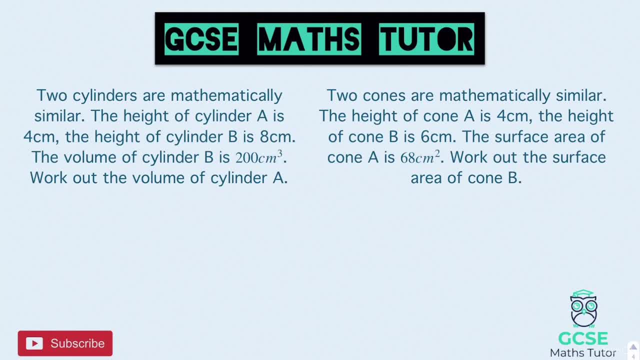 Okay, so for the first one. I'm not going to draw the pictures for this, but we've got A and B. I'm just going to write A to B And we have the volume of B. It says it's 200 centimetre cubed. So to get my scale factor, we've. 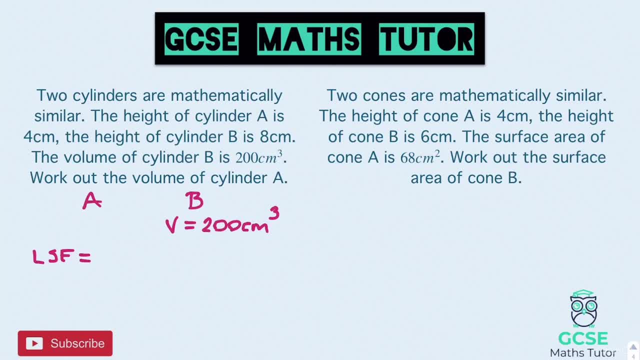 got the height. so the length scale factor is 8, the bigger one divided by 4, which equals 2.. We are looking at volume. Okay, so I'm going to cube that for my volume scale factor, So for my volume scale, and I'm moving from the big shape down to the little shape, A is the smaller one, So I'm going 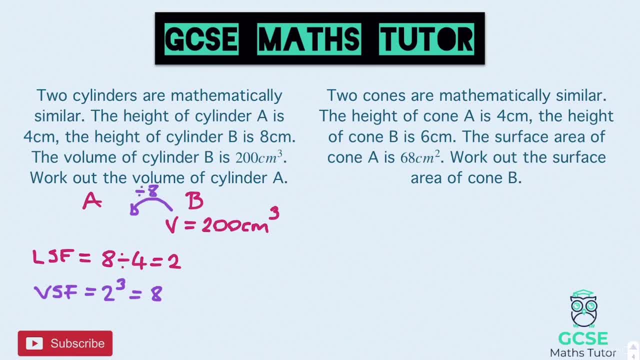 to divide by 8, and 200 divided by 8 is 25 centimetre cubed. There we go. So the answer for my first one is 25 centimetre cubed, and that's that one On to the next one. So we've got shaped A and B. 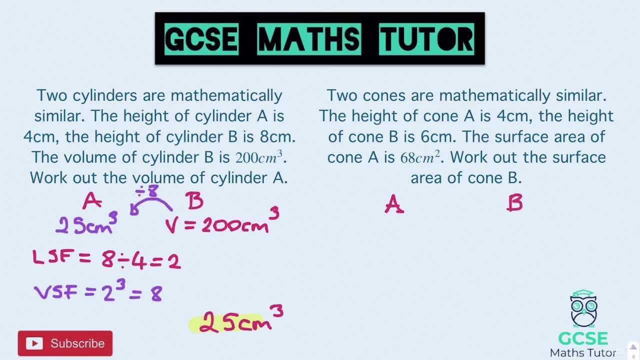 They're cones. So we've got A and we've got B and it says the surface area of A is 68 centimetre squared. I'm just going to put A next to that, so I don't forget that I'm looking at the area there. 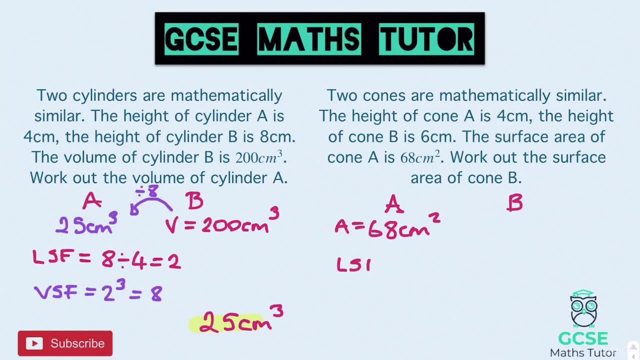 Right, so let's find our length scale factor. So my length scale factor this time The bigger shape is 6.. The smaller shape is 4.. 6 divided by 4, which again is 1.5.. Now this time we're dealing with area. 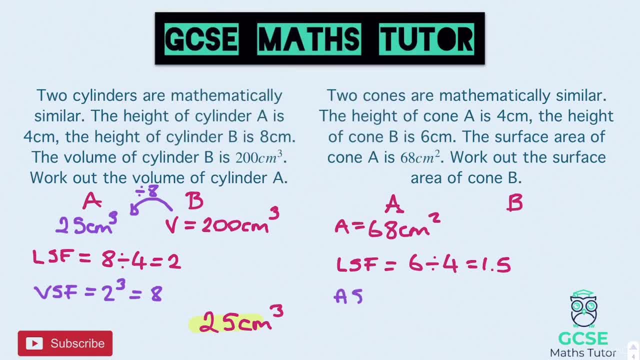 So I don't need to cube it, I need to square it. So to get my area scale factor this time, I'm going to do 1.5 squared And we're working that out. 1.5 times 1.5 is 2.25.. So my scale factor, this time for area, is 2.25.. 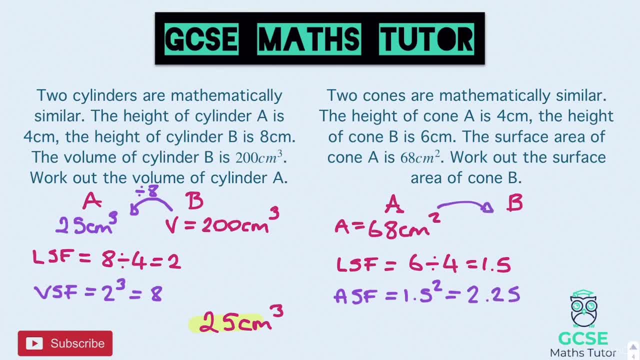 Now, this time we're moving from the smaller to the bigger shape, So we're going to multiply by that scale factor. So times 2.25 and 2.25 multiplied by 68 gives me 153 centimetres squared, So that's 2.25.. 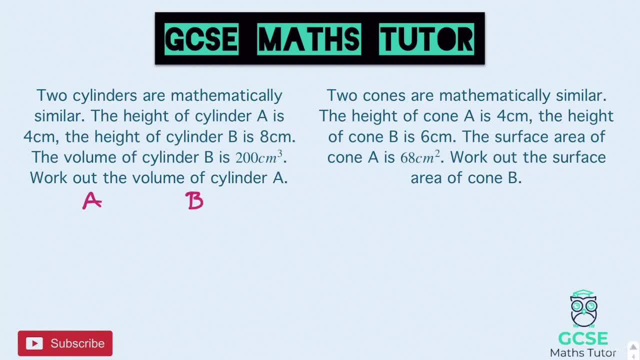 A is a little bit to the left and B is a little bit to the right. so that's what we're going and we have the volume of B. it says it's 200 centimetre cubed. So to get my scale factor, we've got the height. so the length scale factor is 8, the bigger one divided by 4, which equals 2.. 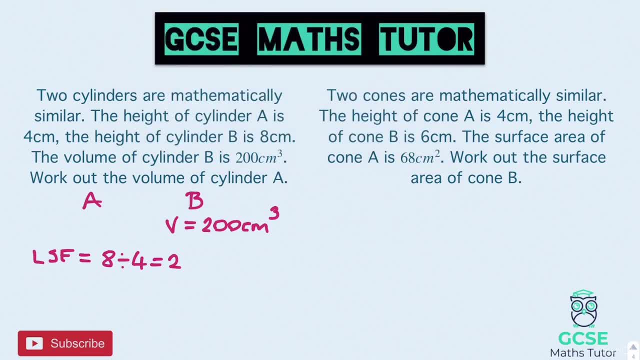 We are looking at volume, so I'm going to cube that for my volume scale factor. So for my volume scale factor I need to do 2 cubed, which is 8.. And I'm moving from the big shape down to the little shape. A is the smaller one, so I'm going to divide by 8.. 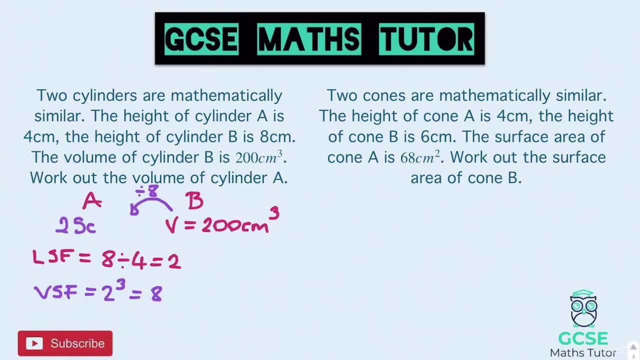 And 200 divided by 8 is 25 centimetre cubed. There we go. so the answer for my first one is 25 centimetre cubed, And that's that one On to the next one. So we've got shaped A and B. 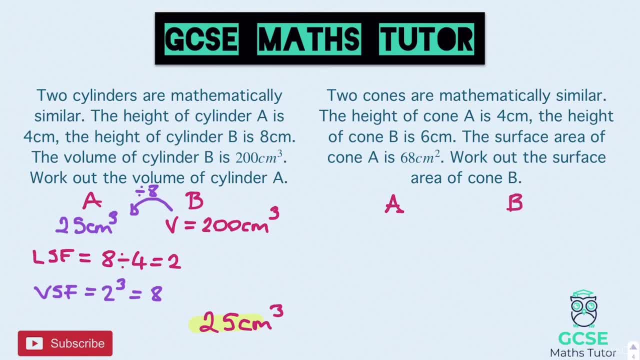 They're 2.. We've got cones, so we've got A and we've got B, And it says the surface area of A is 68 centimetre squared. I'm just going to put A next to that, so I don't forget that I'm looking at the area there. 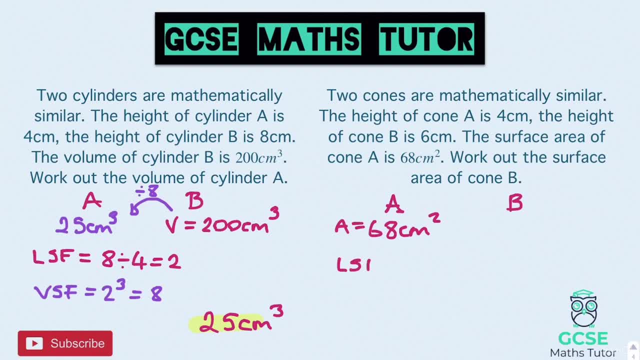 Right, so let's find our length scale factor. So my length scale factor: this time the bigger shape is 6, the smaller shape is 4, 6 divided by 4, which again is 1.5.. Now this time we're dealing with area, so I don't need to cube. 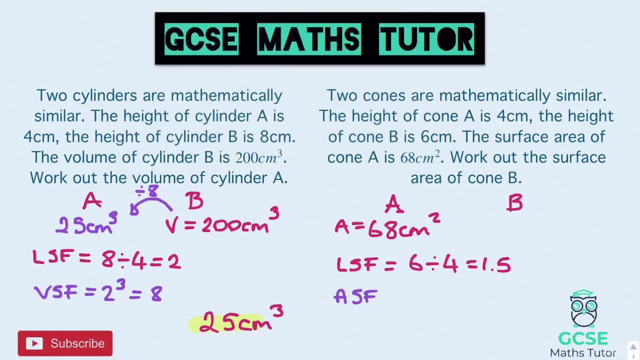 I need to square it. so to get my area scale factor, this time I'm going to do 1.5 squared And we're working that out. 1.5 times 1.5 is 2.25.. So my scale factor, this time for area, is 2.25.. 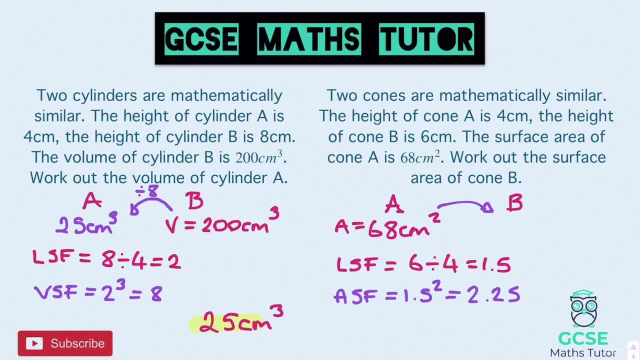 Now, this time we're moving from the smaller to the bigger shape, So we're going to multiply by that scale factor, so times 2.25.. And 2.25 multiplied by 68 gives me 155.. 153 centimetres squared. 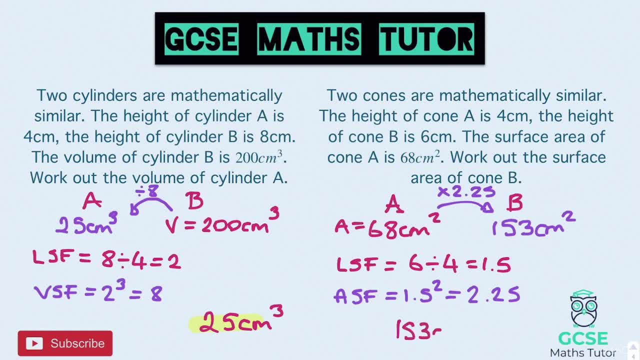 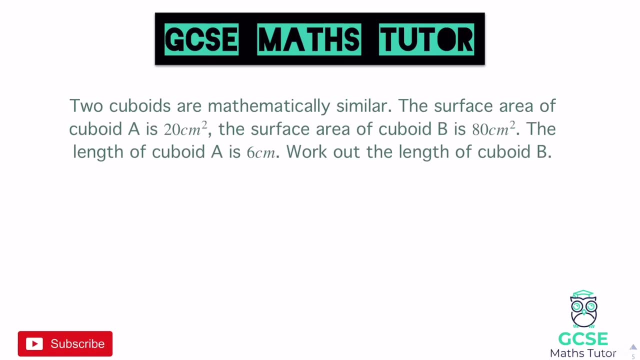 There we go. so 153 centimetres squared, because we're looking at area, And that is the surface area of that shape, shape B. Right, there we go. let's have a look at some slightly different scenarios, then. Okay, so in this question it says two cuboids are mathematically similar. 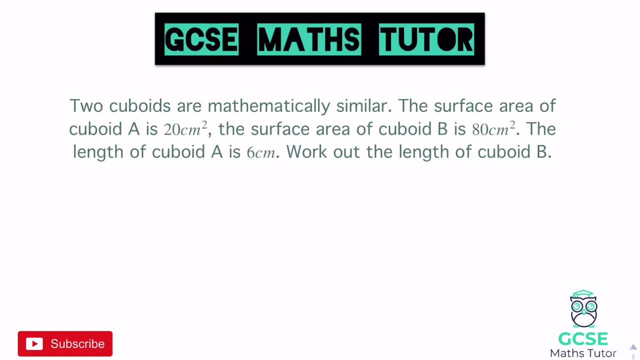 It says the surface area, so straight away- it's not giving us a length here, straight away- It says the surface area of cuboids. So the cuboid A is 20 and the surface area of cuboid B is 80. And then it says the length of cuboid A is 6, work out the length of cuboid B. 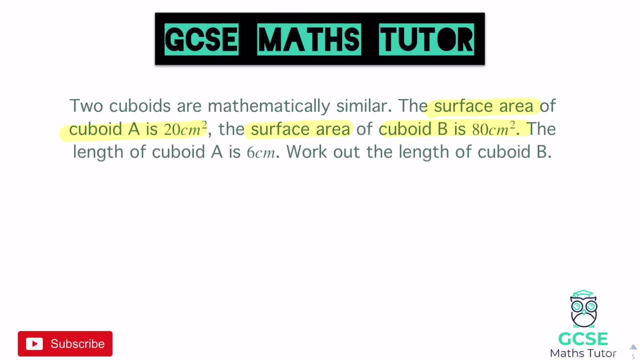 Okay. so this time it's given us the surface area and it's wanting us to work out our length. Now let's just have a think about this. So we've got a cuboid again And let's say that's A and it says the surface area is 20.. 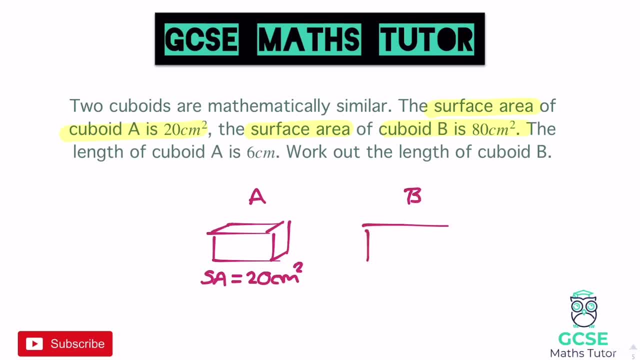 Okay, And then we've got a cuboid B which, looking at it, it says 80, so that's a bigger cuboid, so I'll draw that a little bit bigger. There we go, And it says the surface area for this one is 80.. 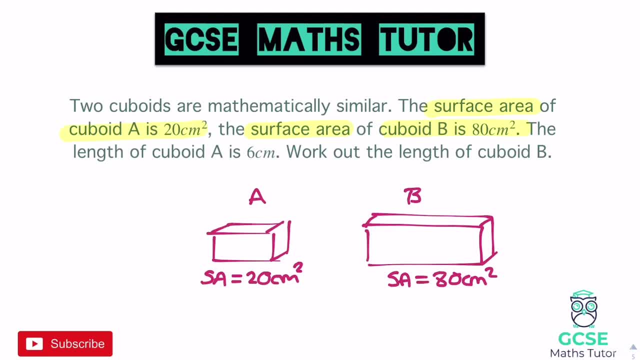 Right. so it's wanting me to work out the length. Now I'm going to label the length slightly differently here, just because I've already written below. Okay, so I'm going to say that the length this times, this one, let's go with that. 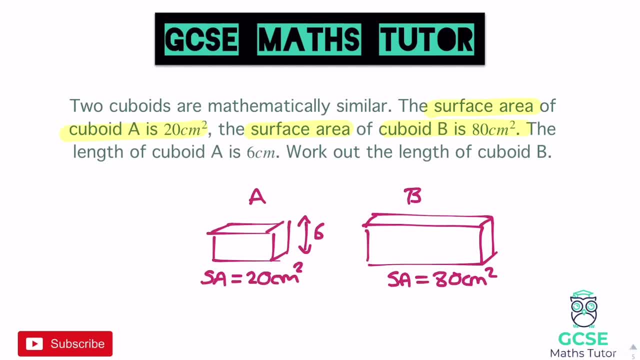 It doesn't actually matter here where I label it. So the length is 6 for A And for B. we don't know. Okay, so we don't know what the length of B is Right. so if we actually work out a scale factor here, the only scale factor we can actually work out is between these two areas. 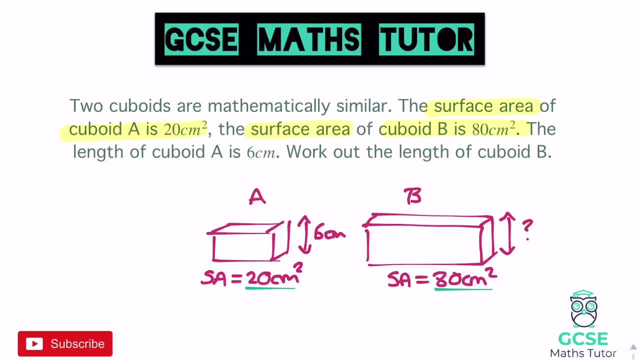 because they're linked up, we've got the surface area of both. So if I work them out this time, doing big divided by little, it won't give me the length scale factor, it will straight away give me the area scale factor. 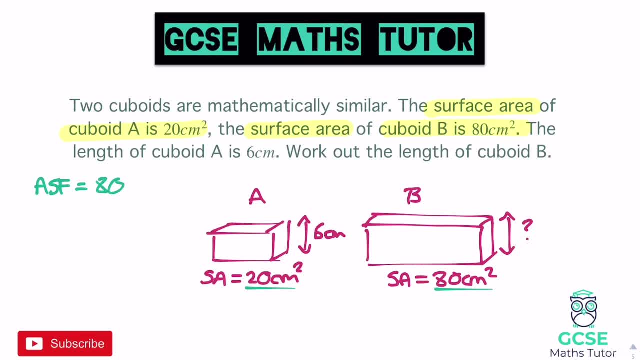 So the area scale factor will be 80 divided by the 20, which comes out as 4.. Now, if I want to get from area to length- which is what we want, because we want to work out what the other length is instead of the 6,- 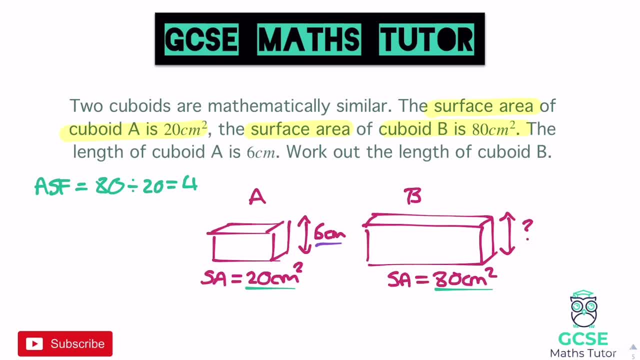 if I want to get from area to length, instead of squaring or cubing, I'm going to have to do the reverse of that, And the opposite of squaring, which is how you get from length to area, is square rooting. 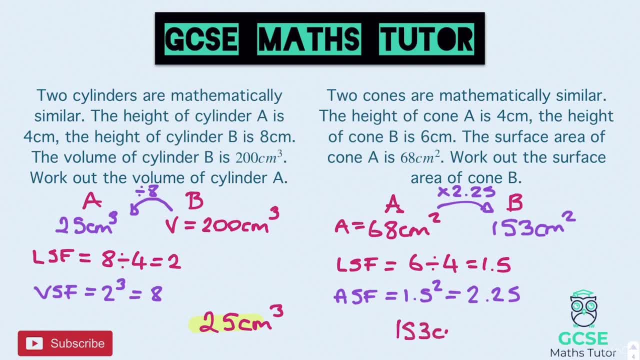 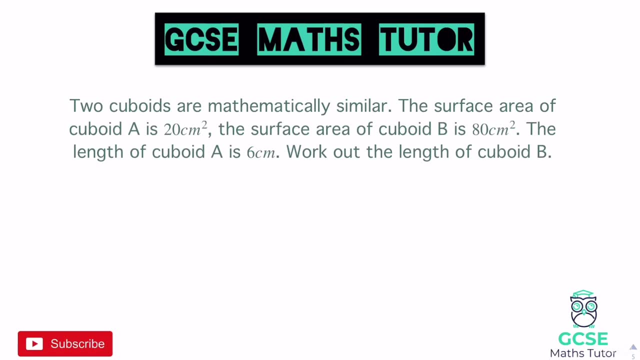 There we go. So 153 centimetres squared, because we're looking at area, And that is the surface area of that shape, shape B. Right, there we go. Let's have a look at some slightly different scenarios then. OK, so in this question it says two cuboids are mathematically similar. 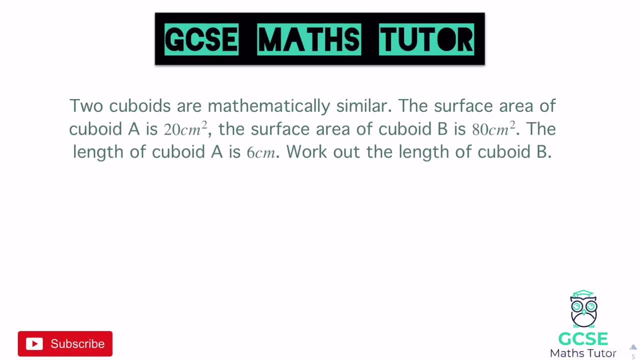 It says the surface area, So straight away it's not given us a length here. straight away It says the surface area of cuboid A is 20 and the surface area of cuboid B is 80. And then it says the length of cuboid B is 80. 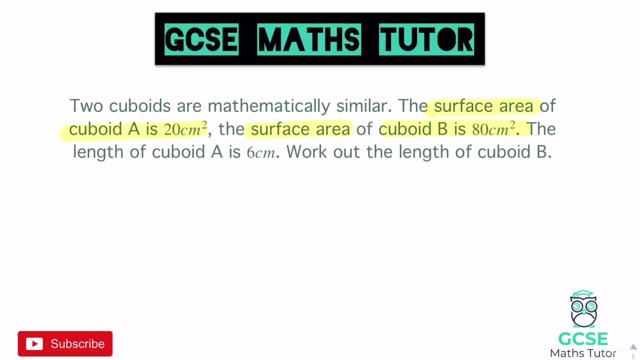 And then it says cuboid A is 6. Work out the length of cuboid B. OK, so this time it's given us the surface area and it's wanting us to work out our length. Now let's just have a think about this. So we've got a cuboid again. 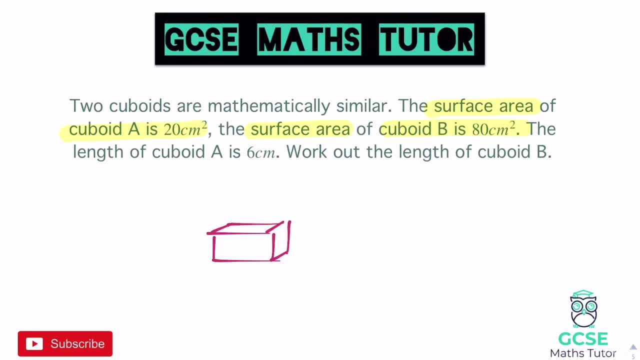 And let's say that's A And it says the surface area is 20.. OK, Then we've got cuboid B which, looking at it, it says 80. so that's a bigger cuboid. so I'll draw that a little bit bigger. 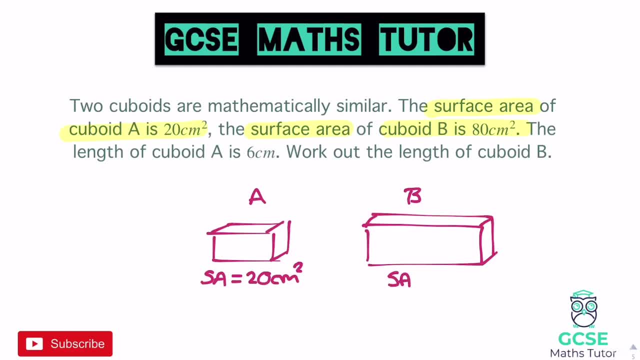 There we go, And it says the surface area for this one is 80.. Right, so it's wanting me to work out the length. Now I'm going to label the length slightly differently here, just because I've already written below. OK, so I'm going to say that the length this times this one. Let's go with that. 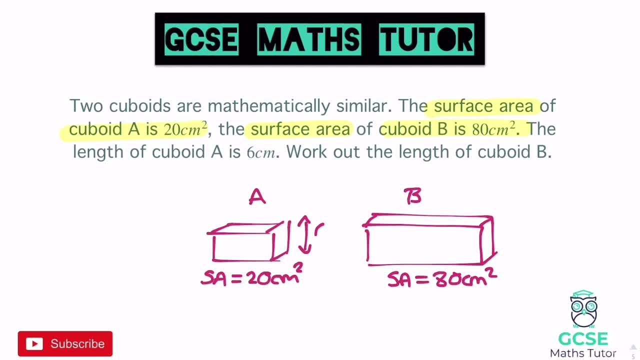 It doesn't actually matter here where I label it. So the length is 6 for A and for B. we don't know. OK, so we don't know what the length of B is Right. so if we actually work out the length of A, 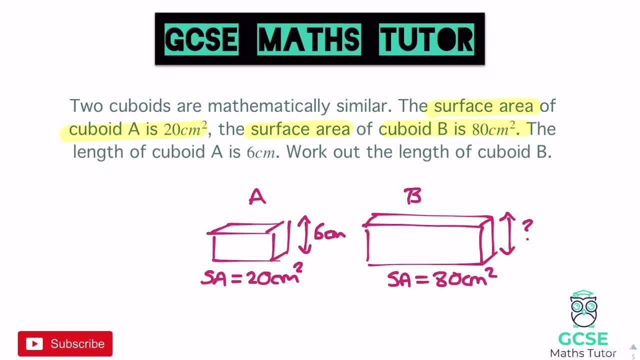 Right. so if we actually work out the length of B, I'm actually going to work out a scale factor here. The only scale factor we can actually work out is between these two areas, because they're linked up. We've got the surface area of both. 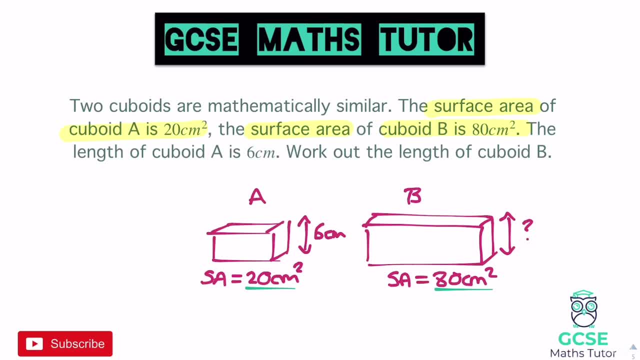 So if I work them out this time doing big divided by little, It won't give me the length scale factor, it'll straight away give me the area scale factor. So the area scale factor will be 80 divided by the 20, which comes out as 4.. 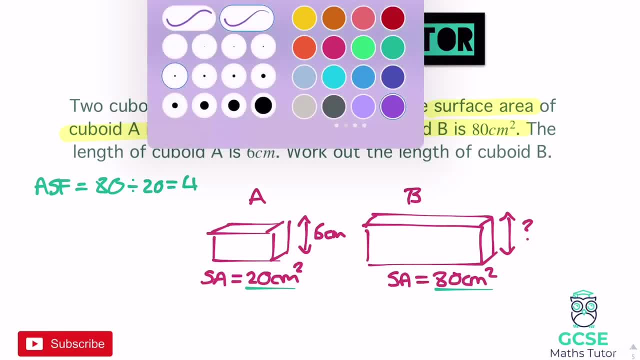 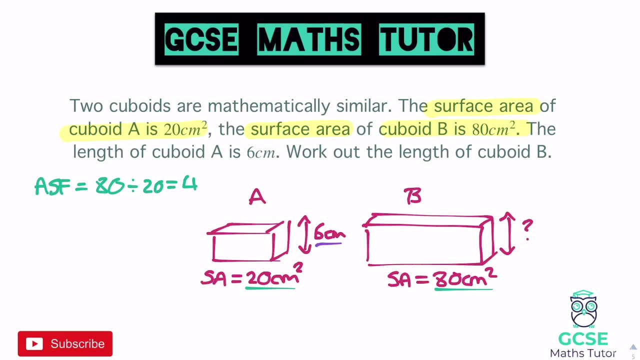 Now, if I want to get from area to length, which is what we want because, because we want to work out what the other length is instead of the 6. If I want to get from area to length instead of squaring or cubing. 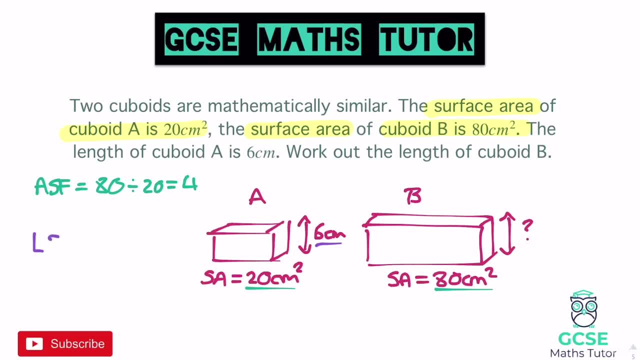 I'm going to have to do the reverse of that, And the opposite of squaring, which is how you get from length to area, is square rooting. So to get from 4 back to whatever that length scale factor was, I'm going to have to do a square root. 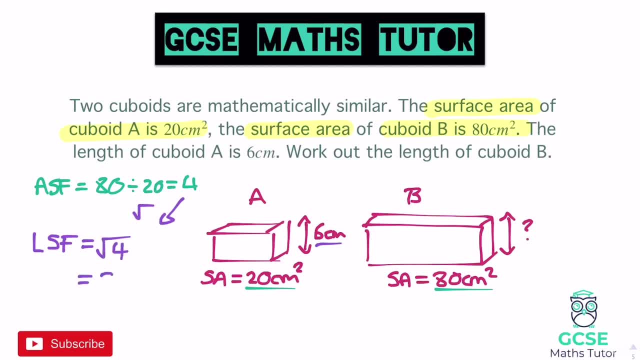 So I'll work out the square root of 4,, which is 2, and therefore my length scale factor must have been 2.. So that's the only length scale factor that will give me an area scale factor of 4.. So to get from the small shape back up to the big shape, 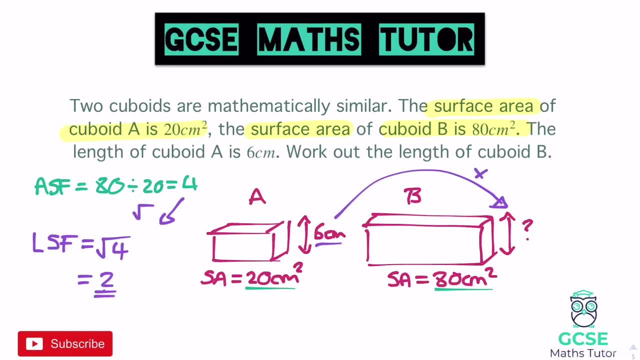 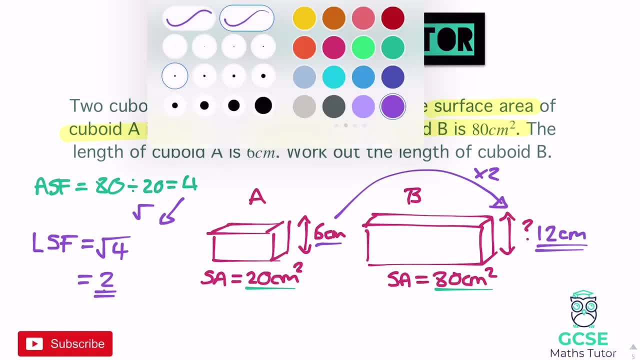 I'm going to multiply by that scale factor, which in this time is 2, because we're looking at length now, and 6 times 2 is 12 centimetres. So my final answer for this question is 12 centimetres. 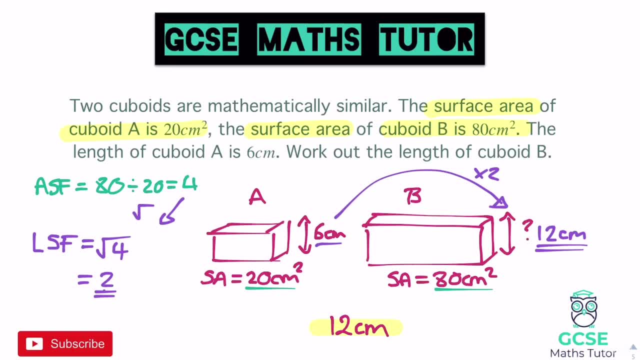 OK, so a slightly different scenario there. If you're given the areas, you can get the area scale factor and you have to go back to length by square rooting. Similarly, which we're going to have a look at now, if I had the volumes and I've got the volume scale factor, 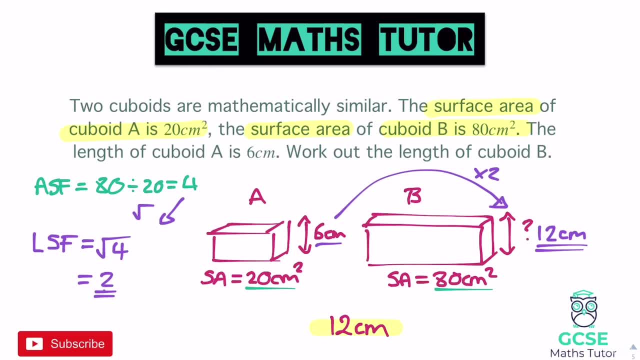 the opposite of cubing, which is how we get from length to volume, is cube rooting. So I'd have to do the opposite again and I would have to cube root the scale factor. So let's have a look at one of those scenarios before you have a go. 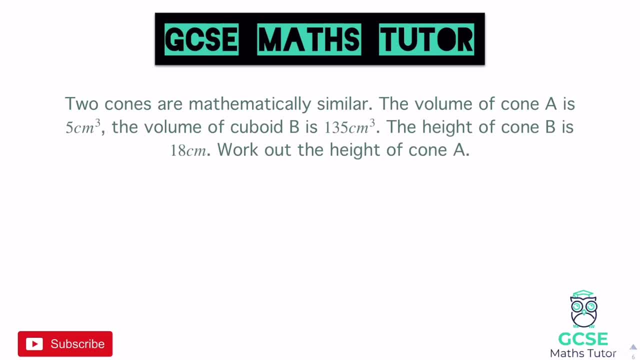 OK. so this question says two cones are mathematically similar and then, like I said, it says the volume of A is 5 centimetre cubed and the volume of B is 135 centimetre cubed, And then it says the height of cone B is 18, work out the height of A. 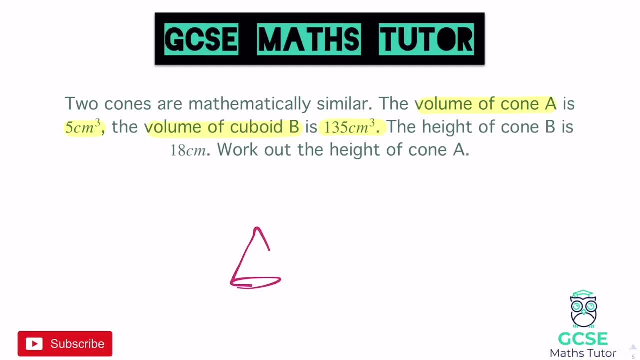 So again, let's draw. Let's draw this, A being our smaller shape here, which it says has a volume of 5.. I'll just put that next to it. this time, Volume equals 5 centimetre cubed. And then we've got cone B, which is bigger. 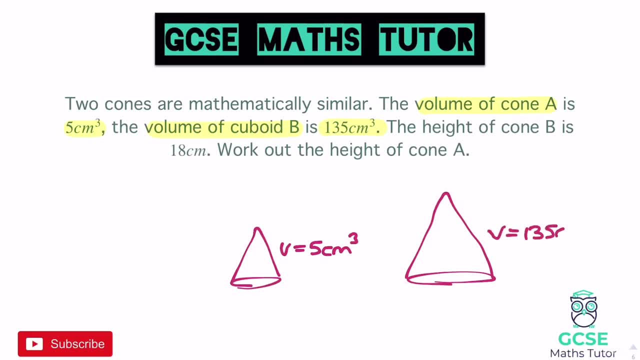 and it says the volume of that is 135 centimetre cubed. There we go. So we've got A and B and it gives us the height of one of them. Which one was it? The height of cone B is 18.. 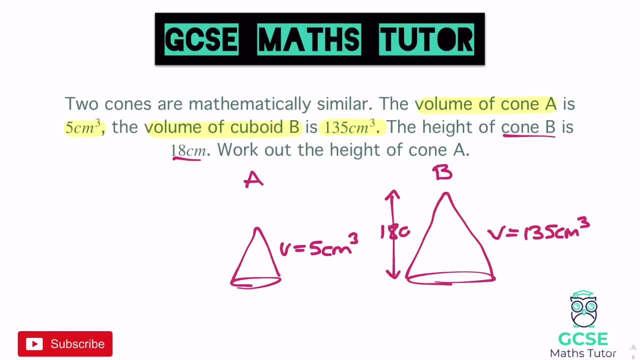 OK, so it's given us the height here. So it's given us the height of cone B, which is 18 centimetres, Right, so let's have a think about what we can do here then. Now, what we have been given is the two volumes. 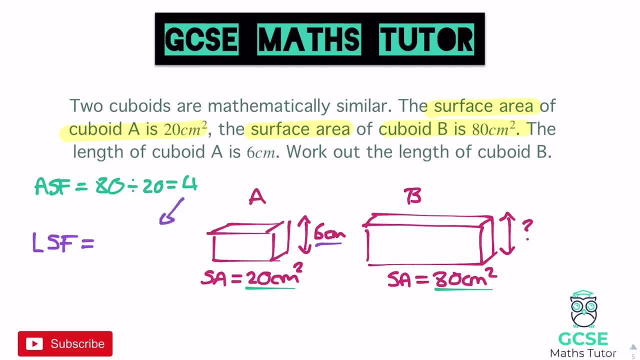 So to get from 4 back to whatever that length scale factor was, I'm going to have to do a square root. So I'll work out the square root of 4.. Which is 2, and therefore my length scale factor must have been 2.. 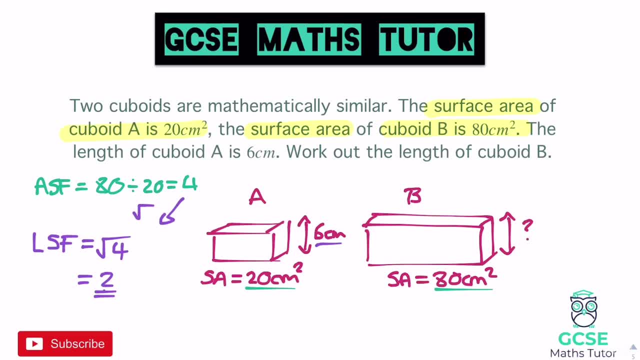 That's the only length scale factor that will give me an area scale factor of 4.. So to get from the small shape back up to the big shape, I'm going to multiply by that scale factor, which in this time is 2, because we're looking at length now, and 6 times 2 is 12 centimetres. 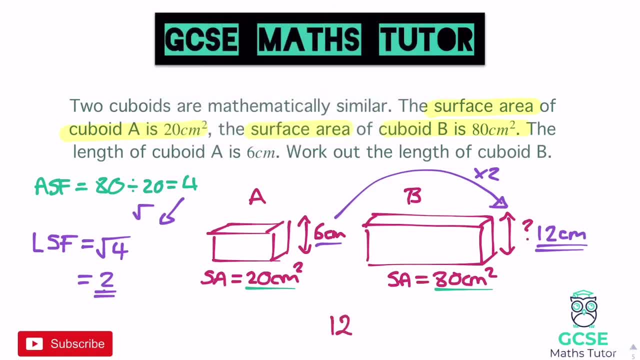 So my final answer for this question is 12 centimetres. OK, so a slightly different scenario there. If you're given the areas, you can get the area scale factor and you have to go back to length by square rooting Similarly, which we're going to have a look at now. 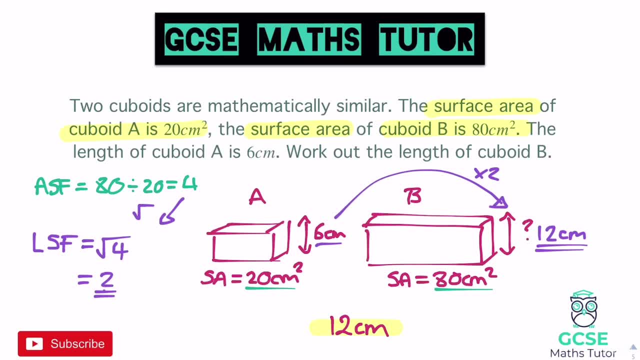 if I had the volumes and I got the volume scale factor. the opposite of cubing, which is how we get from length to volume, is cube rooting. So I'd have to do the opposite again and I would have to cube root the scale factor. 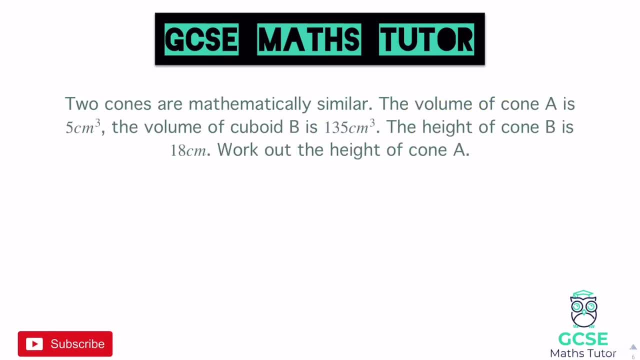 So let's have a look at one of those scenarios before you have a go. OK, so this question says two cones are mathematically similar And then, like I said, it says the volume of A is 5 centimetre cubed and the volume of B is 135 centimetre cubed. 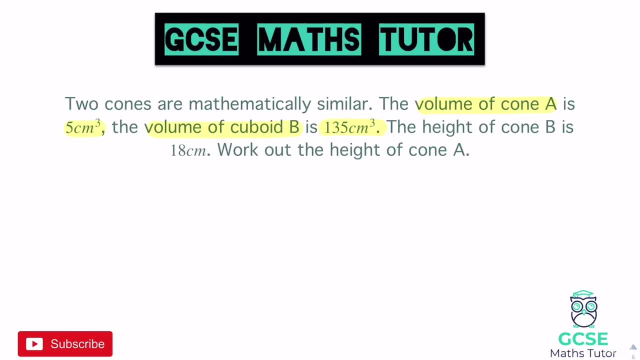 And then it says the height of cone B is 18, work out the height of A. So again, let's draw this, A being our smaller shape here, which it says has a volume of 5.. I'll just put that next to it. this time, volume equals 5 centimetre cubed. 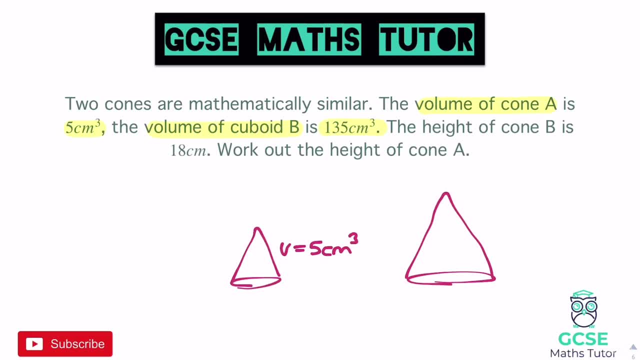 And then we've got cone B, which is bigger, And it says the volume of that is 135 centimetre cubed. There we go, So we've got A and B and it gives us the height of one of them. Which one was it? The height of cone B is 18.. 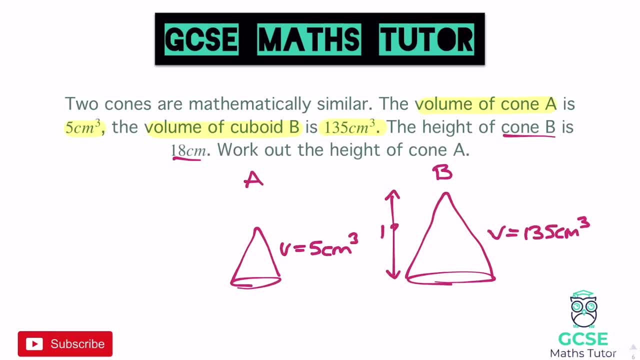 OK, so it's given us the height here, 18 centimetres, Right. so let's have a think about what we can do here then. Now, what we have been given is the two volumes We've got 5 and 135.. 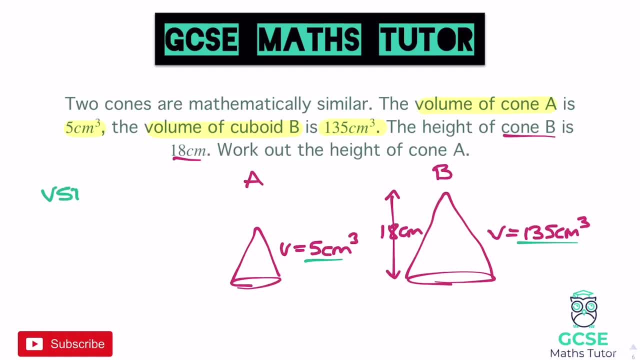 So straight away I can get the volume scale factor. So the volume scale factor is going to be 135 divided by 5.. Obviously, if you don't have a calculator, you just need to do a bit of bus stop for that or something to work that out. 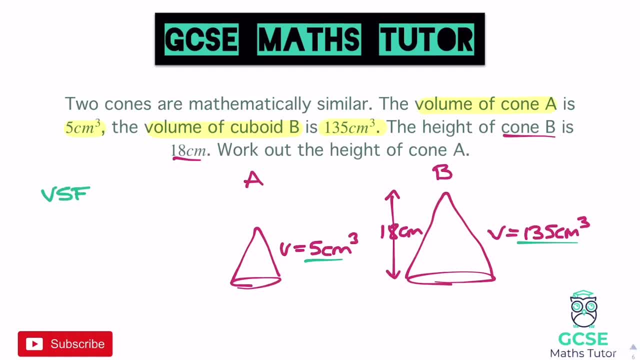 We've got 5 and 135. So straight away I can get the volume scale factor. So the volume scale factor is going to be 135 divided by 5.. Obviously, if you don't have a calculator, you just need to do a bit of bus stop for that or something to work that out. 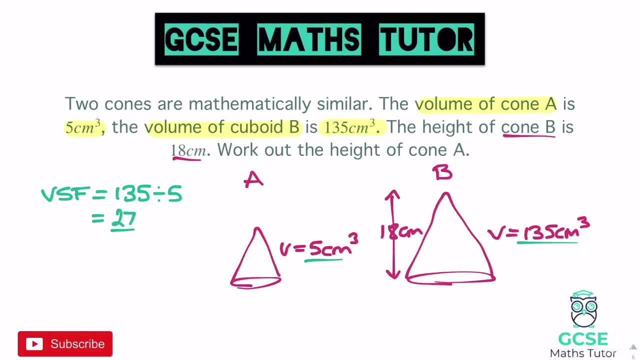 But the volume scale factor comes out as 27.. So we need a length scale factor. So to get back to length, we need to do the opposite of what we do if we were going from length to volume, which is cubing. So we're going to do the opposite of that. 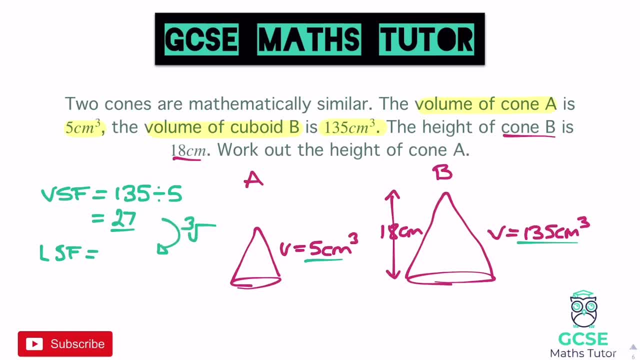 We are going to cube root. So the cube root of 27,. 27 is a cube number. The cube root of 27 is 3.. So my volume scale, my length scale factor, is 3.. Now, this time we're moving from the bigger. 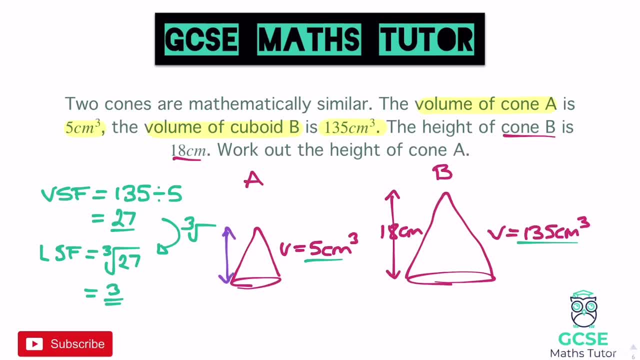 shape, down to the little height here, the little shape. So we're going to have to divide by that scale factor. So we're going to divide by the length scale factor, which is 3.. And if you do 18 divided by 3, you get 6 centimetres: 18 divided by 3.. 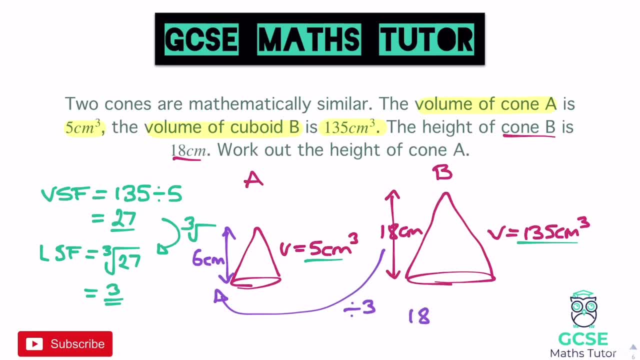 Again. you can write that, working out down: obviously, 18 divided by 3 equals 6.. So my final answer for this question is 6 centimetres. As it's a length, this time, there we go: 6 centimetres. 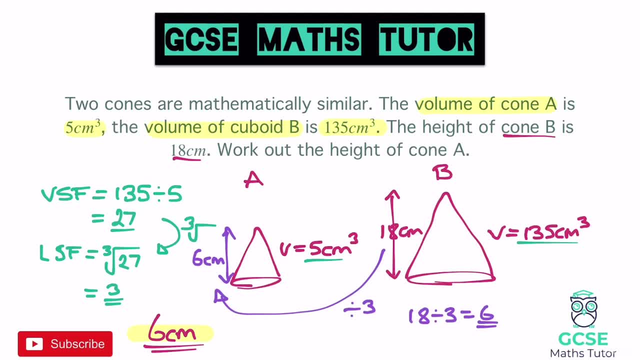 Right, here's a couple for you to have a go at. then Just obviously think about which scale factor you're finding- the area or the volume- And then just remember how to get back to length from that. So square root the area to get back to length, or cube root the volume to get back to length. 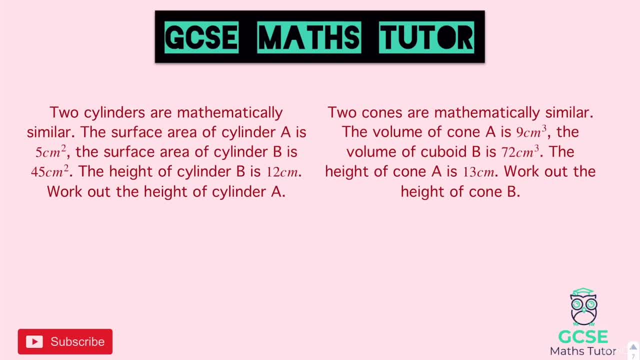 OK, here they are. OK, so two questions there. Pause the video and we'll go over the answers in a sec, Right, OK? so for this first question, we are given the surface areas. so I can find the area scale factor by doing the bigger area, which is 45, and dividing it by the smaller area. 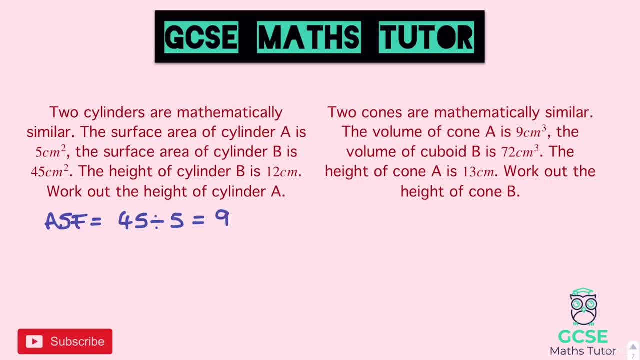 which is 5, and 45 divided by 5 is 9.. You will tend to notice not all the time, but you will tend to notice that a lot of the time square numbers or cube numbers come up in these, so knowing them is obviously very helpful. 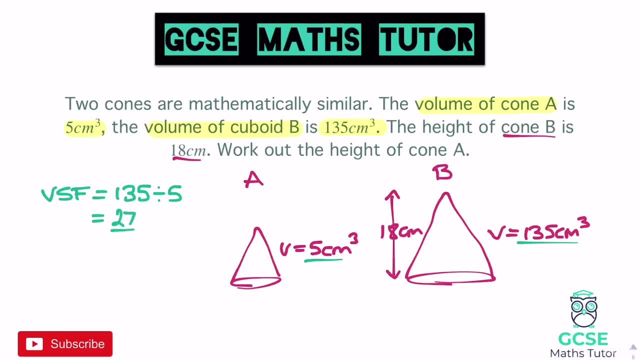 But the volume scale factor comes out as 27.. Now again, we're trying to work out a height, So we need a length scale factor. So to get back to length, we need to do the opposite of what we do if we were going from length to volume, which is cubing. 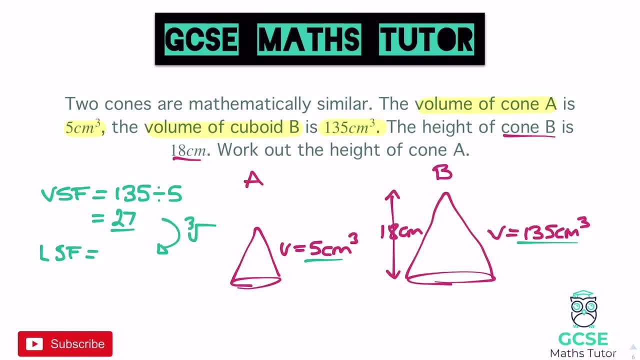 So we're going to do the opposite of that. We are going to cube root. So the cube root of 27,. 27 is a cube number. The cube root of 27 is 3.. So my length scale factor is 3.. 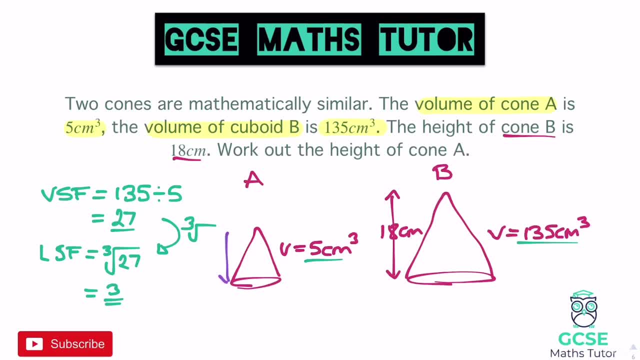 Now, this time we're moving from the bigger shape down to the little height here, The little shape. So we're going to have to divide by that scale factor. So we're going to divide by the length scale factor, which is 3.. 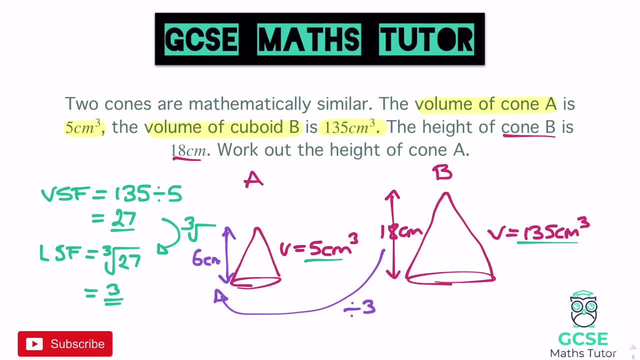 And if you do 18 divided by 3, you get 6 centimetres, 18 divided by 3.. Again, you can write that, working out down, obviously, 18 divided by 3 equals 6.. So my final answer for this question is 6 centimetres. 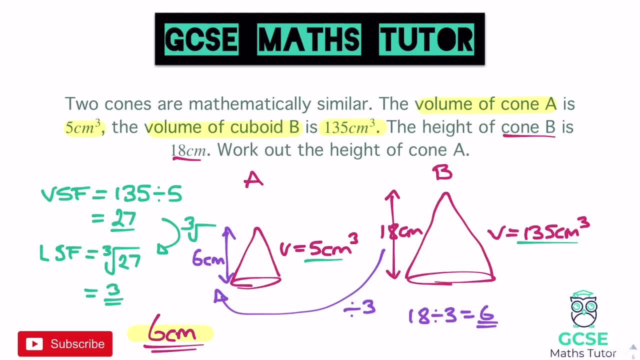 As it's a length, this time There we go, 6 centimetres Right. here's a couple for you to have a go at. then Just obviously think about which scale factor you're finding the area or the volume, And then just remember how to get back to length from that. 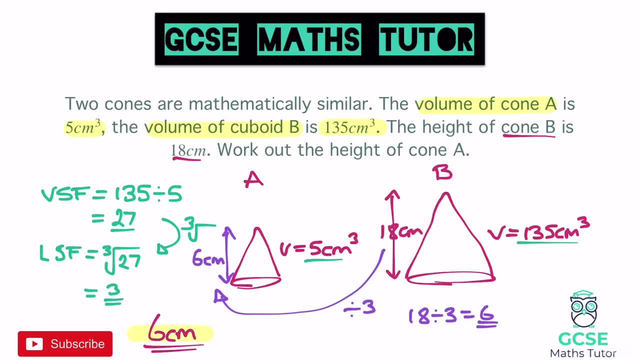 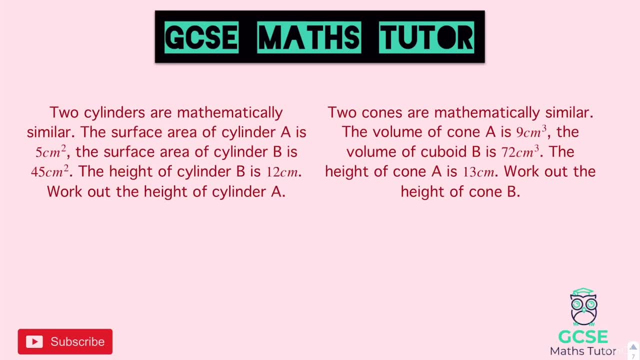 So square root the area to get back to length, or cube root the volume to get back to length. OK, here they are. OK. so two questions there. Pause the video and we'll go over the answers in a sec, Right, OK? so for this first question we are given the surface areas. 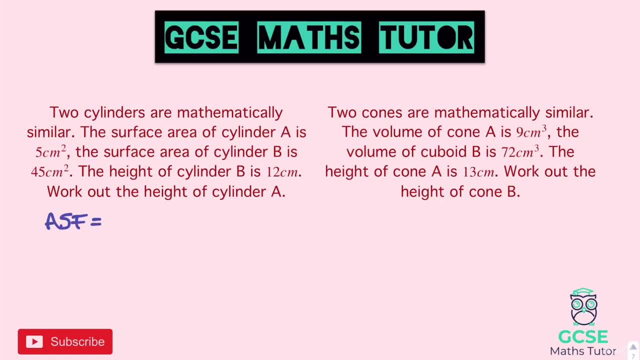 So I can find the area scale factor by doing the bigger area, which is 45.. And dividing it by the smaller area, which is 5.. And 45 divided by 5 is 9.. You will tend to notice not all the time, but you will tend to notice that a lot of the time square numbers or cube numbers come up in these. 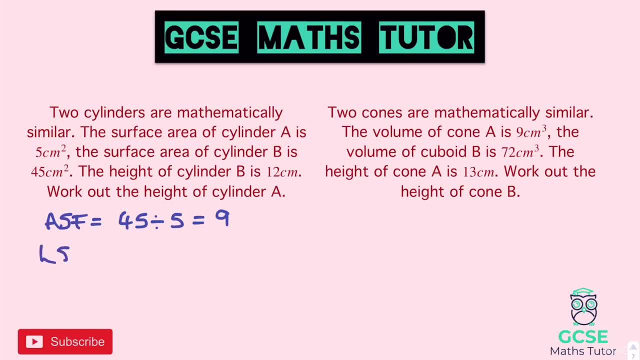 So knowing them is obviously very helpful. Now to get the length scale factor: as that's an area, we need to square root it, So the square root of 9,, which is 3.. Now, in this question here, let's just have a quick look. 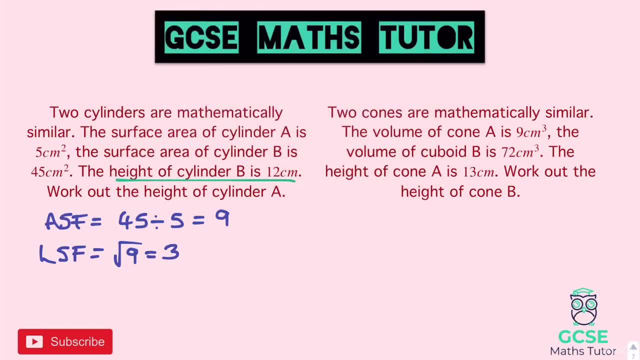 We are going from the height of cylinder B is 12.. Now B is the one with the larger area. So obviously you could draw a picture for this one. But if we're going from the larger one to the smaller one, we're going to do 12.. 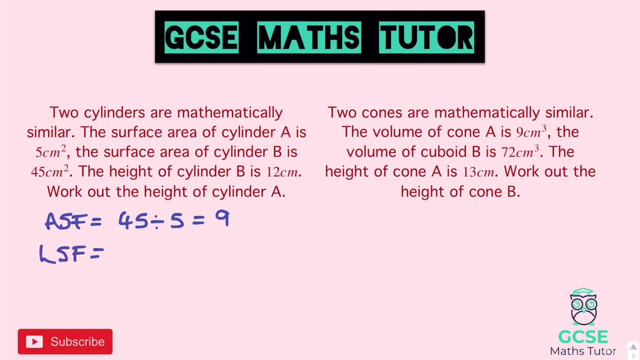 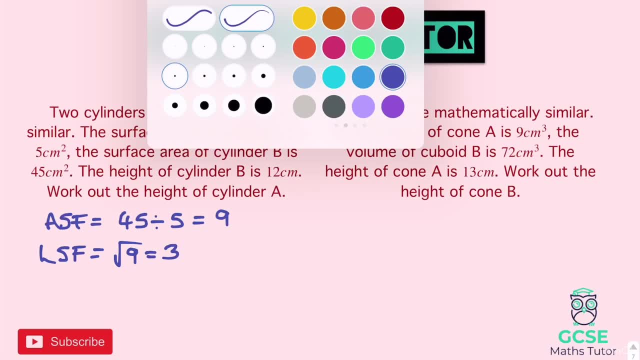 Now to get the length scale factor. as that's an area, we need to square root it. So the square root of 9,, which is 3.. Now in this question here, let's just have a quick look- We are going from: the height of cylinder B is 12.. 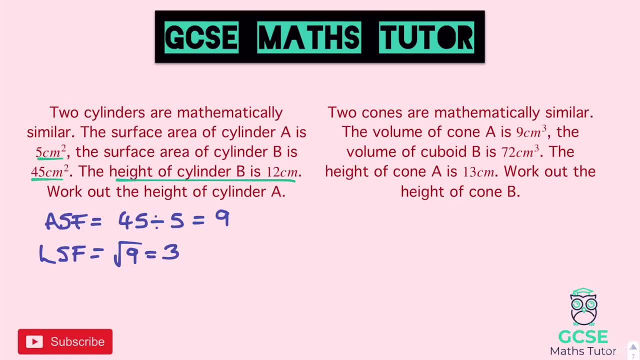 Now, B is the one with the larger area, so obviously you could draw a picture for this one. but if we're going from the larger one to the smaller one, we're going to do 12 and we're going to divide that by the length scale factor. 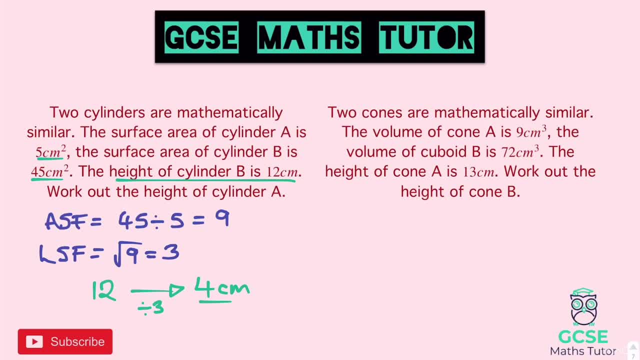 So divide that by 3 and that will give us 4 centimetres for the height of cylinder A. You can already see, just by me doing my working out here, it's a lot easier and a lot clearer when you do draw a picture. 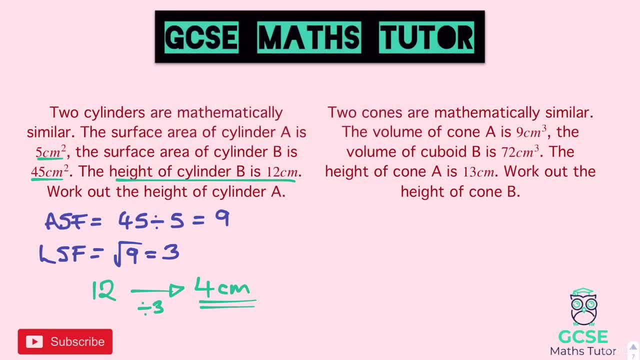 So I do encourage you to make sure that you do draw a picture for all of these, But obviously, just as we've got limited space on here as well, and we've already gone through lots of questions, I'm not going to draw the pictures for these two. 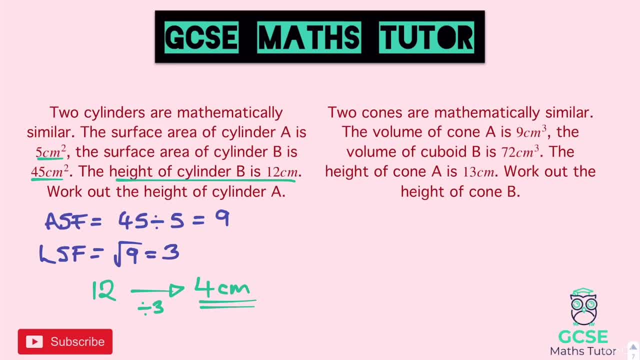 Just get any of the answers. So for the next one, Let's have a look at what we've got. We have a volume of A and B and it's 72 and 9. So we can get a volume scale factor by doing 72. 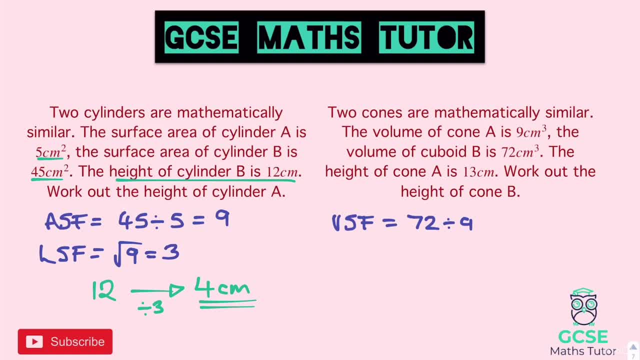 divided by 9 and 72 divided by 9 is 8.. There we go. Now. to get from volume back to length, we need to cube root. So I need to do the cube root of 8, and the cube root of 8 is 2.. 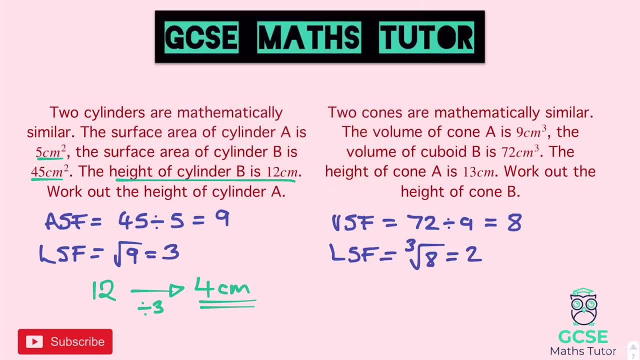 Now we've got the length scale factor. Let's have a look. It says the height of cone A is 13.. Cone A is the smaller one. So to get from 13 to the bigger shape, we're going to times it by 2,. 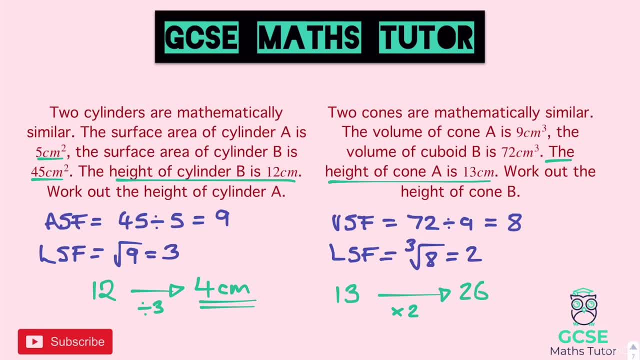 the length scale factor, which gives us 26 centimetres. And there we go. There's our final answer for that one. Right, OK, we're going to look at something else now. Let's have a look, Right, OK? so we're going to put this all together now. 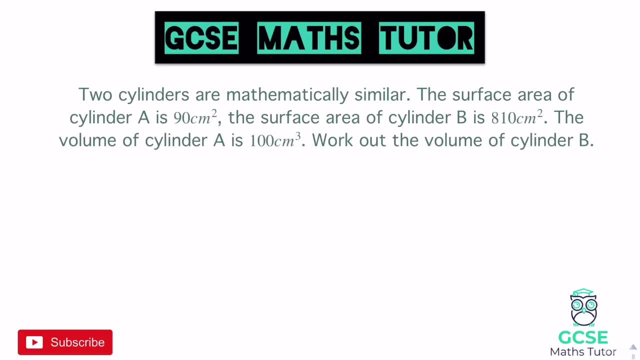 It says two cylinders are mathematically similar. The surface area of cylinder A is 90 and the surface area of cylinder B is 810.. The volume of cylinder A is 100.. Work out the volume of cylinder B. OK, so first things first. we can do a diagram for this one, and I'm going to go for it. 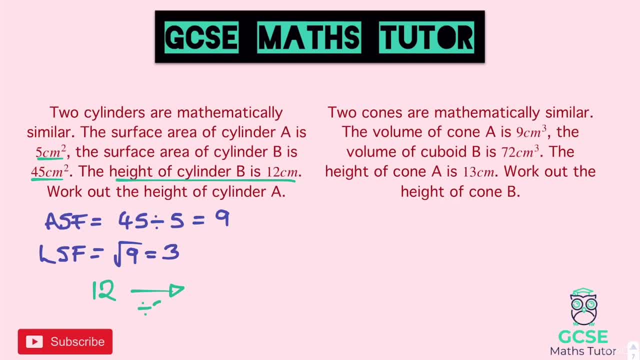 And we're going to divide that by the length scale factor. So divide that by 3. And that will give us 4 centimetres for the height of cylinder A. You can already see, just by me doing my working out here, it's a lot easier and a lot clearer when you do draw a picture. 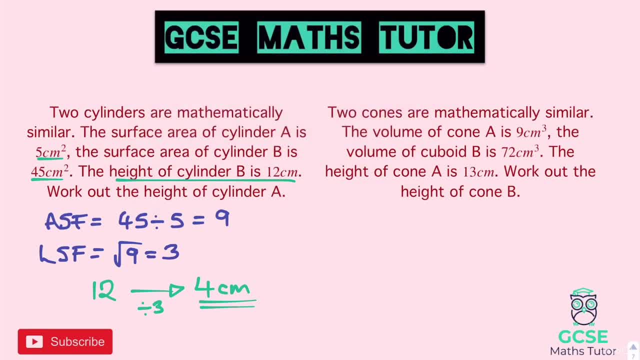 So I do encourage you to make sure that you do draw a picture for all of these, But obviously, just as we've got limited space on here as well and we've already gone through lots of questions, I'm not going to draw the pictures for these two. just get any of the answers. 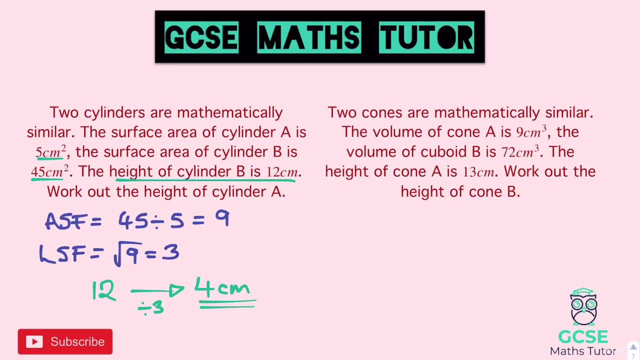 So for the next one, let's have a look at what we've got. We have a volume of A and B and it's 72 and 9.. So we can get a volume scale factor by doing 72 divided by 9.. 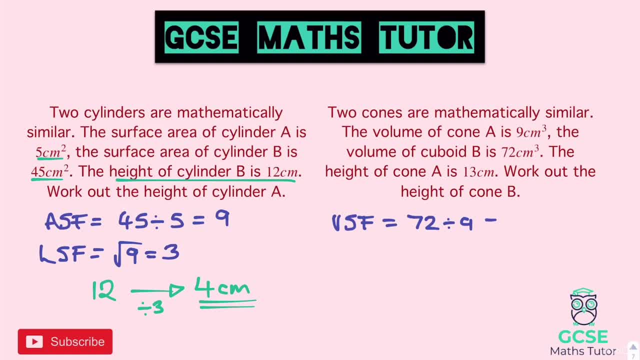 And 72 divided by 9 is 8.. There we go. Now to get from volume back to length, we need to cube root. So I need to do the cube root of 8.. And the cube root of 8 is 8.. 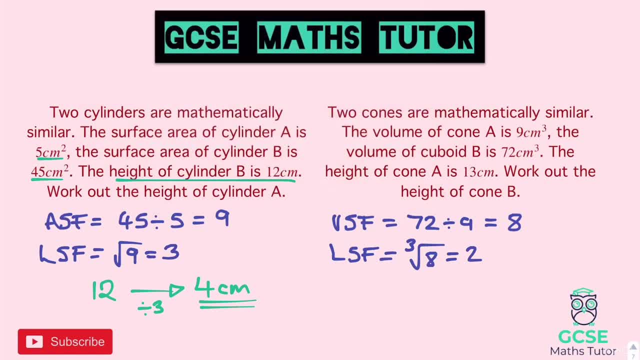 2.. Now we've got the length scale factor. Let's have a look. It says the height of cone A is 13.. Cone A is the smaller one. So to get from 13 to the bigger shape, we're going to times it by 2,. 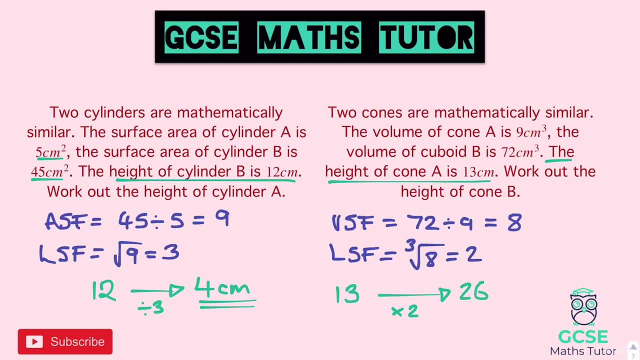 the length scale factor, which gives us 26 centimetres. And there we go. There's our final answer for that one. Right, OK, we're going to look at something else now. Let's have a look, Right, OK? so we're going to put this all together now. 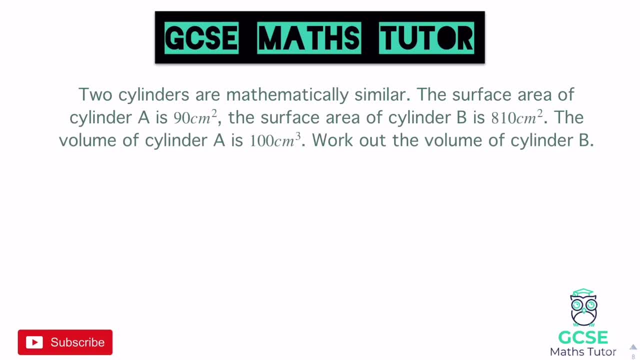 It says two cylinders are mathematically similar. The surface area of cylinder A is 19.. The surface area of cylinder B is 810.. The volume of cylinder A is 100.. Work out the volume of cylinder B. OK. so first things first, we can do a diagram for this one. 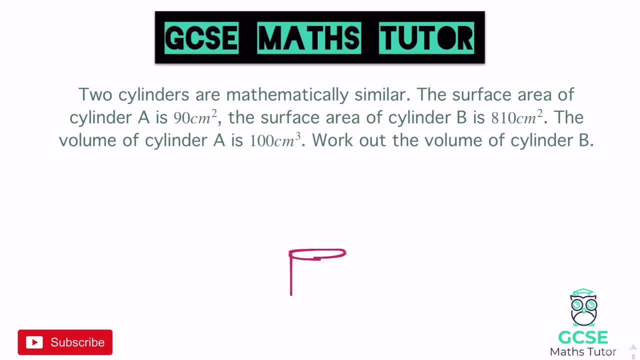 And I'm going to go for it. I'm going to do cylinder A. It's a cylinder, OK, I'm just going to draw it a bit smaller this time. So cylinder A And we have cylinder B. There we go, cylinder B. 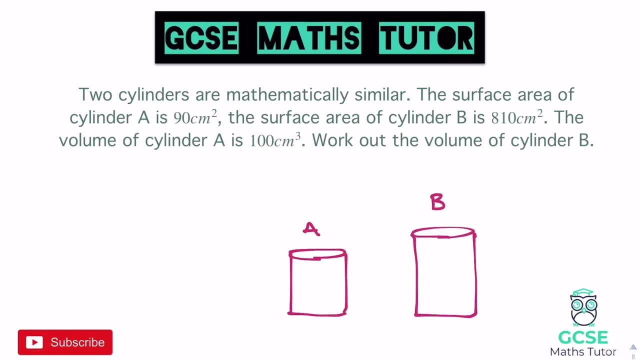 Now it says the surface area of A is 90 centimetres squared. So the surface area is 90.. And for this one the surface area equals what's it say, 810.. Right, then. it also says the volume of A is 100 centimetre cubed. 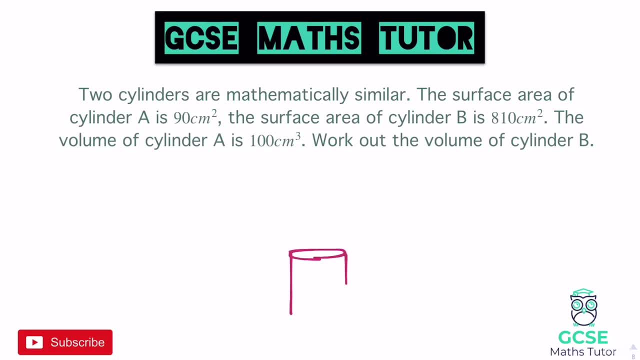 I'm going to do cylinder A. It's a cylinder. OK, I'm going to draw it a bit smaller this time. So cylinder A and we have cylinder B. There we go, cylinder B. Now. it says the surface area of A is 90. 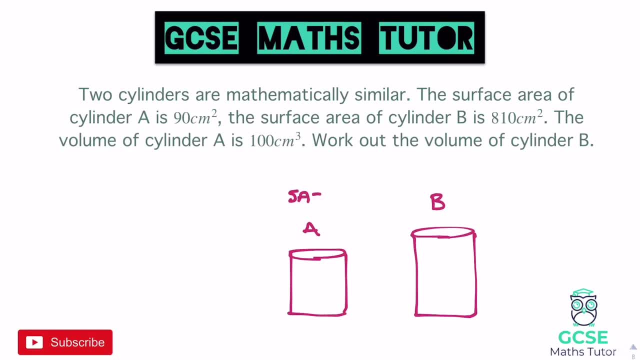 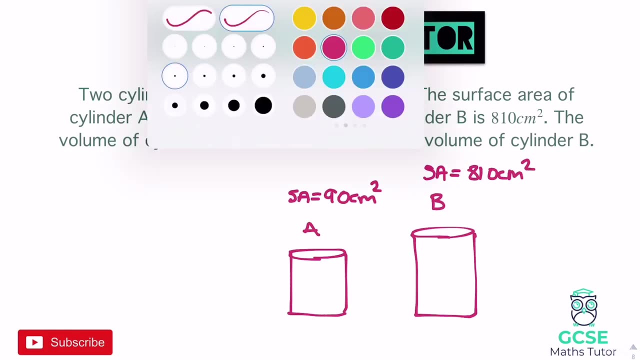 centimetres squared, So the surface area is 90.. And for this one, the surface area equals what's it say, 810.. Right then. it also says the volume of A is 100 centimetre cubed. I'm going to change the colour for this one. 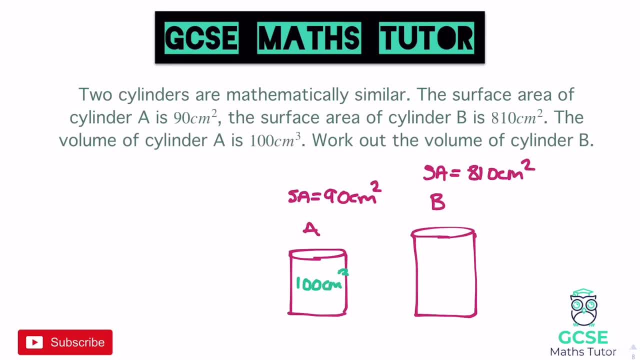 100 centimetre cubed And it wants us to work out the volume of cylinder B. So in this circumstance, here we need to have a look at all three scale factors, and I'll explain why. here Let's have a look. 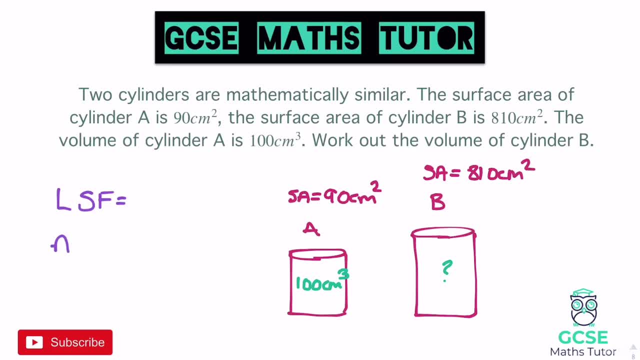 But always just write all these down to the side anyway, just to remind yourself. So, area scale factor, length scale factor and finishing off with our volume scale factor. Now the only thing we need to be careful of here is if we have a look in the 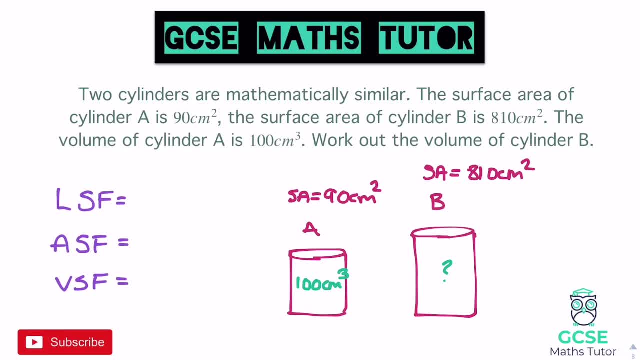 question. we're told about area and we're told about volume. Now there's not one step for moving between these two scale factors. OK, there's no way that I can just move straight from area to volume or straight from volume to area. 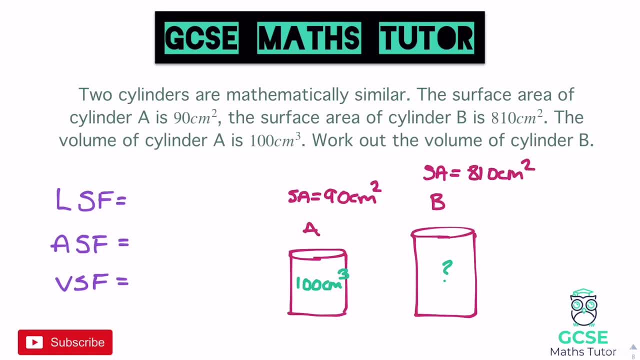 So what I'm going to have to do is figure out which one I can actually work out, and we'll talk about how we can go about this. So it says here: the surface area of A is 90 and the surface area of B is 810. 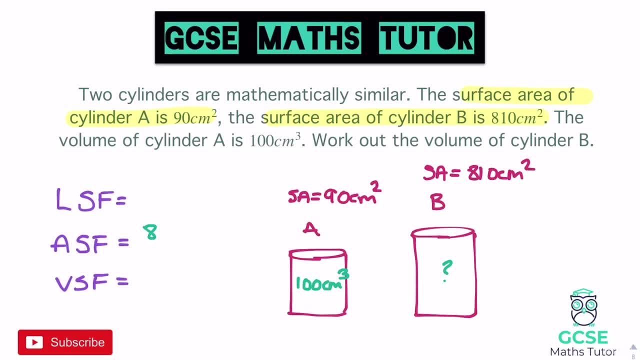 So we can definitely work out the area scale factor, because we can do 810, the bigger shape divided by 90.. 81 divided by 9 is 9, so 810 divided by 90 is also 9.. There we go, So my area scale factor is 9.. 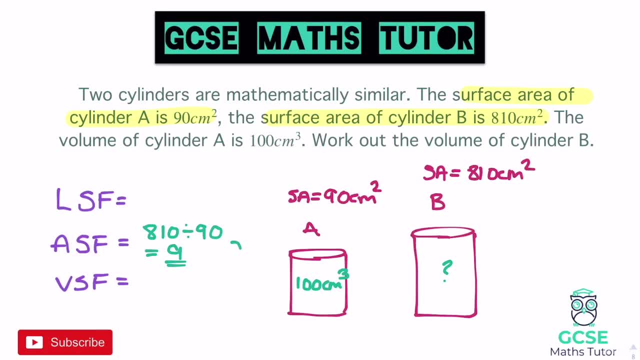 Now we want to work out a volume And, as I said, there's no way of jumping straight from area to volume, but we can go from area back to length And then, once we've got length, we can move down to volume. 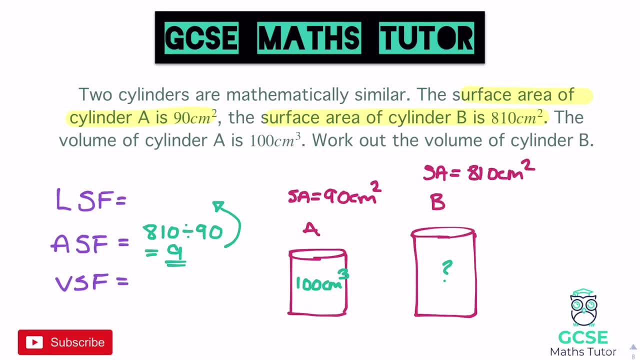 OK, so I can kind of do it in a bit of a rotation there. So first things first, how did we get from area back to length? Well, that was doing a square root. So to get the length I can do the square. 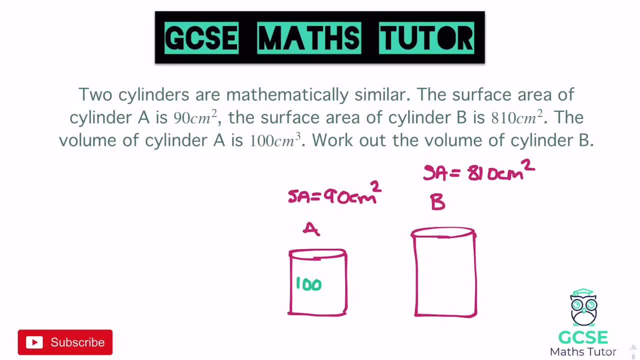 I'm going to change the colour for this one, 100 centimetre cubed, And it wants us to work out the volume of cylinder B. So in this circumstance here we need to have a look at all three scale factors. 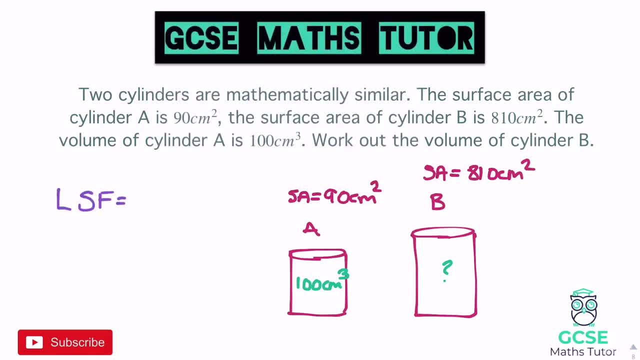 And I'll explain why here. Let's have a look, But always just write all these down to the side anyway, just to remind yourself. So, area scale factor, length scale factor and finishing off with our volume scale factor. Now the only thing we need to be careful of here is: 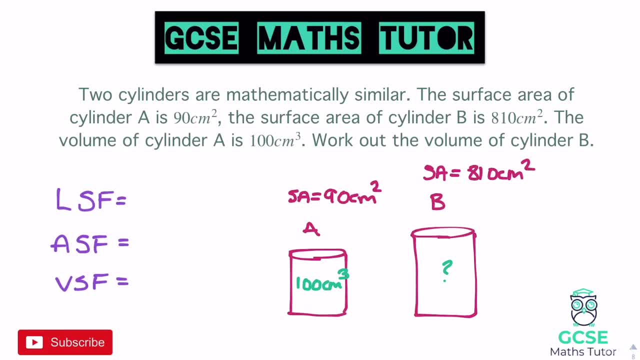 if we have a look in the question, we're told about area and we're told about volume. Now, there's not one step for moving between these two scale factors. OK, there's no way that I can just move straight from area to volume. 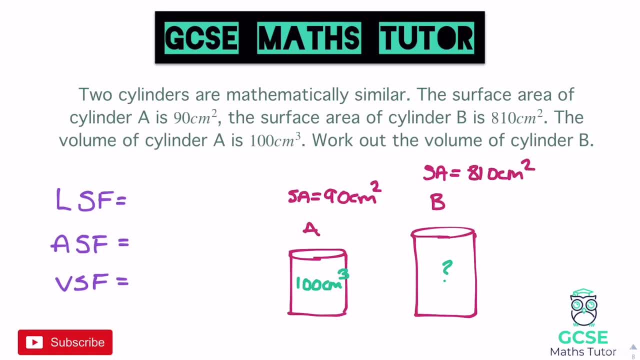 or straight from volume to area. So what I'm going to have to do is figure out which one I can actually work out. We'll talk about how we can go about this. So it says here: the surface area of A is 90 and the surface area of B is 810. 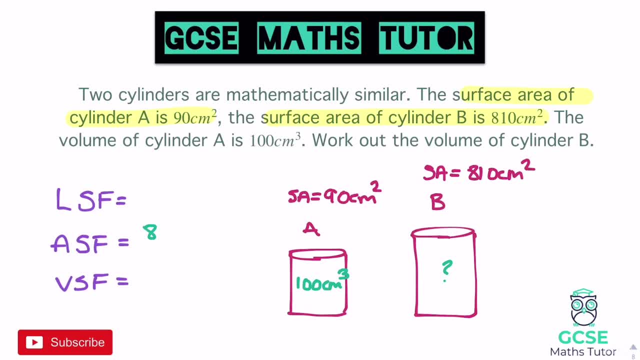 So we can definitely work out the area scale factor, because we can do 810, the bigger shape divided by 90.. 81 divided by 9 is 9.. So 810 divided by 90 is also 9.. There we go. 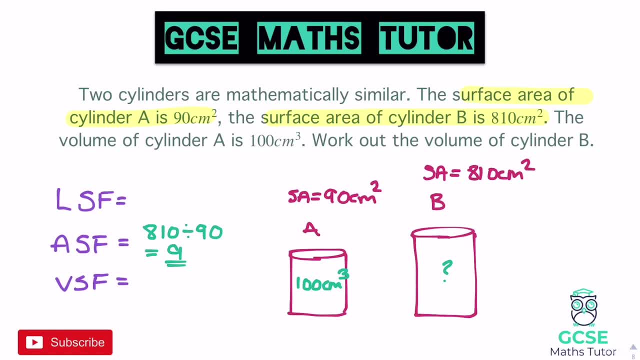 So my area scale factor is 9.. Now we want to work out a volume And, as I said, there's no way of jumping straight from area to volume. But we can go from area back to length And then, once we've got length, we can move down to volume. 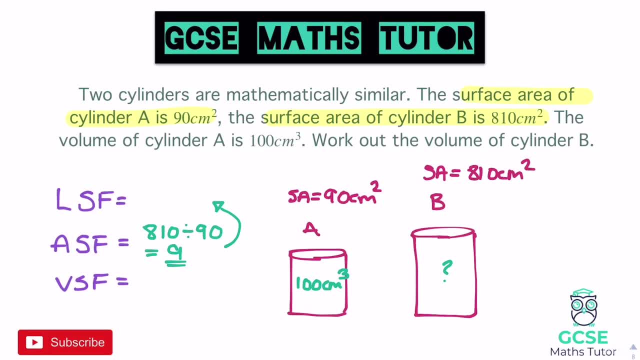 OK, so I can kind of do it in a bit of a rotation there. So first things first, how did we get from area back to length? Well, that was doing a square root. So to get the length, I can do the square root of 9,. 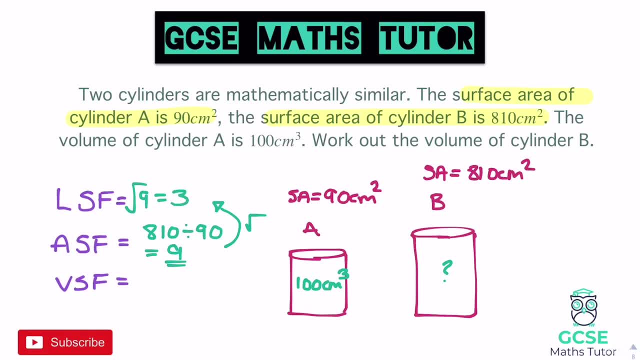 which gives me a length scale factor of 3,. just like on the last question, Now that we have a length of 3, I can move from length down to volume. How did we do that? We cubed it So to get from length to volume. 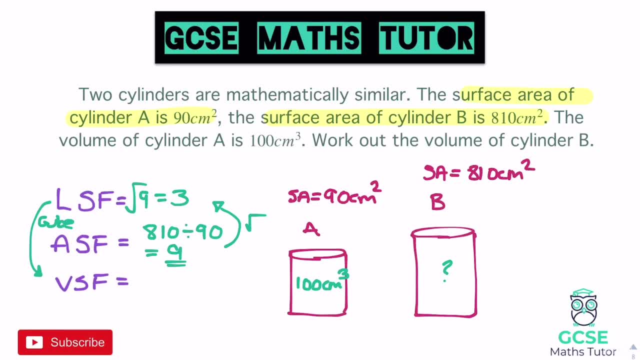 we cubed the scale factor and that's cubing the length scale factor. So to get to volume, I can do 3 cubed. 3 cubed is 27.. OK, so it's always about moving back to the length scale factor. 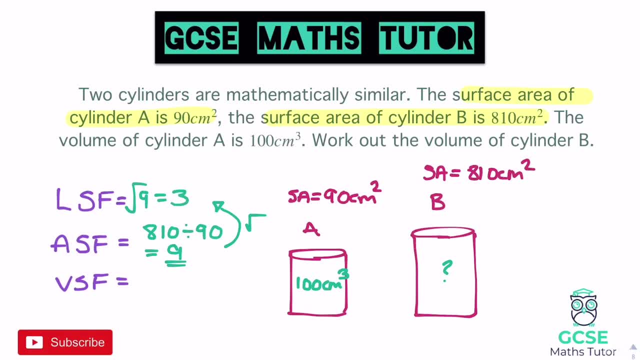 root of 9, which gives me a length scale factor of 3.. Just like on the last question, Now that we have a length of 3, I can move from length down to volume. How did we do that? We cubed it. 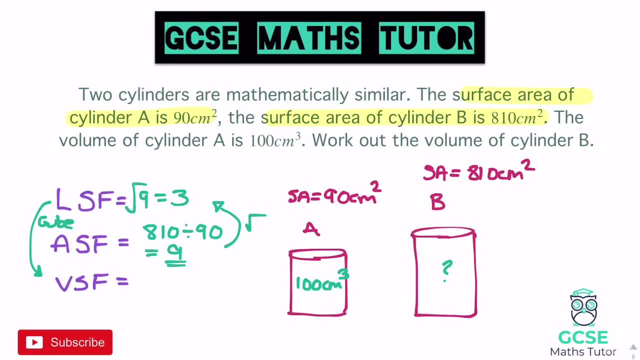 So to get from length to volume, we cube the scale factor, and that's cubing the length scale factor. So to get to volume, I can do 3 cubed. 3 cubed is 27.. OK, so it's always about moving back to the length scale factor, and that means 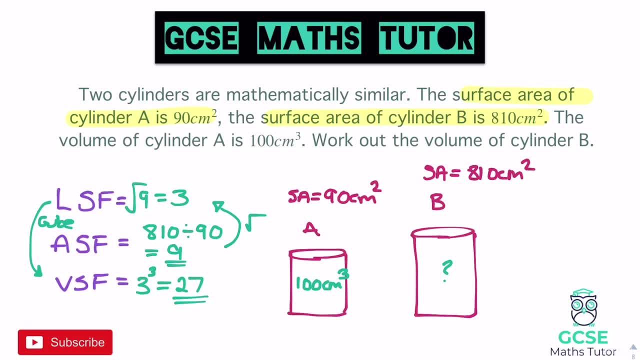 either square rooting or cube rooting, depending on which scale factor we start with. As we started with area, we square root to go backwards and then cube that answer to get down to our volume scale factor. OK, so now we've got that. we can finish this off. 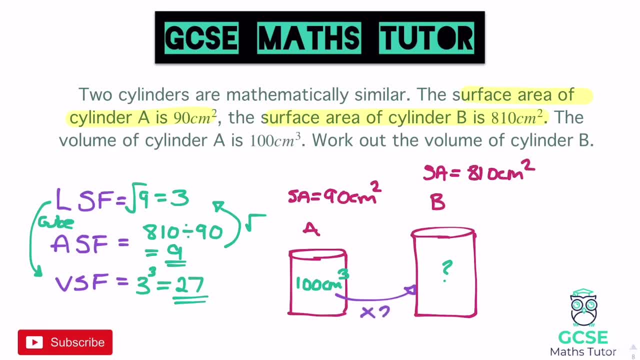 We're going from the small to the big. so we can times by 27, the volume scale factor, which is 2700 centimetres cubed. OK, 100 times 27 there. So there's our final answer: 2700 centimetre cubed. 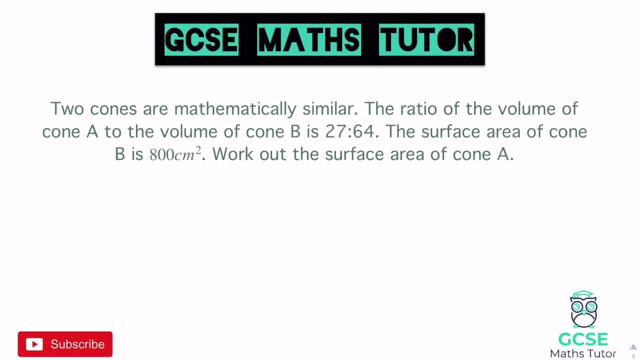 We're going to have a look at one more before you have a go. OK, now, a very similar process in this question, but, as you can see- you might have spotted it- there's a ratio here, so we'll have a look at how we deal. 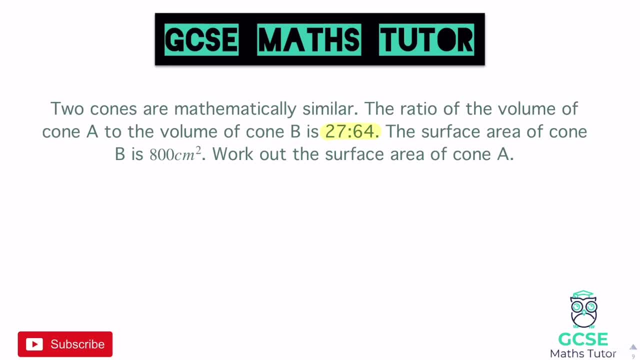 with it when there's a ratio. So two cones are mathematically similar. The ratio of the volume of cone A to the volume of cube B is 27 to 64, and the surface area of cone B is 800.. Work out the surface area of cone A. 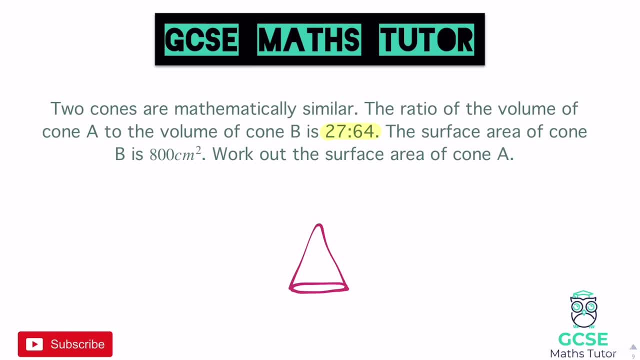 Now let's just draw a little picture for this one. So we've got a cone, there we go, and a bigger one, cone B. So we've got A and B and it's given us the volumes Now, as they are in the ratio of 27 to 64,. 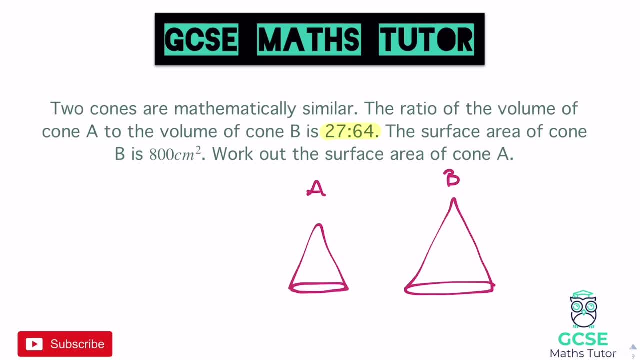 it doesn't actually matter what the volume is, as long as we know what the what, the ratio is. So the volume of the smaller one, let's say, is just 27.. OK, we'll talk about this a bit more, but let's just say the volume of the other one is 64.. 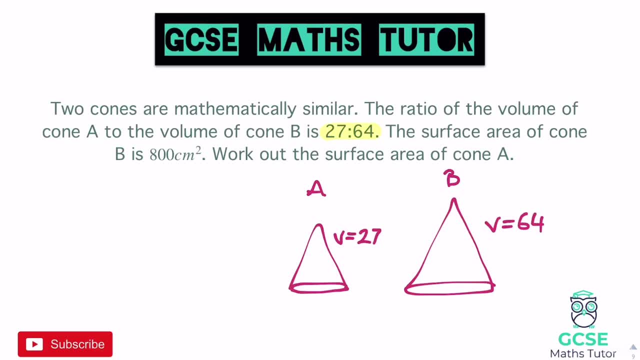 Now, because it's in the ratio of 27 to 64, it could be any multiple of 27 and 64 in that ratio. OK, so let's just imagine we double them both: 54 and 128.. Doing the big divided by the little is always going to give us. 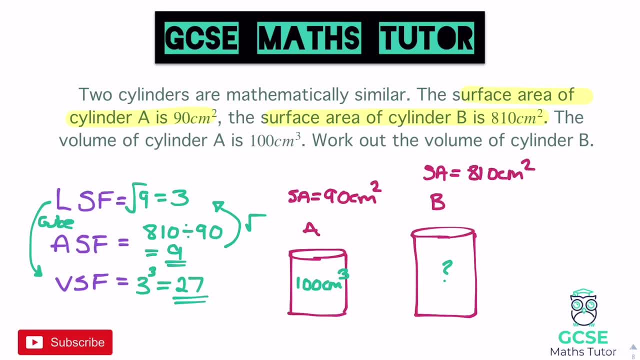 And that means either square rooting or cube rooting, depending on which scale factor we start with. As we started with area, we square root to go backwards And then cube that answer to get down to our volume scale factor. OK, so now we've got that, we can finish this off. 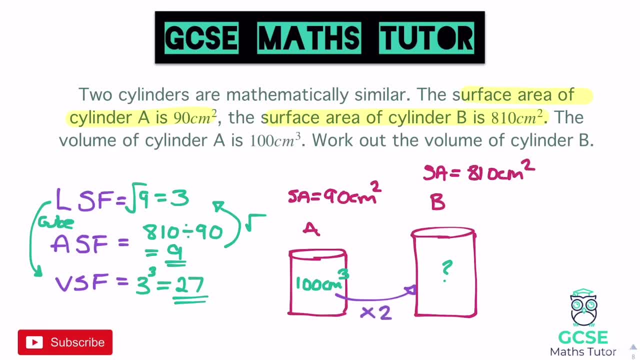 We're going from the small to the big. So we can times by 27 the volume scale factor, which is 2700 centimetres cubed. OK, 100 times 27 there. So there's our final answer: 2700 centimetre cubed. 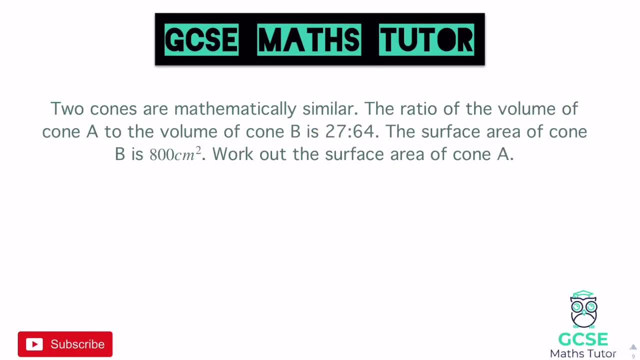 We're going to have a look at one more before you have a go. OK, now a very similar process in this question, but, as you can see- you might have spotted it- There's a ratio here, So we'll have a look at how we deal with it when there's a ratio. 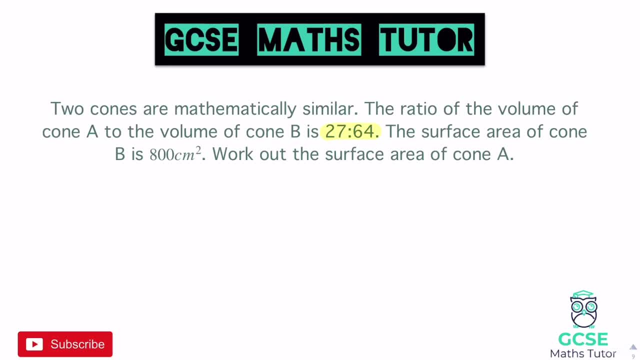 So two cones are mathematically similar. The ratio of the volume of cone A to the volume of cube B is 27 to 64. And the surface area of cone B is 800.. Work out the surface area of cone A. Now let's just draw a little picture for this one. 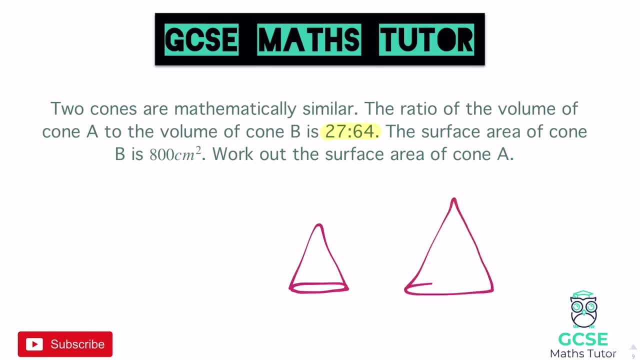 So we've got a cone, there we go, and a bigger one, cone B. So we've got A and B and it's given us the volumes. Now, as they are in the ratio of 27 to 64, it doesn't actually matter what the volume is. 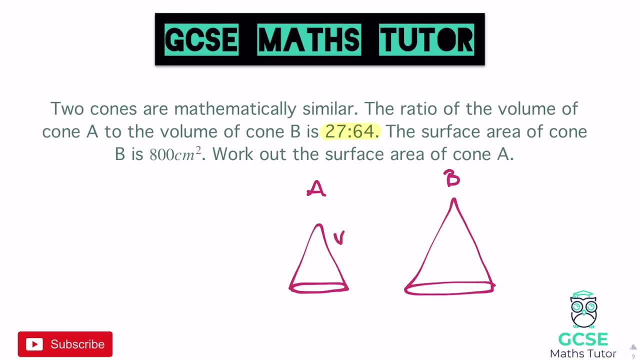 as long as we know what the ratio is. So the volume of the smaller one, let's say, is just 27.. OK, we'll talk about this a bit more, but let's just say the volume of the other one is 64.. 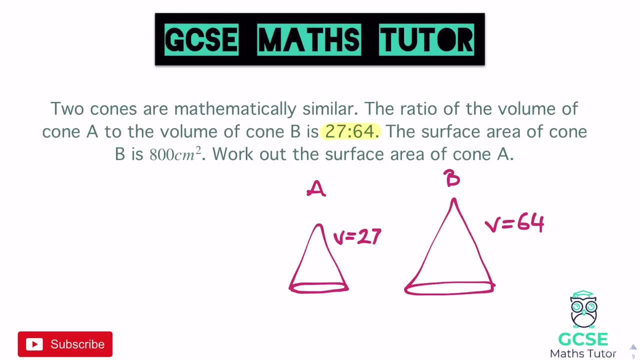 Now, because it's in the ratio of 27 to 64, it could be any multiple of 27 and 64 in that ratio. OK, so let's just imagine we double them both: 54 and 128.. Doing the big divided by the little. 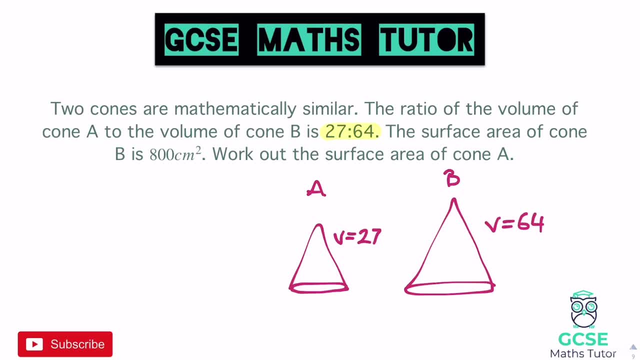 is always going to give us the same answer there, because obviously it's kept in the same ratio. So it doesn't actually matter if we use the smallest possible answer here, which is 27 and 64. We can just use that instead as our big divided by little. 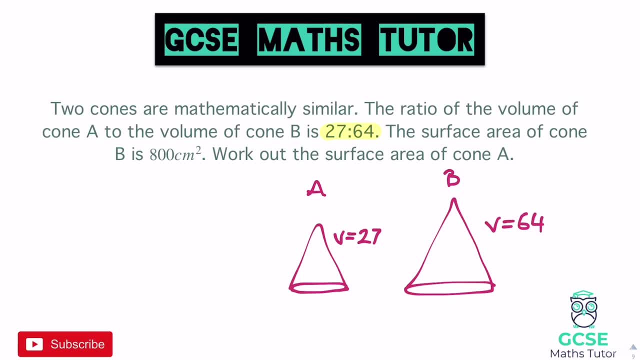 to get our scale factor. OK, it doesn't matter that it's in a ratio. We'll just label it 27 and 64.. OK, so let's also label this last piece of information. It says the surface area of cone B is 800 centimetres squared. 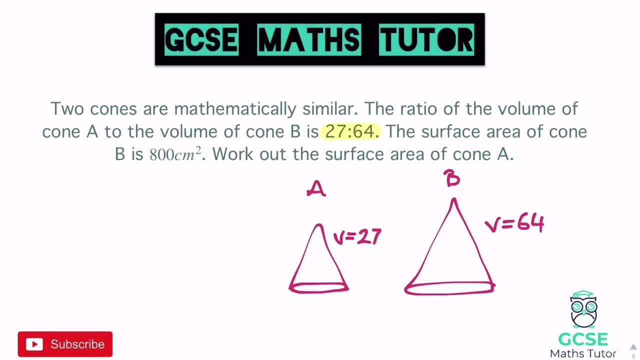 the same answer there, because obviously it's kept in the same ratio. So it doesn't actually matter if we use the smallest possible answer here, which is 27 and 64. We can just use that instead as our big divided by little to get our scale factor. 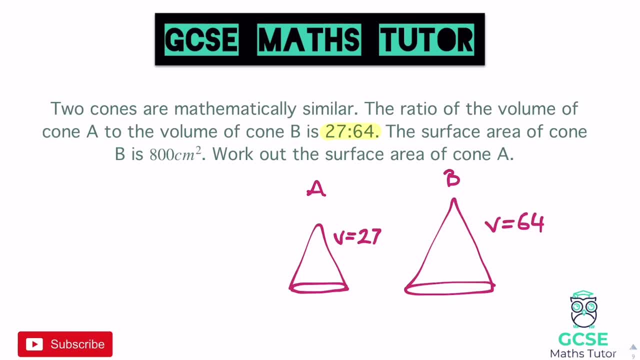 OK, it doesn't matter that it's in a ratio. We'll just label it 27 and 64.. OK, so let's also label this last piece of information. It says the surface area of cone B is 800 centimetres squared. 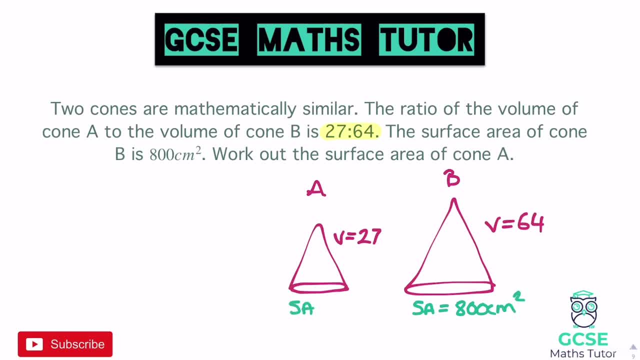 There we go. And it wants us to work out the surface area of A. OK, so moving that to our scale factors, then we've got length scale factor, area scale factor and volume scale factor. There we go, So we've been given the volumes. 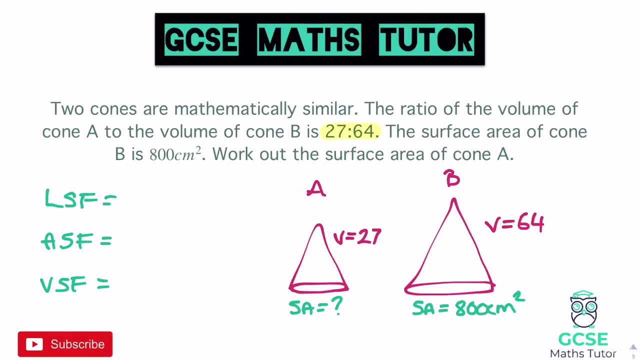 Well, obviously we've been given the ratio of the volumes, So all we have to do is do: the big one divided by the little one again, which is 64 divided by 27.. OK, obviously, these volumes are obviously going to be a lot bigger than that, particularly as the surface area is 800. 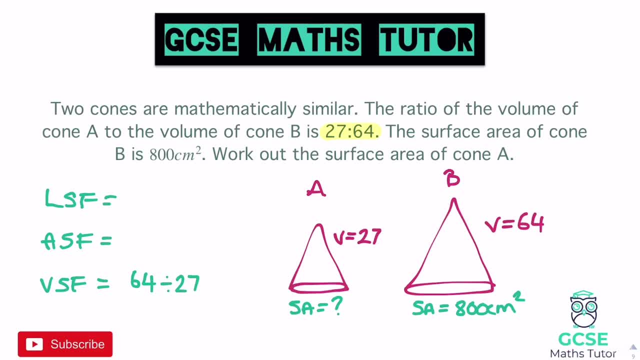 But it doesn't matter how big we make these numbers, It will always be within the same ratio, So we can just use the smallest numbers here. It's going to give us the same answer. So 64 divided by 27.. This is definitely a calculator question. 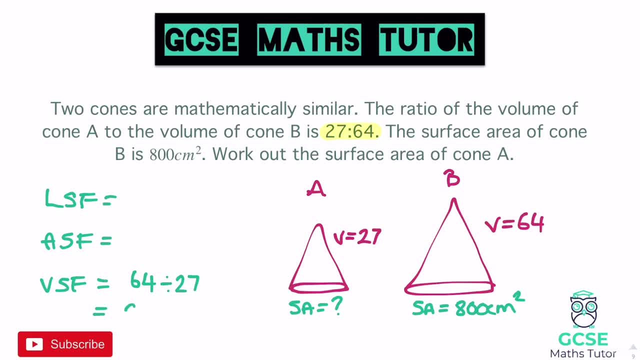 Gives us an answer and it's really not very nice. It comes out as 2.3.. That's not a three: 2.370.. OK, and there's a recurring dot above the three and the nought. Now, this is very, very important at this point. 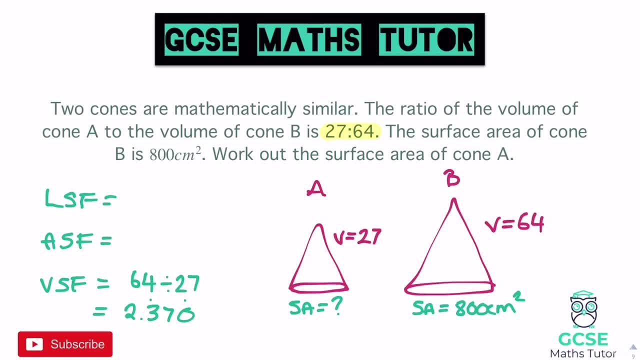 We need to leave that answer in the calculator screen? OK, because this is going to massively affect our answer. If we definitely don't want to round this, because it will massively affect our scale factors if we do so Now, again, we need to get from volume to area. 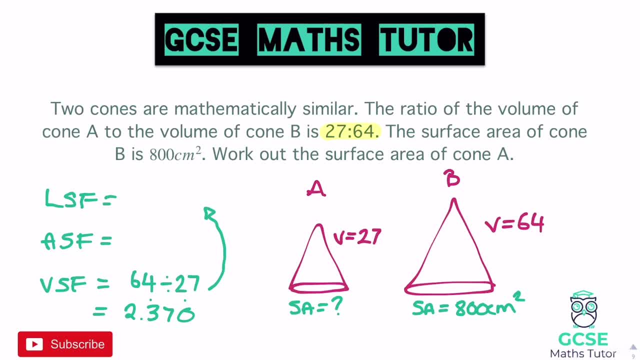 And the only way to do that is to first return back to length. And the way to get from volume back to length, that was a cube root. So I need to cube root that number there And to do that on the calculator you're going to have to press cube root answer. 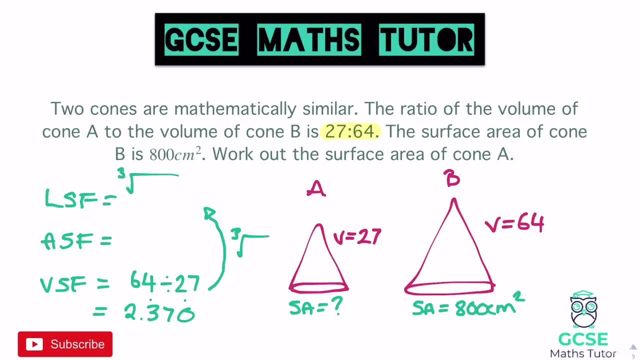 OK, So press your cube root button and then press your answer button which is next to the equal sign, And that's just going to cube root the answer on the calculator. So on my calculator it just says cube root answer. I'm going to put the decimal under here. 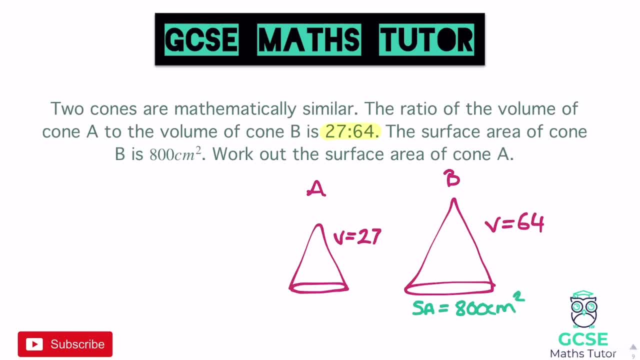 There we go. And it wants us to work out the surface area of A. OK, so moving that to our scale factors, then we've got length scale factor, area scale factor and volume scale factor. There we go, So we've been given the volumes. 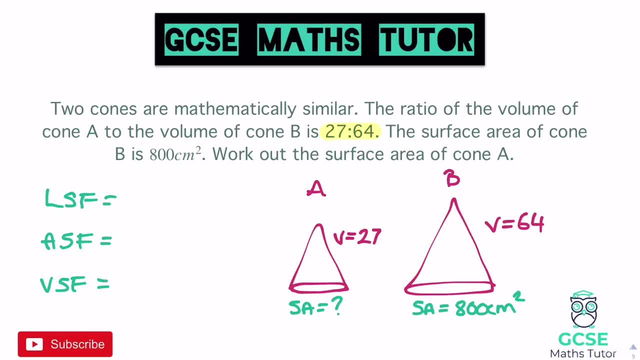 Well, obviously we've been given the ratio of the volumes, So all we have to do is do the big one divided by the little one again, which is 64 divided by 27.. OK, obviously, these volumes are obviously going to be a lot bigger than that. 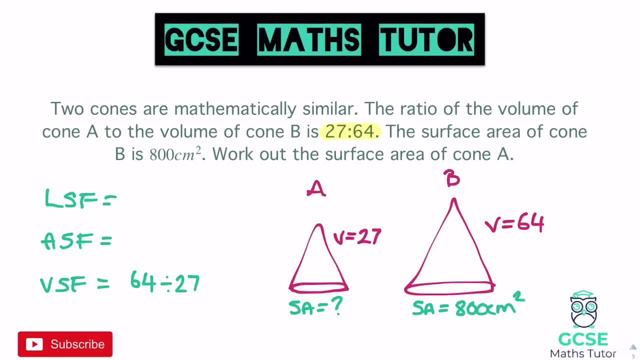 particularly as the surface area is 800.. But it doesn't matter how big we make these numbers. It will always be within the same ratio. So we can just use the smallest numbers here. It's going to give us the same answer. So 64 divided by 27.. 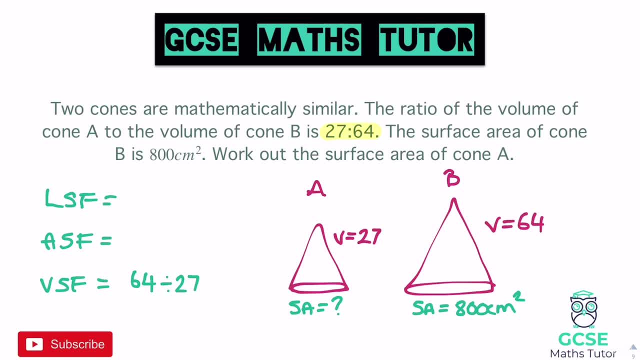 This is definitely a calculator question- Gives us an answer and it's really not very nice. It comes out as 2.3.. That's not a three: 2.370.. OK, and there's a recurring dot. It's above the three and the nought. 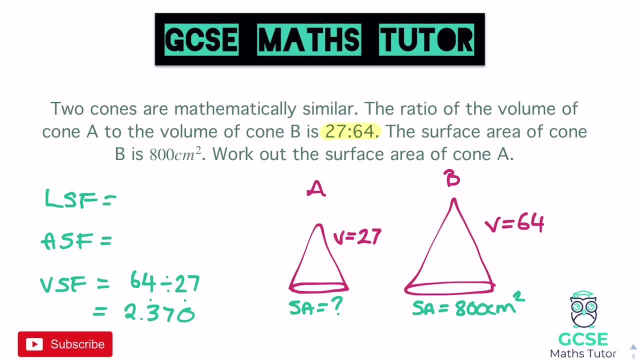 Now this is very, very important at this point. We need to leave that answer in the calculator screen. OK, because this is going to massively affect our answer. We definitely don't want to round this, because it will massively affect our scale factors if we do so. 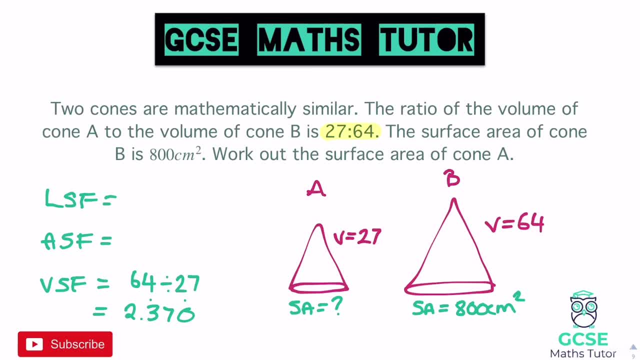 Now again, we need to get from volume to area, And the only way to do that is to first return back to length. And the way to get from volume back to length, that was a cube root, So I need to cube root that number there. 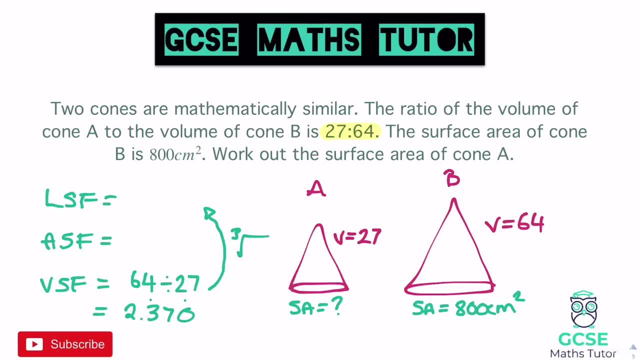 And to do that on the calculator you're going to have to press cube root answer. OK, so press your cube root button and then press your answer button, which is up next to the equal sign, And that's just going to cube root the answer on the calculator. 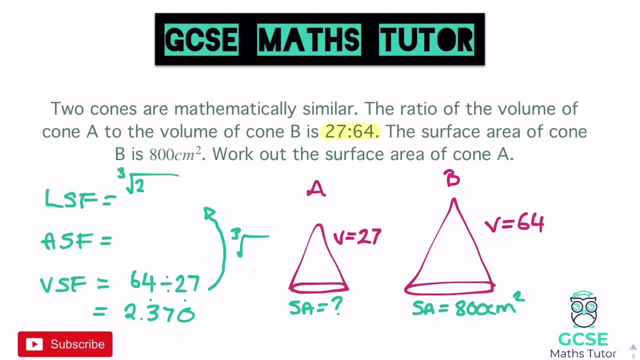 So on my calculator it just says cube root answer. I'm going to put the decimal under here: 2.370 dots above the three and the zero. You'll see if you type in cube root of 2.370,. I don't do that right now. 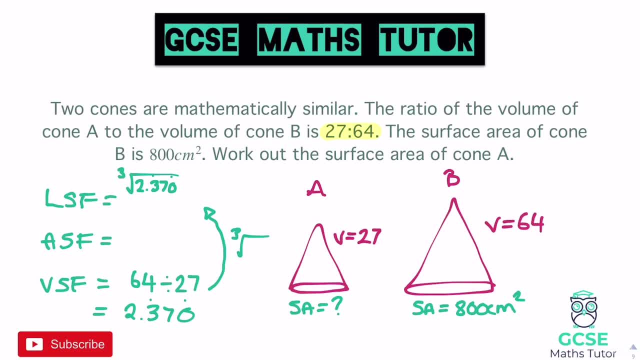 But if you do type that in, you're not going to get the same answer as we're going to get right now. So I'm going to press cube root answer equals And I get four thirds on my calculator screen, which is 1.3 recurring. 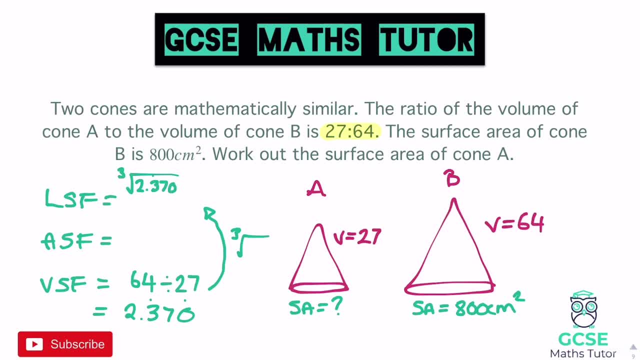 Two point three seven zero dots above the three and the zero. You'll see if you type in cube root of two point three seven zero. I don't do that right now, but if you do type that in, you're not going to get the same answer as we're going to get right now. 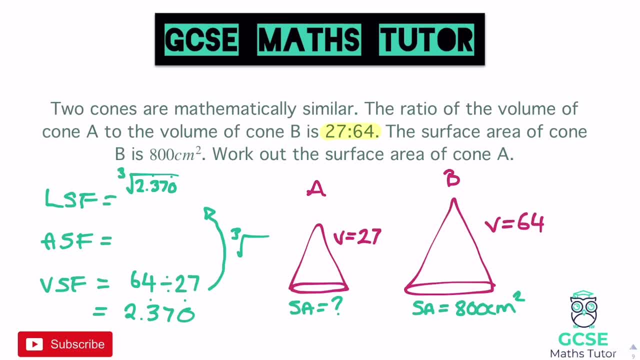 So I'm going to press cube. root answer equals. I get four thirds on my calculator screen, which is one point three recurring. I'm going to write it as the decimal version, but it comes up as four thirds. I'm going to write that in as well. 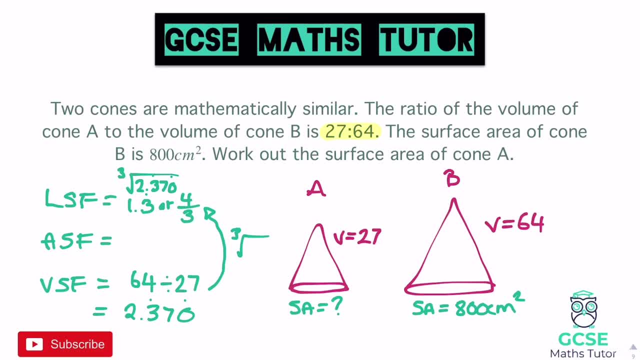 Four thirds. OK, if you round that you will not get four thirds. And in fact, if I test that out right now, if I cube root two point three, seven, zero, I get one point three, three, three, two, six, three, eight. 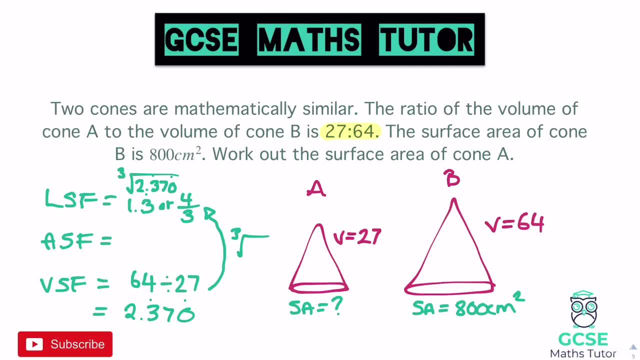 So it's very close, but it's not two thirds, Sorry, four thirds. So I want to just put four thirds back into my calculator And there we go, sticking with four thirds. Now to finish this off, obviously we're looking at area. 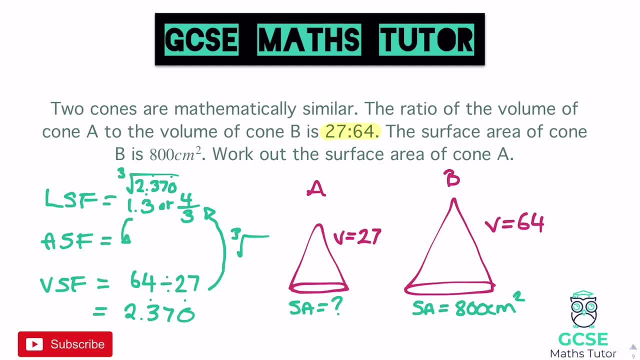 So to get back down from length to area, how do we do that? We square it. OK, so I'm going to do this in a different colour because it's getting a bit lost. OK, so to get from length to area, square your answer. 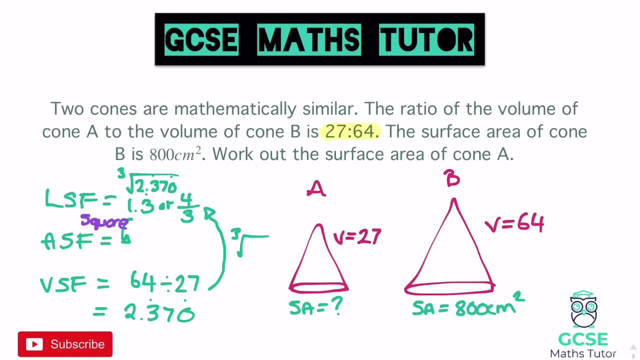 So we want four thirds squared or one point three recurring squared. So square answer equals And you get one point seven recurring. Not very nice at all this question. There we are. So one point seven recurring is the scale factor that we need there. one point seven recurring. 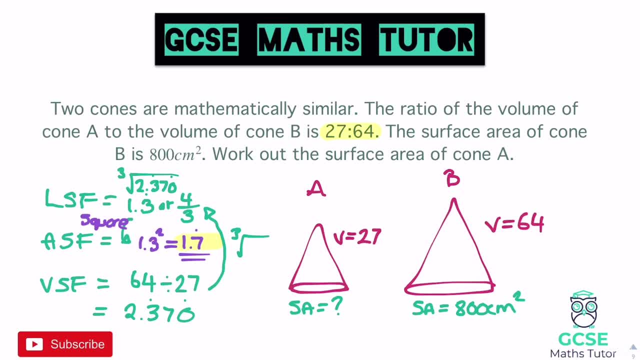 OK, so a little bit nasty there. Obviously we are. it's already quite difficult moving between the lengths of all human area scale factors. You just have to be very careful, when these decimals do come up on your calculator, that you just keep using the answer on your calculator screen. 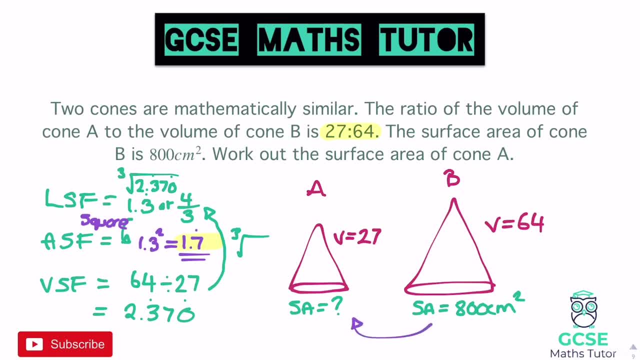 But from here it's nice and easy. We're going from the big down to the small, We're using the area scale factor, big to small, we're going to divide. So divide by one point seven, recurring. So what I would do is leave one point seven recurring on your calculator screen. 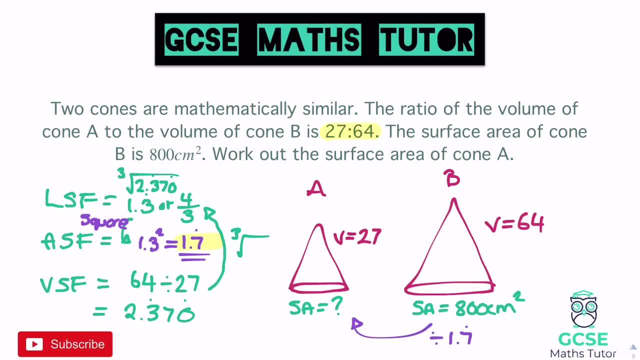 Type in eight hundred, divide by and again use the answer button. It will just put that one point seven recurring in for you. So eight hundred divided by answer, and you should get four hundred and fifty. So just make sure that you can do that on your calculator. 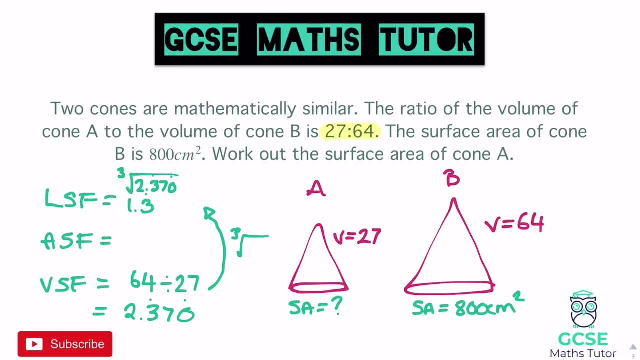 OK, I'm going to write it as the decimal version, but it comes up as four thirds. I'm going to write that in as well. Four thirds, OK, if you round that, you will not get four thirds. In fact, if I test that out right now, if I cube root 2.370, I get 1.3332638. 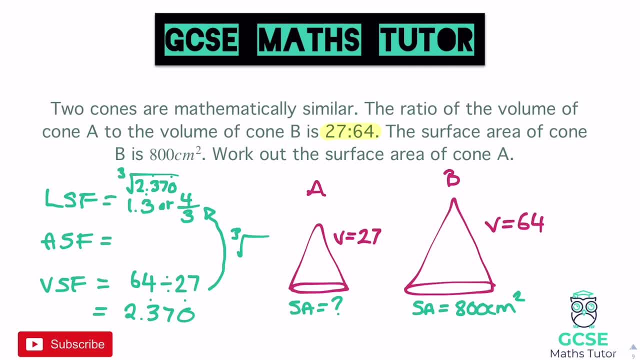 So it's very close, but it's not two thirds, sorry, four thirds. So I want to just put four thirds back into my calculator And there we go, sticking with four thirds. Now to finish this off, obviously we're looking at area. 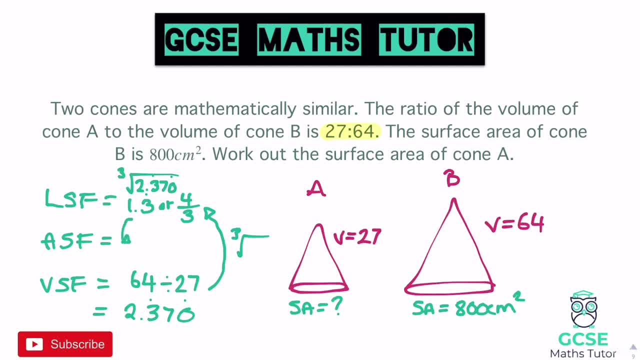 So to get back down from length to area, how do we do that? We square it. OK, so I'm going to do this in a different colour because it's getting a bit lost. OK, so to get from length to area, square your answer. 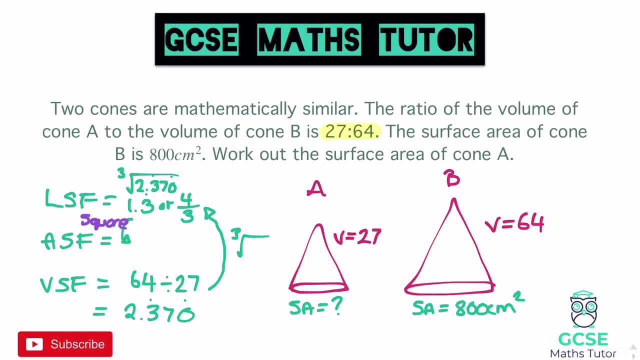 So we want four thirds squared or 1.3 recurring squared, So square answer equals and you get 1.7 recurring. Not very nice at all this question. There we are. So 1.7 recurring is the scale factor that we need there: 1.7 recurring. 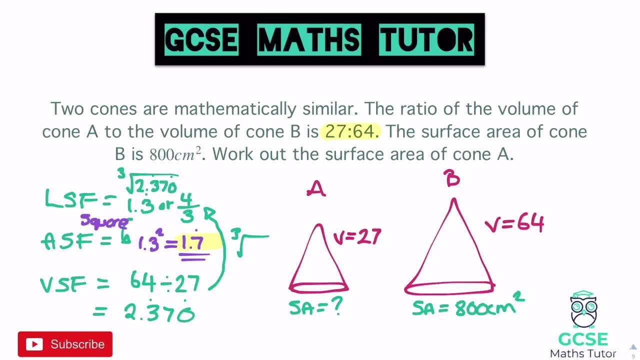 OK, so a little bit nasty there. Obviously it's already quite difficult moving between the lengths of all human area scale factors. You just have to be very careful, when these decimals do come up on your calculator, that you just keep using the answer on your calculator screen. 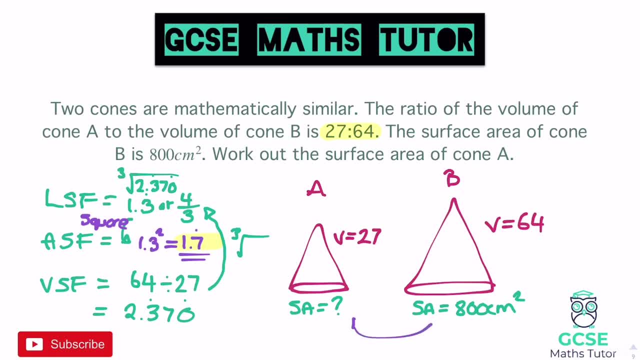 But from here it's nice and easy. So, from the big down to the small, we're using the area scale factor. big to small, We're going to divide. So divide by 1.7, recurring. So what I would do is leave 1.7 recurring on your calculator screen. 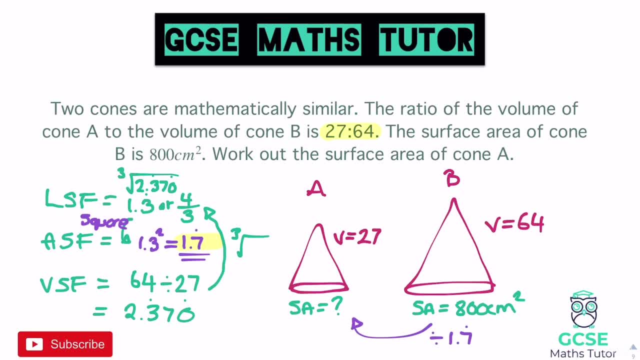 type in 800, divide by and again use the answer button. It will just put that 1.7 recurring in for you. So 800 divided by answer and you should get 450.. So just make sure that you can do that on your calculator. 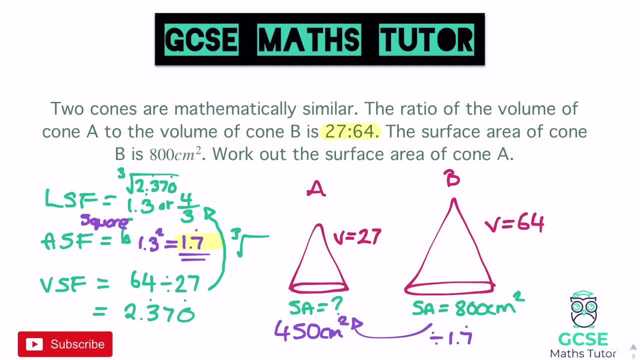 450 centimetre squared, and obviously that's our final answer. just goes to show how it goes, to show you a little bit how that answer button can be used and how it can be really helpful to make sure you don't get any rounding errors if you don't get bang on 450.. 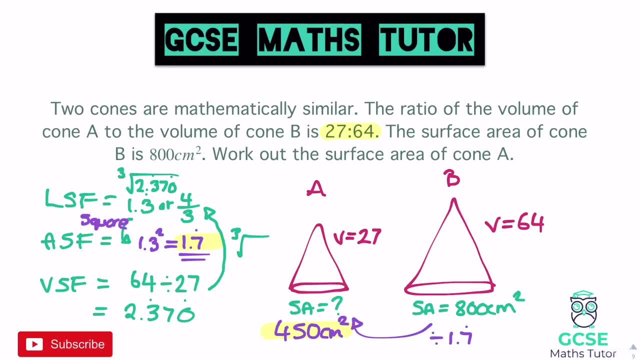 You need to have a little go with the calculator. Make sure you can find these buttons OK. so we've been using the square root, the cube root, the square, the cube button, and then also starting to use the answer button there. OK, so just a little side note. 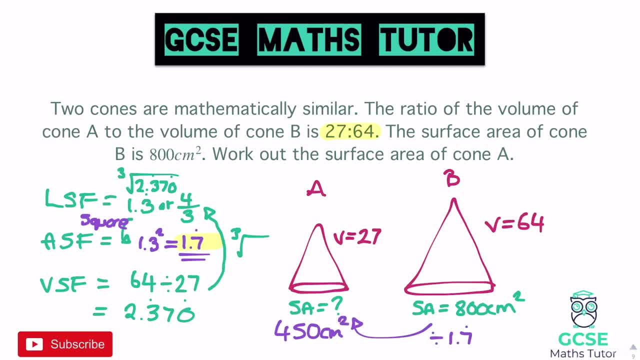 One hundred and fifty centimetre squared, And obviously that's our final answer. It just goes to show how it goes, to show you a little bit how that answer button can be used and how it can be really helpful to make sure you don't get any rounding errors if you don't get bang on four hundred and fifty. 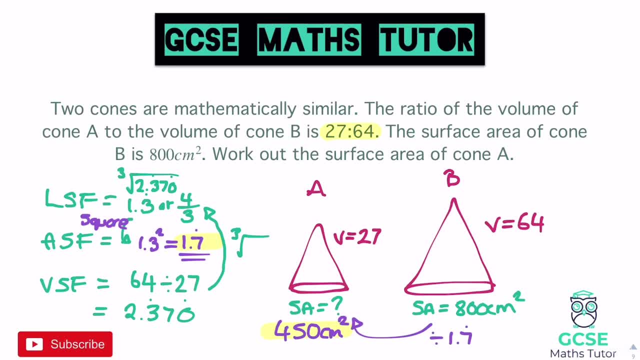 You need to have a little go with the calculator. Make sure you can find these buttons OK. so we've been using the square root, the cube root, the square, the cube button, and then also starting to use the answer button there. OK, so just a little side note what I typed into my calculator. 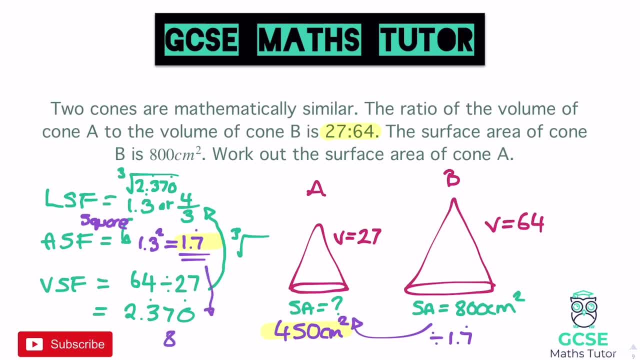 Once I had the one point seven, I typed in eight hundred divided by and then press the answer button which has ANS on it like that, And that did eight hundred divided by one point seven. recurring for me, Right. OK, here's some for you to have a go at. 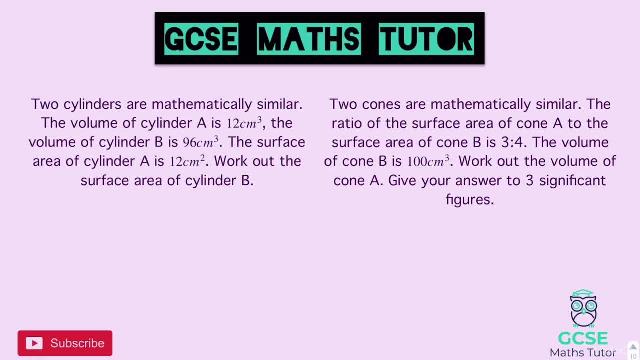 OK, so there's two questions there, one with alter ratio and one with a ratio. Just be careful with your calculator, obviously moving between your length, area and volume scale factor. So, first things first, I would definitely make sure you write all of these down because you are going to be moving between the three. 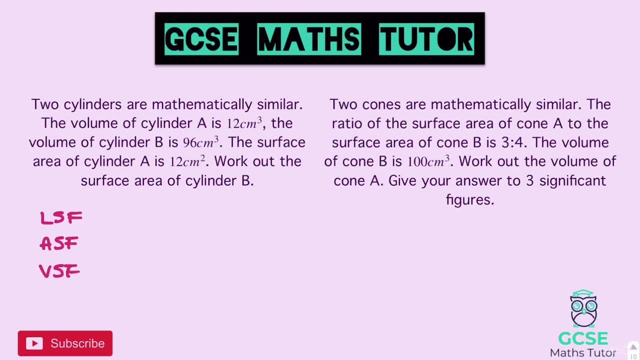 Length area, volume. Identify in each question which one you can work out straight away whether you've been given areas or volumes and then move between the two so you can get the one that you need. OK, right, So pause the video. there have a go. 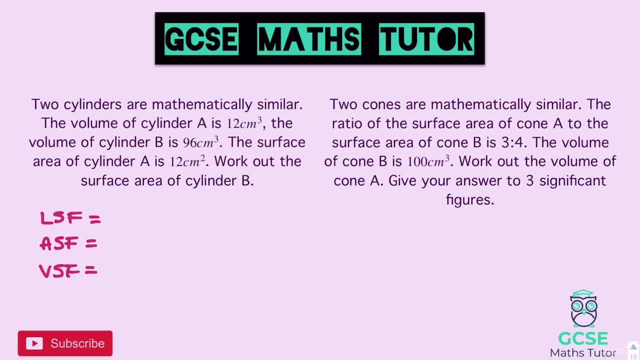 We'll go over the answers in a sec. OK, so the first one: now you've been given what looks like some volumes, So we've got volume is twelve and ninety six. So the first thing I can do is I can do ninety six divided by twelve in my volume scale factor. 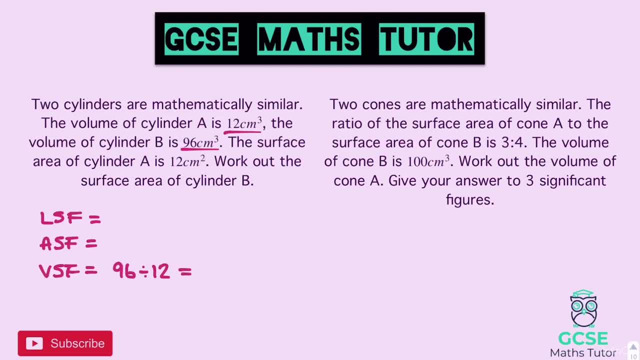 Ninety six divided by twelve is eight. So that's a nice one, because eight's a cube number. So, to return back to length, the cube root, So the cube root. So the cube root of eight, which we shouldn't need a calculator for, is two. 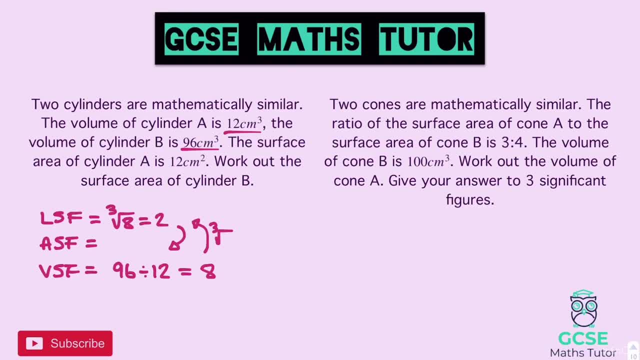 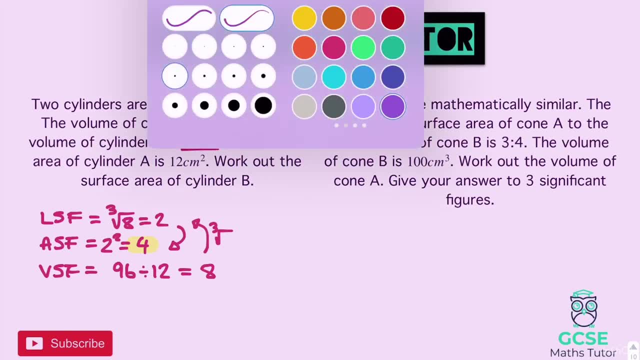 And then we can get back down to area by squaring. So two squared equals four. There we go, And there's a scale factor we're going to be using in this question. So now we have the scale factor. We just need to think: are we going from the small to the big or big to the small? 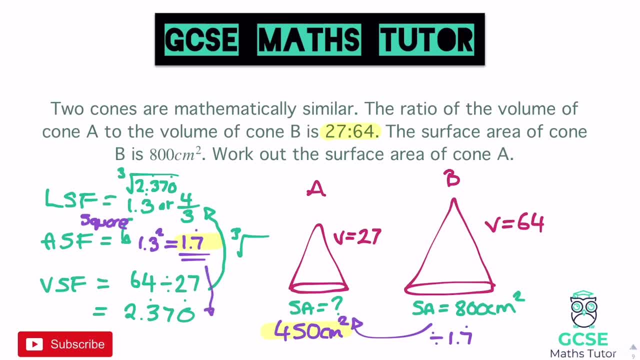 What I typed into my calculator once I had the 1.7, I typed in 800 divided by 1.7 and then pressed the answer button which has ANS on it like that, And that did 800 divided by 1.7, recurring for me. 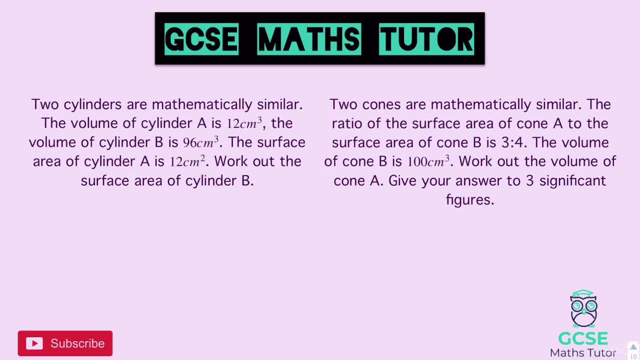 Right, OK, here's some for you to have a go at. OK, so there's two questions there, one with alter ratio and one with a ratio. OK, so just be careful with your calculator, obviously, moving between your length, area and volume scale factor. 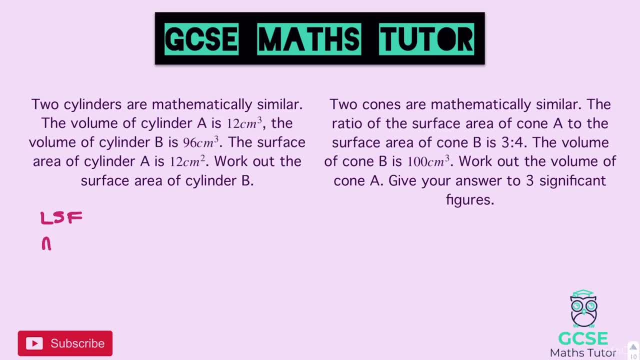 So, first things first. I would definitely make sure you write all of these down, because you are going to be moving between the three Length area volume. Identify in each question which one you can work out straight away whether you've been given areas or 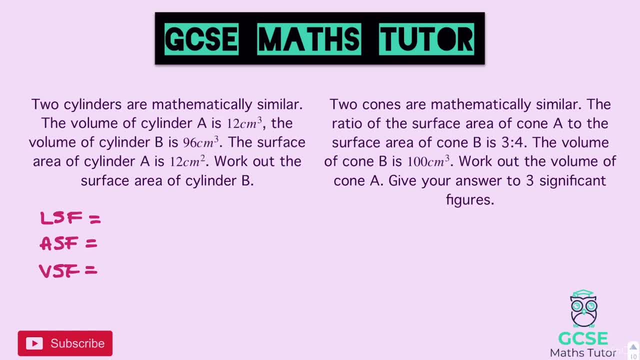 volumes and then move between the two so you can get the one that you need. OK, right, so pause the video there. have a go. We'll go over the answers in a sec. OK, so the first one. now you've been given what looks like some volumes. 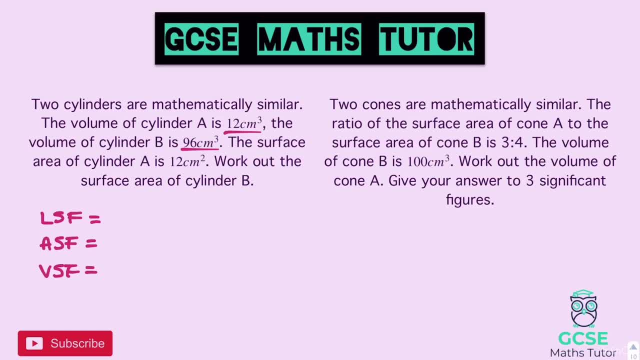 So we've got: volume is 12 and 96. So the first thing I can do is I can do 96 divided by 12. in my volume scale factor, 96 divided by 12 is 8.. So that's a nice one, because 8 is a cube number. 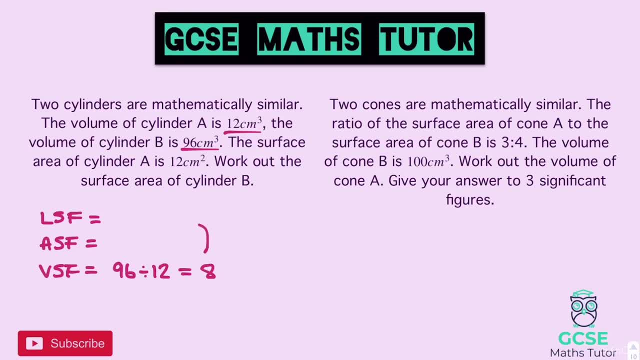 So I can turn back to lengths. I can do a cube root, So cube root, So the cube root of 8, which we shouldn't need a calculator for- is 2.. And then we can get back down to area by squaring. 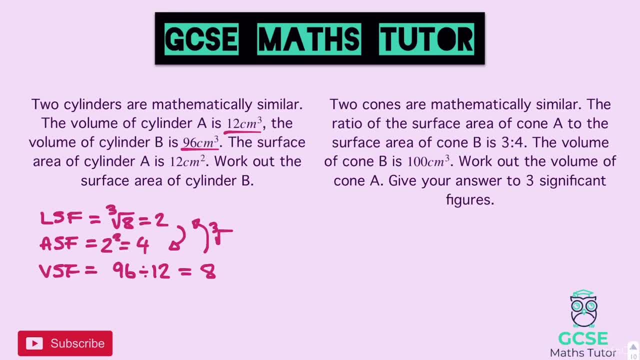 So 2 squared equals 4.. There we go, And there's a scale factor we're going to be using in this question. So now we have the scale factor. We just need to think: are we going from the small to the big or big to the small? 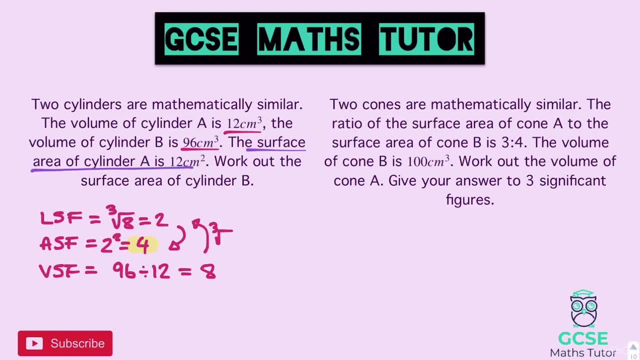 So we've been given the surface area of A, which is 12, which is the smaller one. So 12 is my surface area, So 12.. We're going to multiply that by our scale factor, which is 4.. So 12 times 4 is 48. 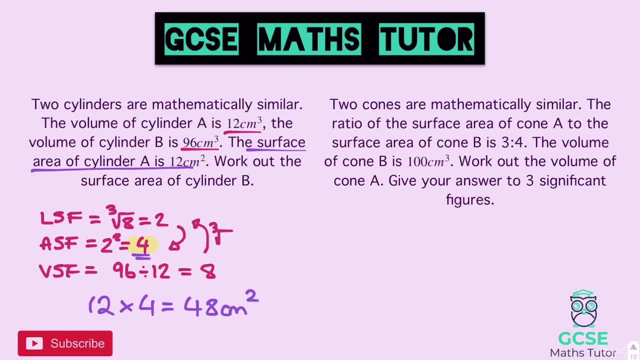 centimetres squared The surface area. there, There we go, And that is our final answer. Let's highlight that: 48 centimetres squared. OK, looking at the next one Now it says two cones are mathematically similar. 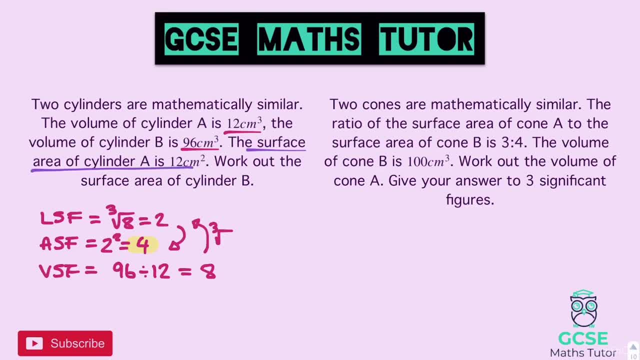 So we've been given the surface area of A, which is twelve, which is the smaller one. So twelve is my surface area, So twelve. we're going to multiply that by our scale factor, which is four. So twelve times four is forty eight centimetres squared. 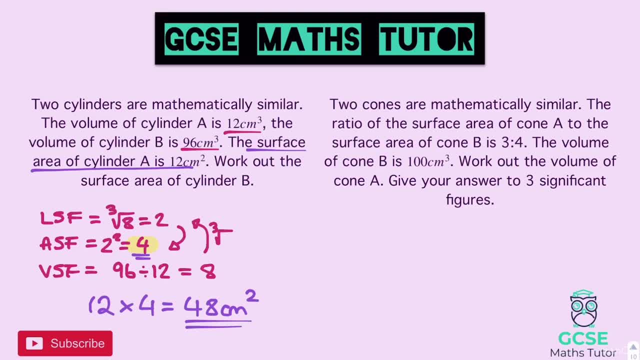 The surface area. there, There we go, And that is our final answer. Let's highlight that. Forty eight centimetres squared. Okay, looking at the next one Now, it says two cones are mathematically similar: The ratio of the surface area. 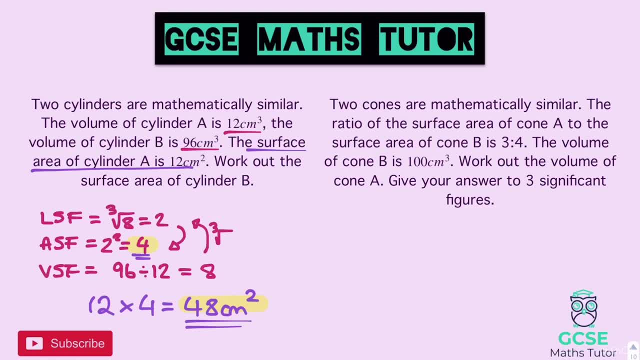 A to B is three to four and then it gives us a volume, So three to four. So let's imagine A is three and B is four And let's start working out our scale factors. So that's a surface area that we've been given there. 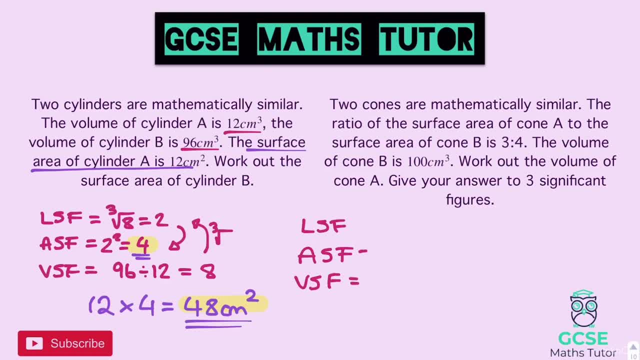 Let's just write all these down. Now we can work out the area scale factor there, because we've got the big one, which is four divided by three, with a smaller one, And that gives us four thirds or one point three recurring. There we go Probably just leave it as four thirds, but there we are. 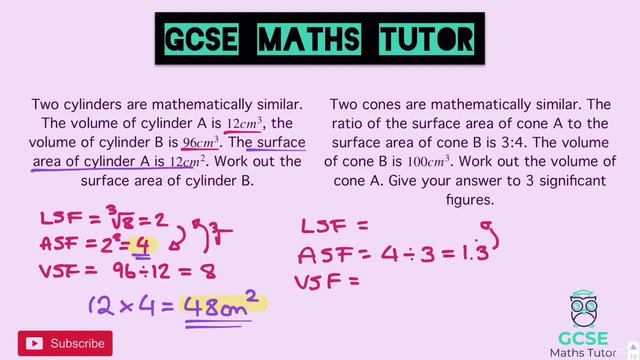 Right, So that's an area So we can go back to lengths by square rooting. So if I square root that, I should type that in. So four divided by three is four thirds Square root, my answer, And I get something really horrible here. 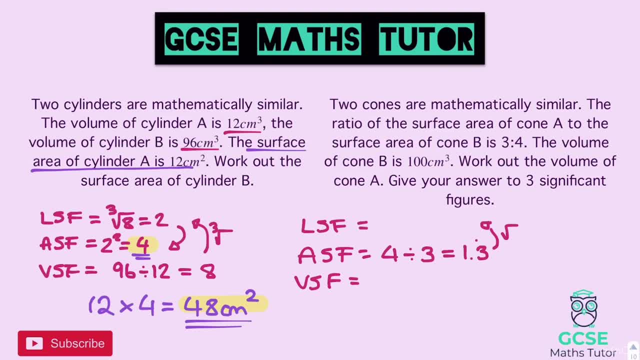 I actually get this horrible third on my screen, or this big long decimal. So that gives me- I want to do the square root of one point three- recurring. I get a really horrible decimal here. Let's see if I can write it all in. Let's get rid of that bit. 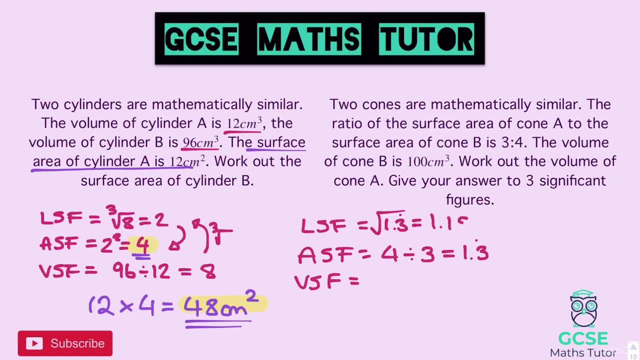 I get one point: one, five, four, seven, zero, zero, five, three, eight. There we go. So that's the horrible decimal that I get. Now we're looking at volume, So I'm going to leave that on my calculator screen. I'm going to get down to volume. 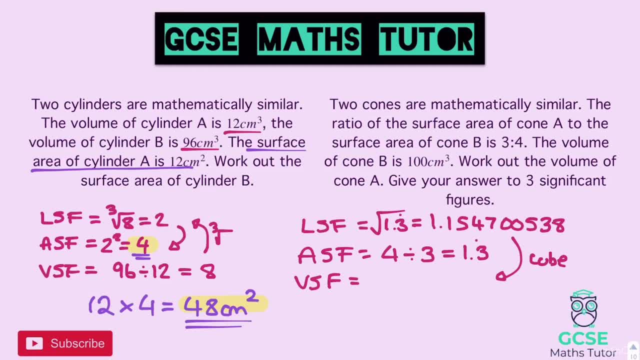 I'm going to cube that. So I'm just going to press the X cubed button or answer cubed. There we go And again I get a really horrible decimal. So cubing that gets me- And I can't even write that all down cube, because it's such a horrible number. 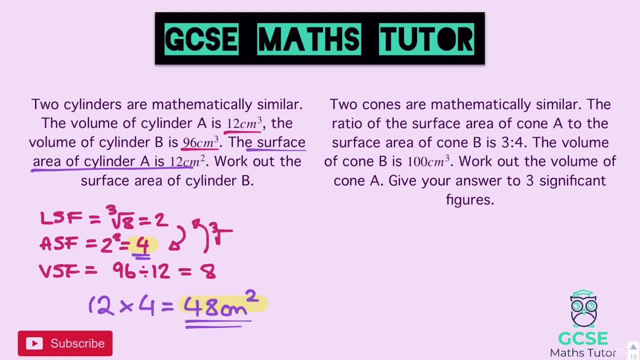 The ratio of the surface area of A to B is 3 to 4. And then it gives us a volume, So 3 to 4.. So let's imagine A is 3 and B is 4. And let's start working out our scale factors. 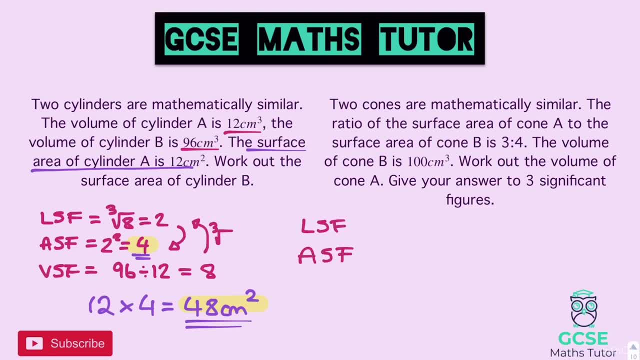 So that's a surface area that we've been given there. Let's just write all these down. Now we can work out the area scale factor there, because we've got the big one, which is 4,, divided it by 3 with a smaller one, and that gives us four thirds. 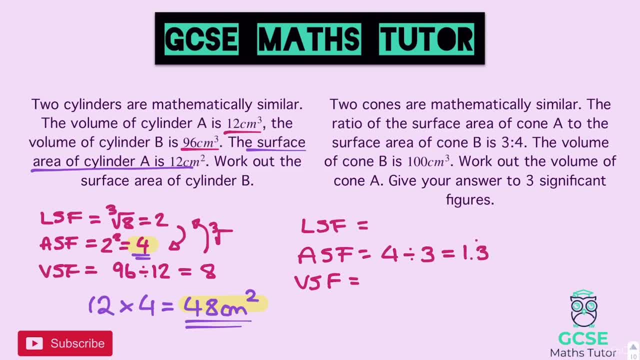 or 1.3 recurring. There we go. I'd probably just leave it as four thirds, but there we are, Right, So that's an area. So we can go back to lengths by square rooting. So if I square root that, I should type that in. 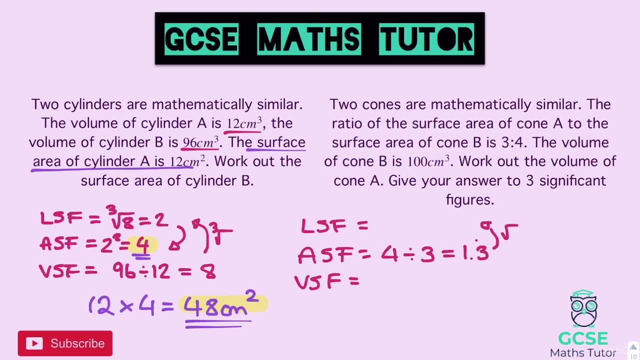 So 4 divided by 3 is four thirds Square root. my answer, And I get something really horrible here. I actually get this horrible third on my screen, or this big long decimal. So that gives me I want to do the square root of 1.3 recurring. 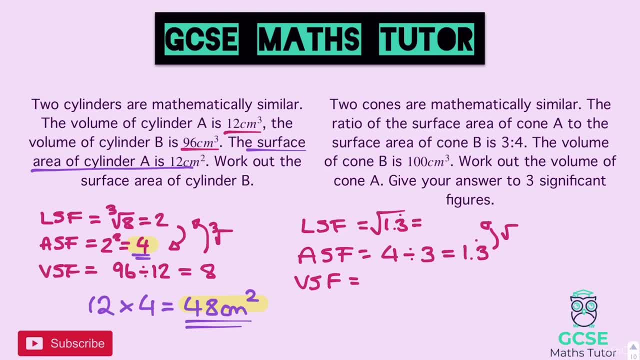 I get. I get a really horrible decimal here. Let's see if I can write it all in. Let's get rid of that bit. I get 1.154700538.. There we go. So that's the horrible decimal that I get. 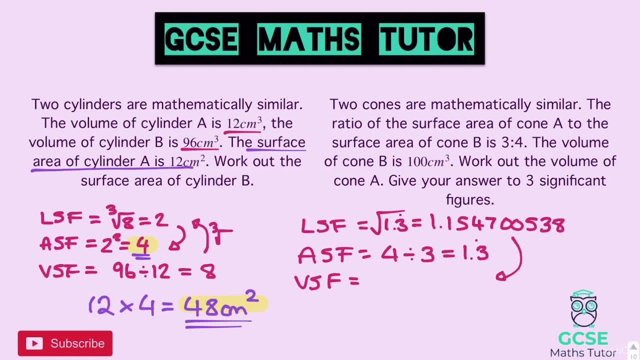 Now we're looking at volume. so I'm going to leave that on my calculator screen. I'm going to get down to volume. I'm going to cube that. So I'm just going to press the X cubed button or answer cubed. 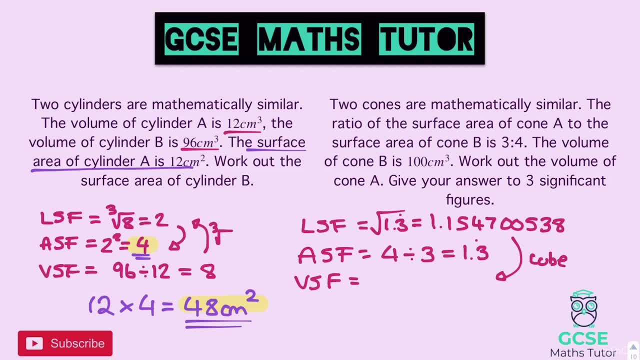 There we go And again I get a really horrible decimal. So cubing that gets me- and I can't even write that all down, cubed because it's such a horrible number- but 1.539600718.. OK now, good thing about this question is: 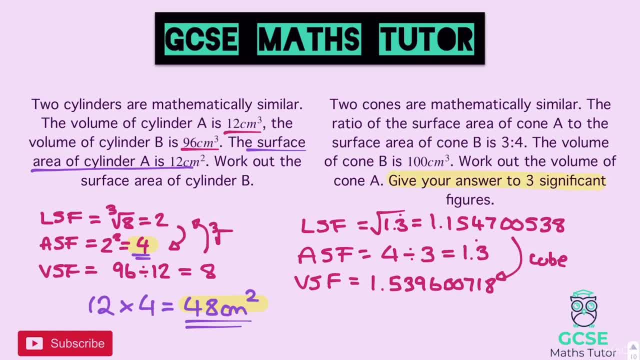 there's a massive hint that you're going to get horrible numbers. Look, it says: give your answer to three significant figures. So that obviously gives us a massive hint that you are going to get horrendous decimals in this one, And you do. 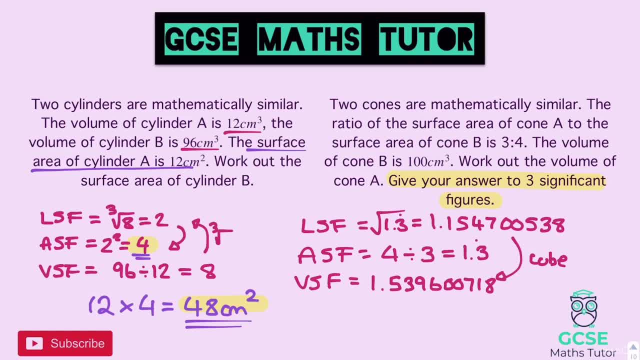 You get 1.539600718 as your volume scale factor. Now it says we're moving from the volume of B down to A. B is the larger shape there. So if we've got A to B, let's have a look. 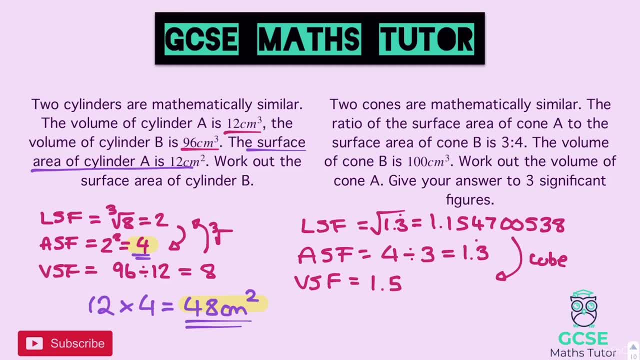 But one point, five, three, nine, six, zero, zero, seven, one, eight. OK, now good thing about this question is there's a massive hint that you're going to get horrible numbers. Look, it says: give your answer to three significant figures. So that obviously gives us a massive hint. 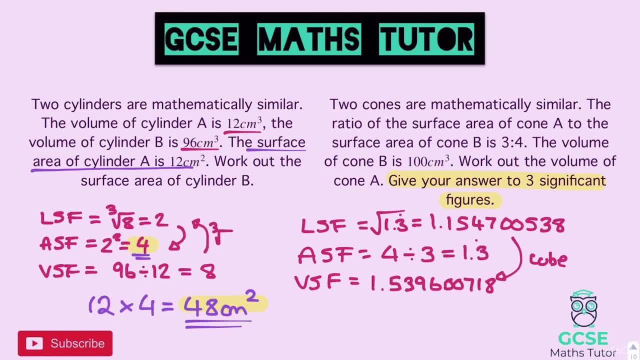 that you are going to get horrendous decimals in this one. And you do get one point five, three, nine, six, zero, zero, seven, one, eight as your volume scale factor. Now it says we're moving from the volume of B down to A. B is the larger shape there. 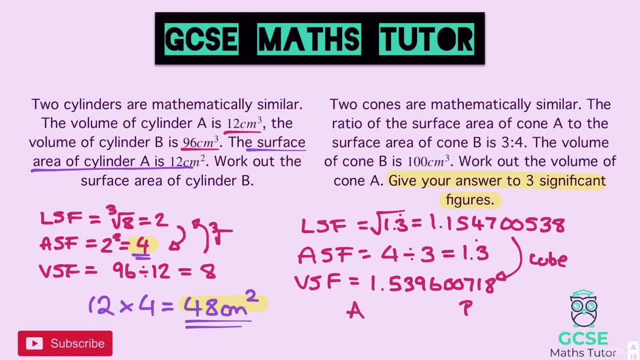 So if we've got A to B, let's have a look A and B And it says that B is one hundred centimetre cubed. So to get back to A, we are going to have to divide by that scale factor. 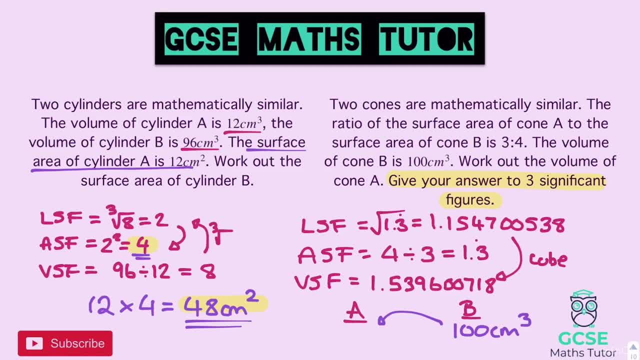 And that scale factor is the one point five, three, nine. horrible thing. So let's just work. Let's get out one hundred divided by answer on the calculator. I'm just going to put divide here and we get sixty four point nine, five one. 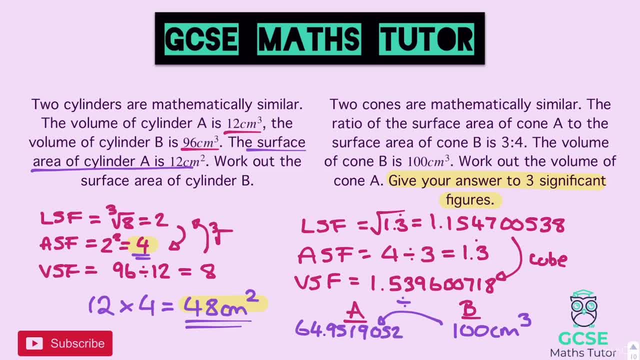 Nine, oh, five, Two, eight. Now another question says to give it to three significant figures. But when you're doing your work- and I always just make sure you write down all of the digits before you decide to do any rounding- Now, three significant figures chops it off after the nine, six, four, nine. 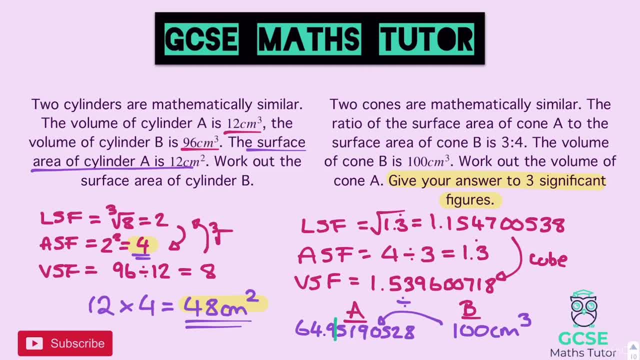 That's the third significant figure And after the nine it's a five. This is one of those weird rounding scenarios where it actually sends that decimal up to a nought and rounds to sixty four, to sixty five. So my answer: See if we can fit this in anywhere. 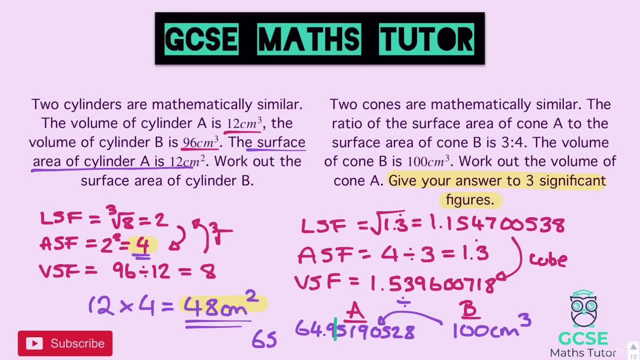 Will be sixty five, And because there's no third significant figure there, I have to put point zero in. So sixty five point zero centimetres cubed Can't really fit that in. I might have to write it somewhere else. There we go, But our final answer there is. 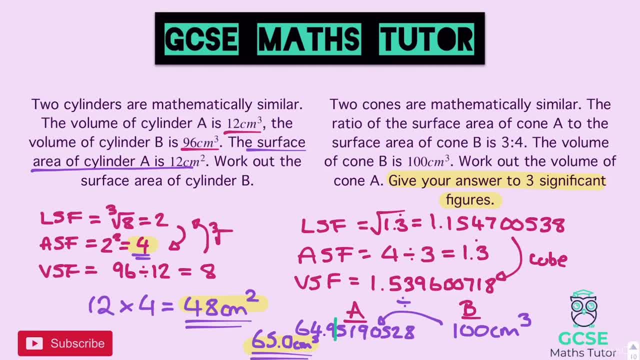 sixty five point zero centimetre cubed is our final answer. OK, so just watch out with that rounding scenario. if your third significant figure, or whatever it's asking you to round, is a zero, do you need to make sure you put that in, to make sure it's definitely? 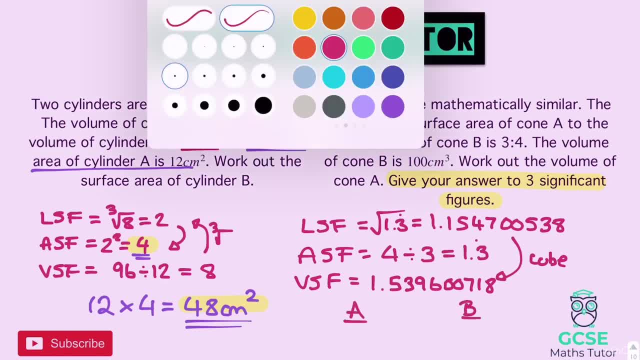 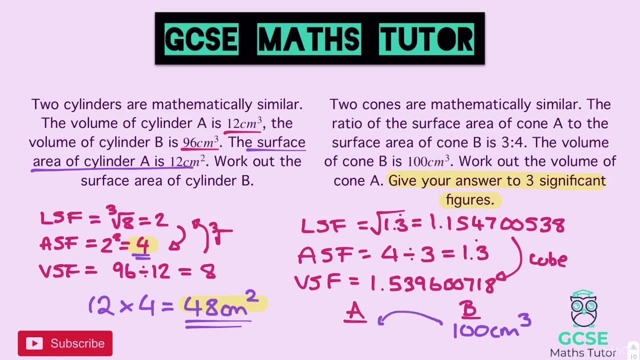 A and B And it says that B is 100 centimetre cubed. So to get back to A, we are going to have to divide by that scale factor And that scale factor is the 1.539 horrible thing. So let's just work that out. 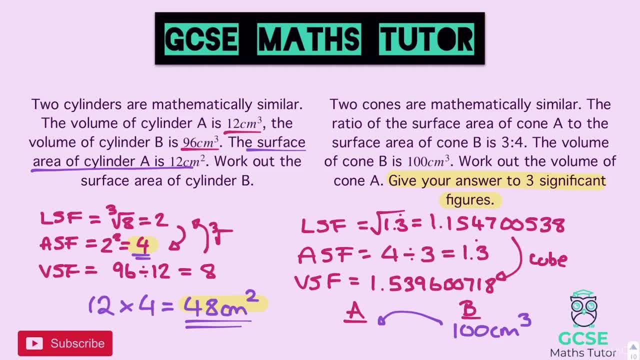 100 divided by answer on the calculator. I'm just going to put divide here and we get 64.95190528.. Now I know the question says to give it to three significant figures, But when you're doing your work- and I always just make sure you write down all- 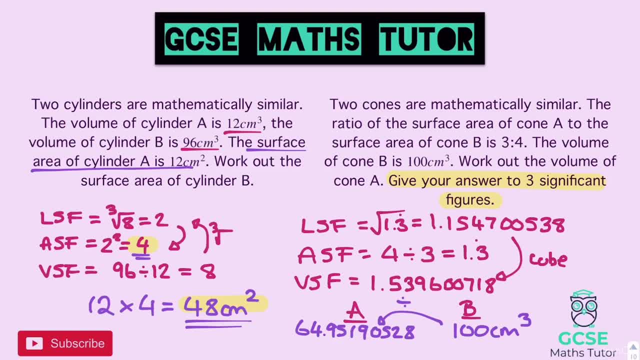 of the digits before you, So I do any rounding. Now three significant figures chops it off. after the nine: six, four, nine: That's the third significant figure, And after the nine it's a five. This is one of those weird rounding. 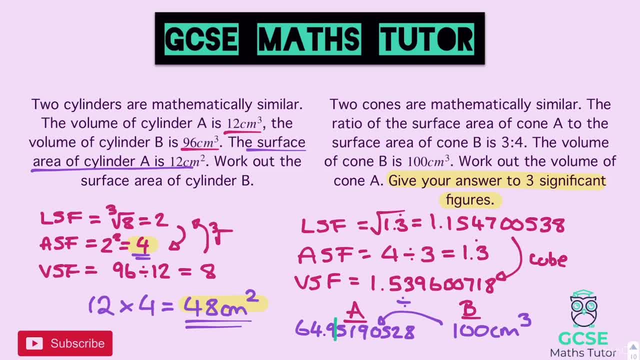 scenarios where it actually sends that decimal up to a nought and rounds the 64 up to 65. So my answer- see if we can fit this in anywhere- will be 65. And because there's no third significant figure there, I have to put 0.0 in. 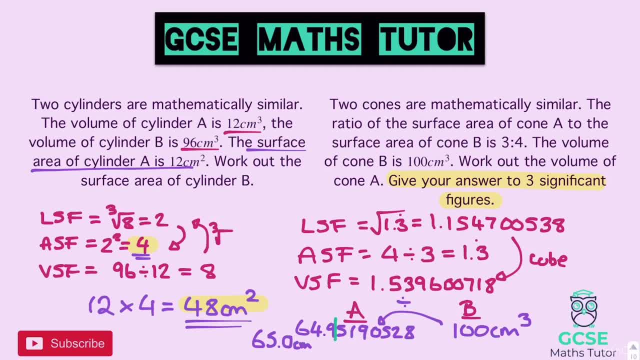 So 65.0.. Centimetres cubed Can't really fit that in. I might have to write it somewhere else. There we go, But our final answer there is: 65.0 centimetre cubed is our final answer. 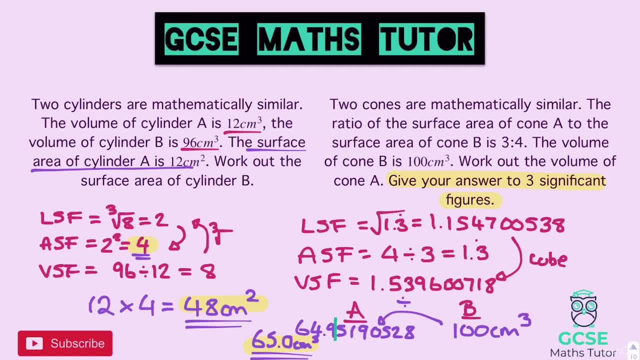 OK. so just watch out with that rounding scenario. If your third significant figure, or whatever it's asking you to round, is a zero, Do you need to make sure you put that in, to make sure it's definitely three significant figures, Right? OK, so let's have a look at one more thing before we finish. 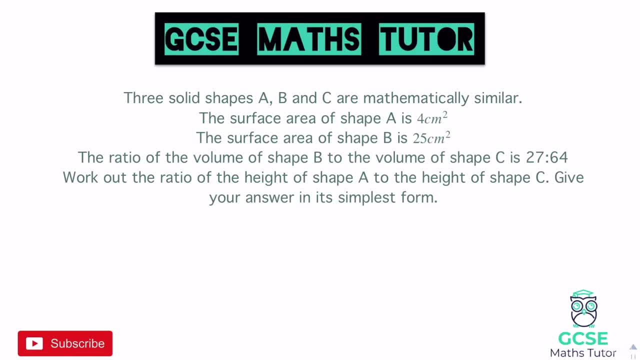 OK. so this question says three solid shapes, A, B and C, are mathematically similar. The surface area of A is four centimetres squared. The surface area of B is 25 centimetres squared. It says the ratio of the volume of shape B to the volume of shape C is 27 to 64.. 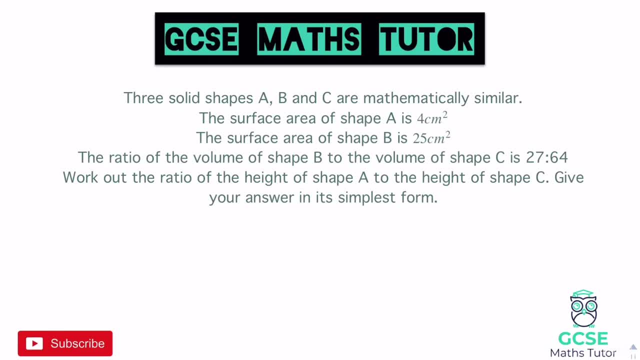 Work out the ratio of the height of shape A to the height of shape C and give your answer in its simplest form. Now, this is slightly different. OK, it's not actually asking us to work out any surface areas, but it's bringing in this sort of ratio idea. 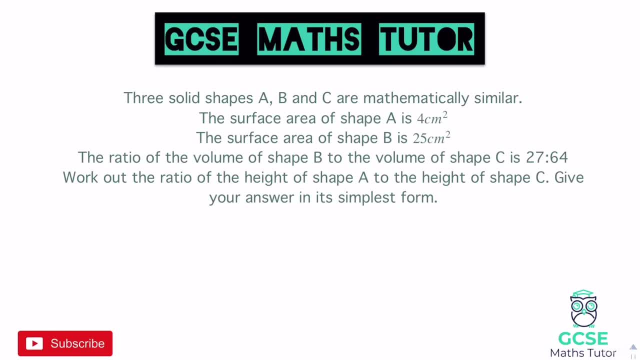 And this is quite a tricky question because we've got three different shapes. Now, whenever we've got three different shapes and it mentions ratios, we're going to have to do a three part ratio at some point. So there's a bit of a hint there that we're going to have to do a three part ratio. 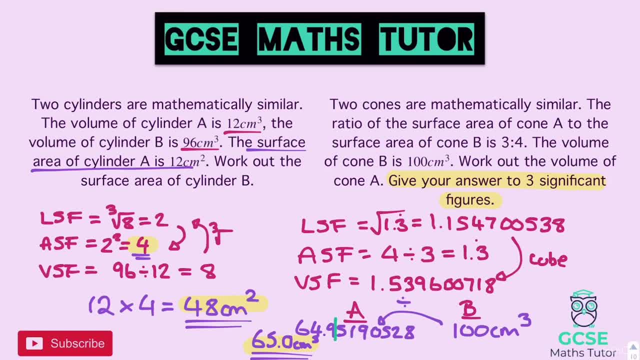 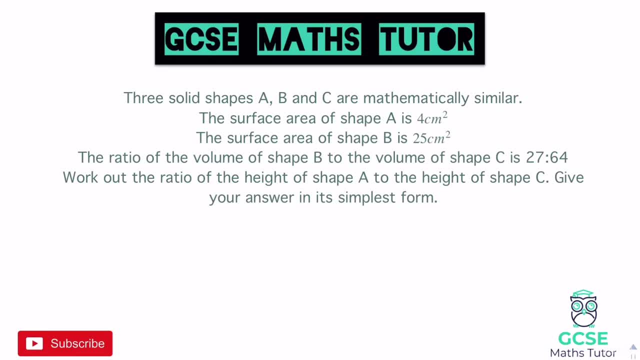 three significant figures, Right, OK? so let's have a look at one more thing before we finish. OK, so this question says three solid shapes: A, B and C are mathematically similar. Surface area of A is four centimetre. 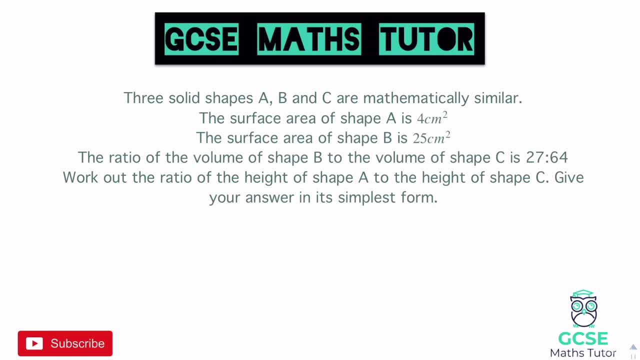 squared and surface area of B is twenty five centimetre squared. So the ratio of the volume of shape B to the volume of shape C is twenty seven to sixty four. Work out the ratio of the height of shape A to the height of shape C and give your. 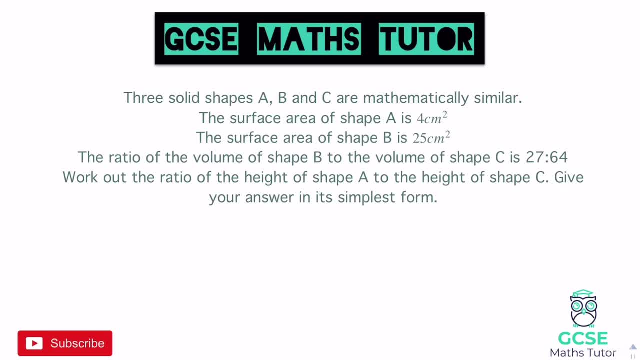 answer in its simplest form. Now, this is slightly different. OK, it's not actually asking us to work out any surface areas, but it's bringing in this sort of ratio idea. And this is quite a tricky question because we've got three different shapes. 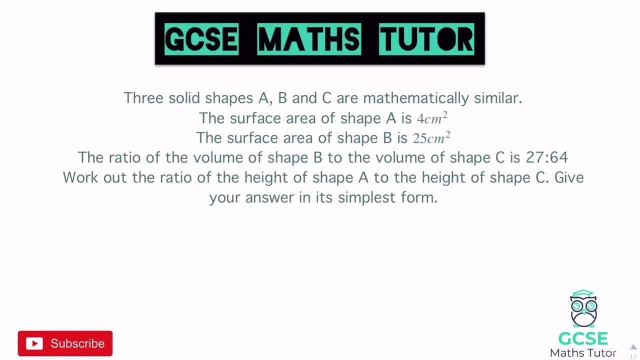 Now, whenever we've got three different shapes and it mentions ratios, we're going to have to do a three part ratio at some point. So there's a bit of a hint there that we're going to have to do a three part ratio. 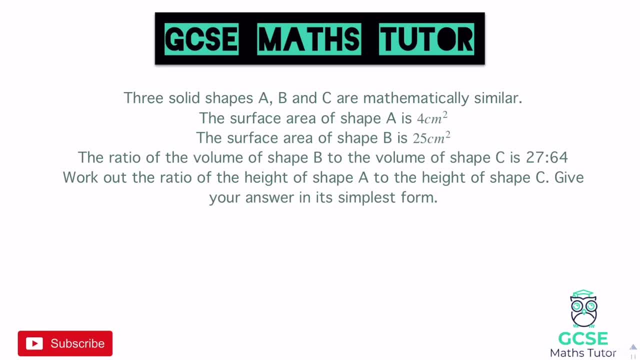 So we'll come to that in a little bit. Let's just have a look at how we tackle this sort of question Now. this first bit of information here gives us a surface area of four to twenty five here for A to B, And if I write that down as a ratio, look A to B. 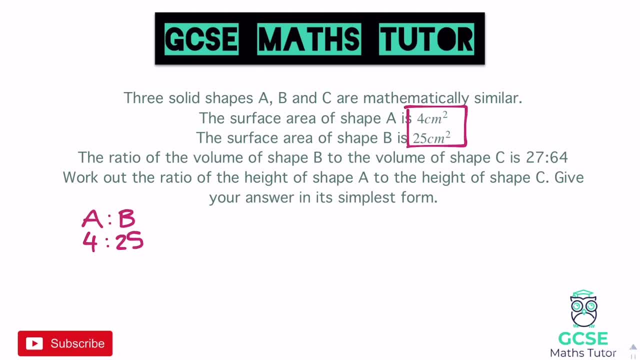 is four to twenty five, And what you might have noticed is- and this is what helps knowing these numbers- is that they're both square numbers and that is an area scale factor right there. So that's our area scale factor, OK, but it's in a ratio of four to twenty five. 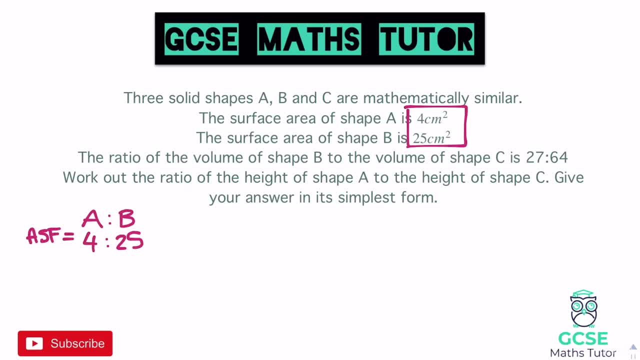 Now, if I want to get that back down to length, OK, how do we move from area to length? because it's asking us ultimately to work out the ratio of the height, which is the length. OK, it mentions, obviously, working out the 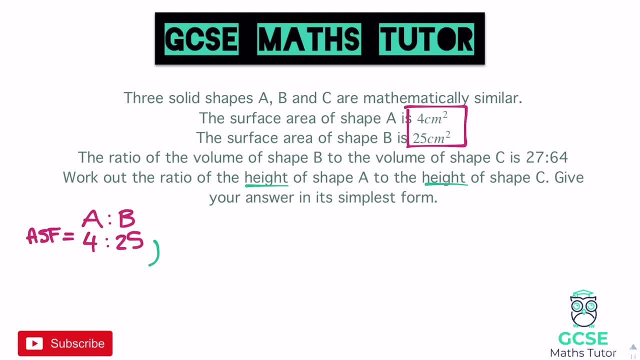 height. here I can move from area to length by square rooting. And if I square root both of those, it's going to give me a length scale factor. The square root of four is two and the square root of twenty five is five. 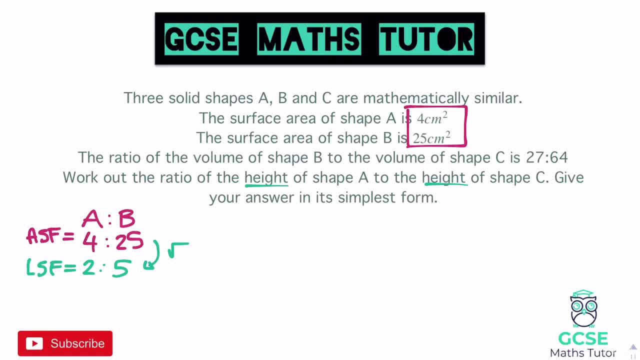 So my ratio of the length is two to five. If the ratio of the areas is four to twenty five, square rooting both of those gives me a length ratio of two to five. Now let's have a look at the other two. OK, so we've also got this bit of information here, where it says the volume. 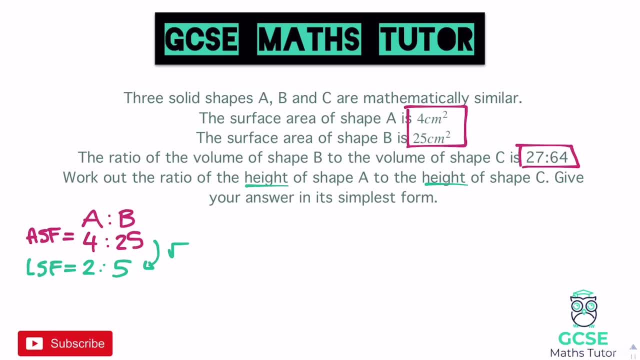 of B to C is twenty seven to sixty four, And again it gives us a massive hint there because they are cube numbers. So if I write that down as a ratio over here, B to C is twenty seven to sixty four And that is a volume scale factor. 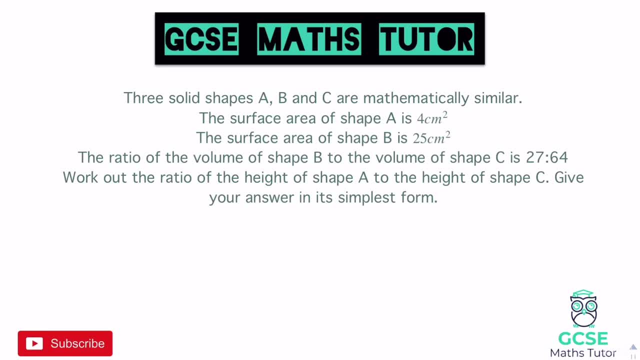 So we'll come to that in a little bit, But let's just have a look at how we tackle this sort of question Now. this first bit of information here gives us a surface area of 4 to 25 here for A to B. 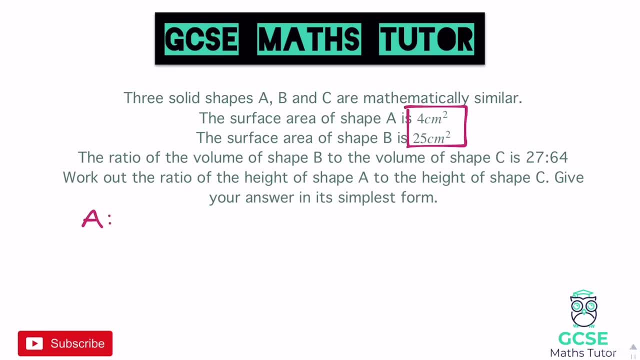 And if I write that down as a ratio, look: A to B is 4 to 25.. And what you might have noticed is- and this is what helps knowing these numbers- is that they're both square numbers and that is an area scale factor, right there. 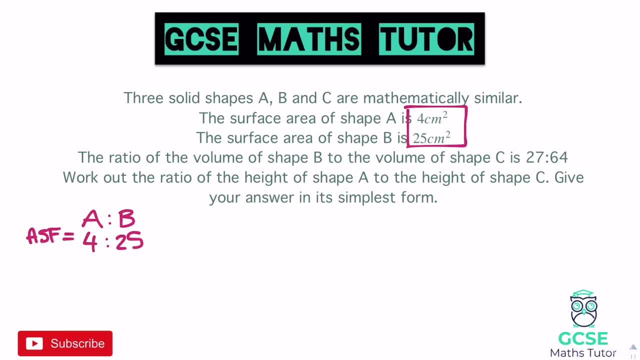 So that's our area scale factor. OK, So it's in a ratio of 4 to 25.. Now, if I want to get that back down to length, OK, how do we move from area to length? Because it's asking us ultimately to work out the ratio of the height. 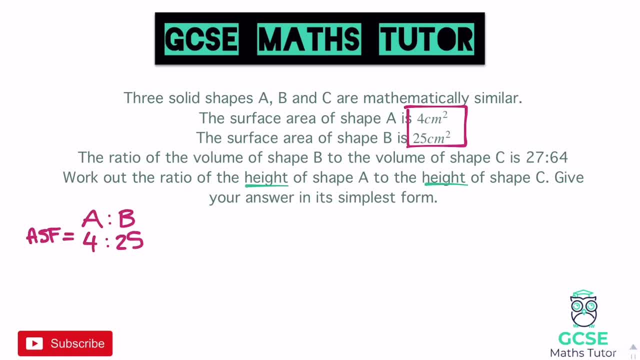 which is the length. OK, it mentions obviously working out the height. here I can move from area to length by square rooting And if I square root both of those, it's going to give me a length scale factor. The square root of 4 is 2 and the square root of 25 is 5.. 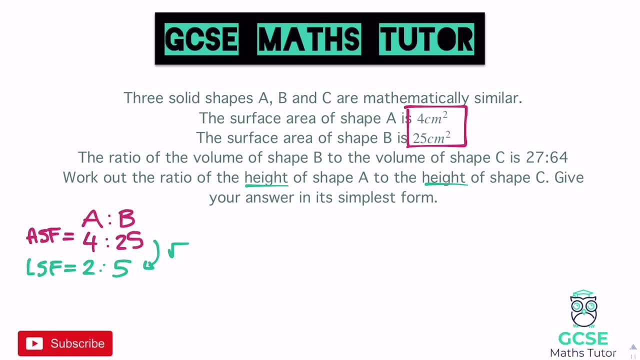 So my ratio of the length is 2 to 5.. If the area is 4 to 25, square rooting both of those gives me a length ratio of 2 to 5.. Now let's have a look at the other two. 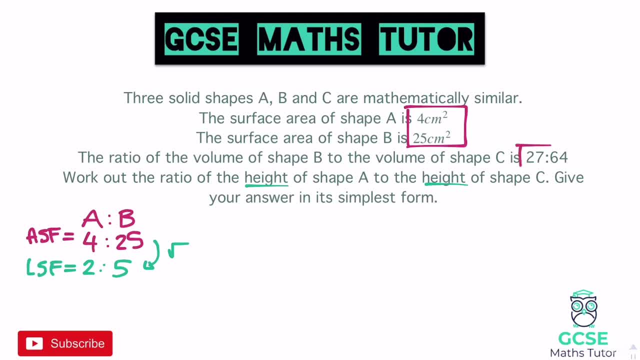 So we've also got this bit of information here where it says the volume of B to C is 27 to 64, and again it gives us a massive hint there because they are cube numbers. So if I write that down as a ratio over here, B to C is 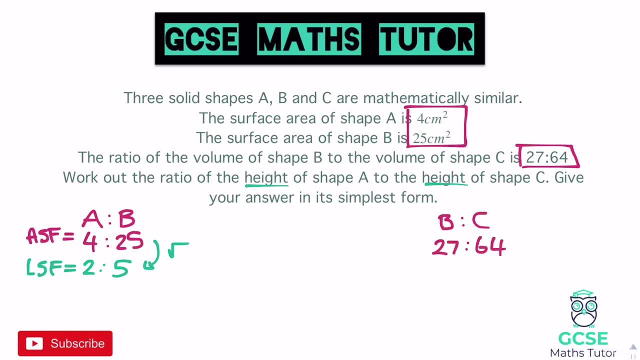 27 to 64, and that is a volume scale factor. The volume scale factor is 27 to 64.. And again, how do we get from volume back to length, The cube root? So we cube root that And that would give me a length scale factor. 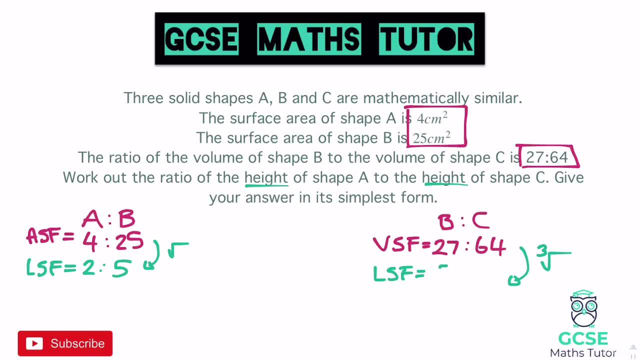 There we go. so my length scale factor is going to be: cube root of 27 is 3,, cube root of 64 is 4, and there we go. Now we have them both as a length scale factor. Now the next step. here it says: work out the ratio of the height of A to the height. 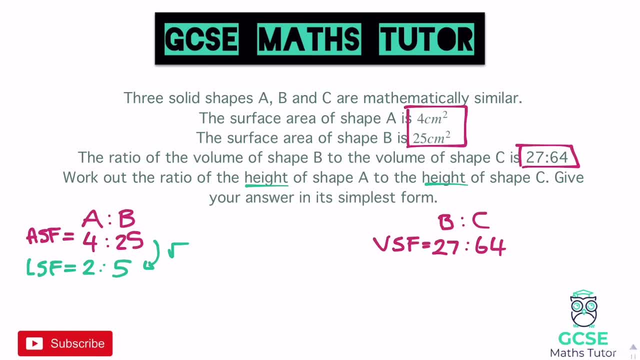 So my volume scale factor is twenty seven to sixty four. And again, how do we get from volume back to length, The cube root? So we cube root that and that would give me a length scale factor. There we go. so my length scale factor is going to be: cube root of twenty seven is: 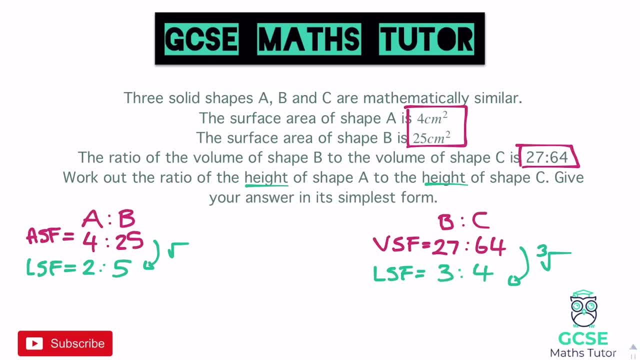 three. cube root of sixty four is four. And there we go. Now we have them both as a length scale factor. Now the next step. here it says: work out the ratio of the height of A to the height of C. So A is over here two and C is over here four. 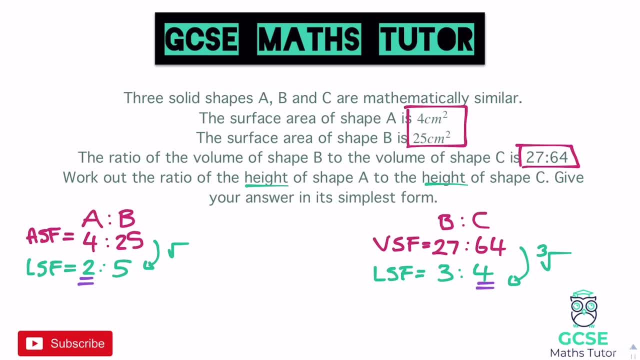 But it's not just as easy as saying two to four, And the reason behind that is these numbers for B are different. When those numbers are different, we can't combine these ratios, So those numbers have got to be the same And we can change these ratios however we like, just like we can do equivalent. 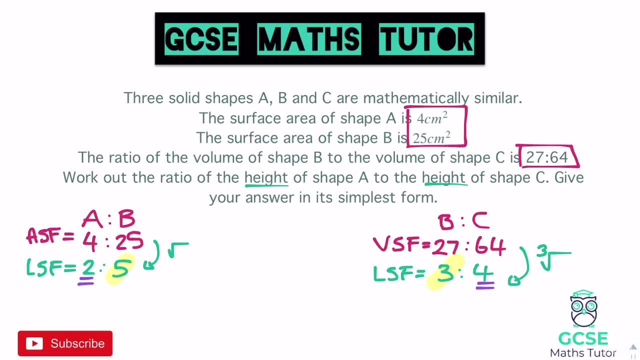 fractions. we can do equivalent ratios, can't we? So I can actually amend or change these ratios to make that number suit the number that I want. So if we line these all up and have a look what we've got at the moment, 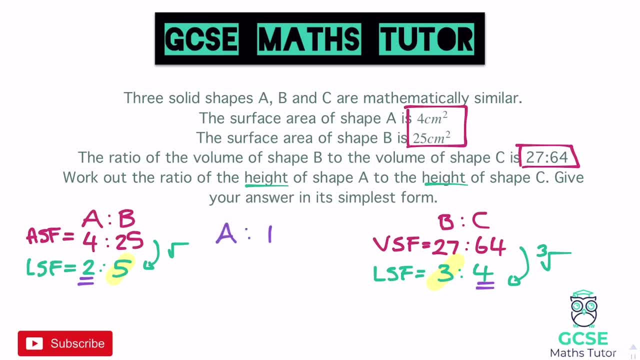 sometimes just piecing it all together can be really helpful. So we've got A to B to C. A to B, it's two to five- I can't write another number there in front of B, so I'm going to put it underneath- and B to C is currently three. 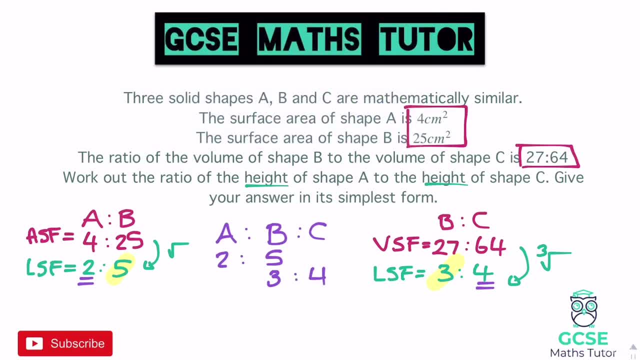 to four. OK, so in terms of actually making this number the same, look five and three. the closest number that I can turn them both into is fifteen. So to do that, I would have to multiply this top ratio, both the numbers- by three, and I'd have to multiply this bottom. 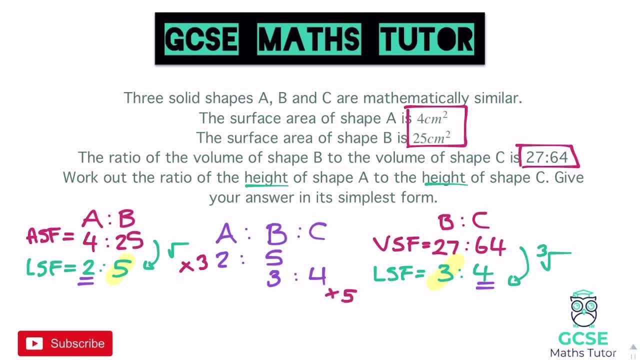 ratio, both the numbers by five. So if I multiply the top ratio there, two becomes six and five becomes fifteen. Multiplying the bottom ratio, the three to four, three becomes fifteen, which we've already got there, so we don't have to write that twice. 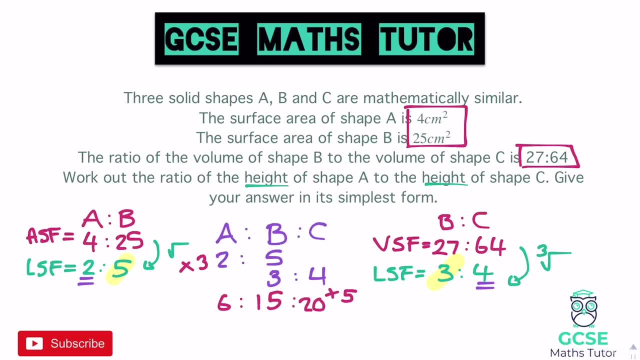 Four becomes twenty. There we go, So we've got six to fifteen to twenty. Now, obviously, the question only asked us to work out the ratio of the height of A to the height of C. And we've got those. now We've got six and twenty. 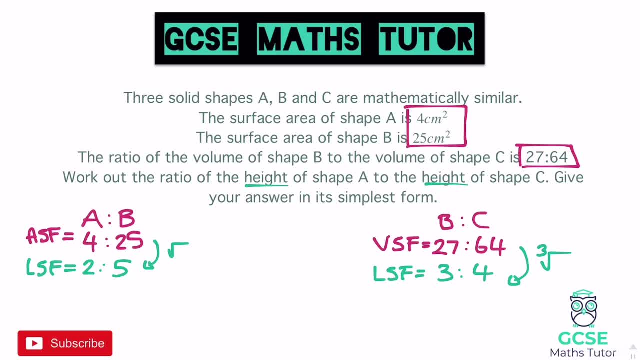 of C. So A is over here 2, and C is over here 4.. But it's not just as easy as saying 2 to 4.. And the reason behind that is these numbers for B are different. When those numbers are different, we can't combine these ratios. 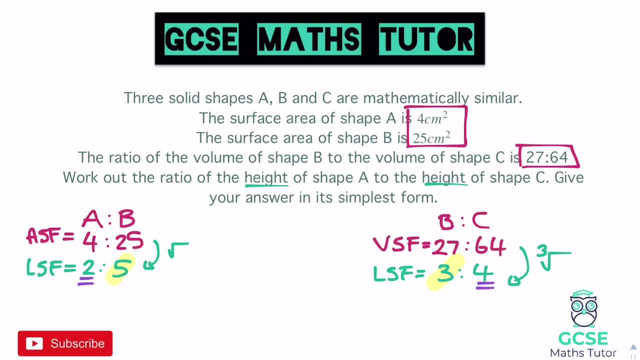 So those numbers have got to be the same And we can change these ratios however we like. just like we can do equivalent fractions, we can do equivalent ratios, can't we? So I can actually amend or change these ratios to make that number suit the number that I want. 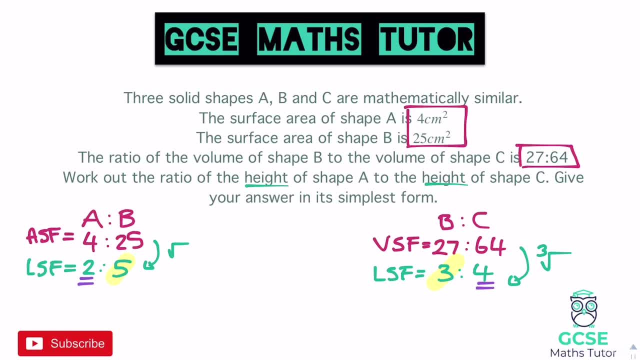 So if we line these all up and have a look what we've got at the moment, sometimes just piecing it all together can be really helpful. So we've got A to B to C, A to B is 2 to 5.. 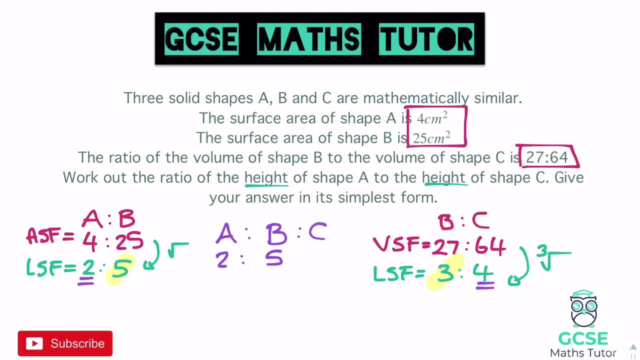 I can't write another number there in front of B, so I'm going to put it underneath, and B to C is currently 3 to 4.. OK, so in terms of actually making this number the same look 5 and 3,. 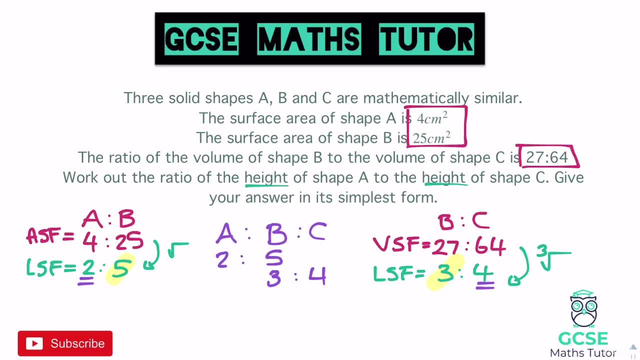 the closest number that I can turn them both into is 15.. So to do that, I would have to multiply this top ratio, both the numbers, by 3, and I'd have to multiply this bottom ratio, both the numbers, by 5.. 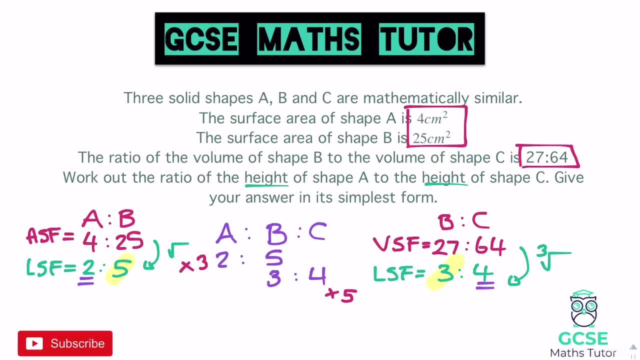 So if I multiply the top ratio there, 2 becomes 6 and 5 becomes 15.. Multiplying the bottom ratio, the 3 to 4,, 3 becomes 15, which we've already got there, so we don't have to write that twice- 4 becomes 20.. 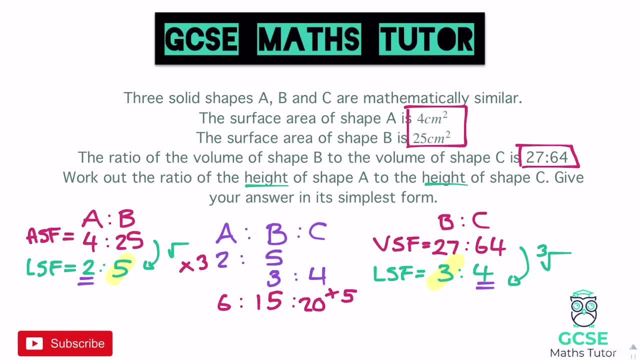 There we go, so we've got 6 to 15 to 20.. Now, obviously, the question only asked us to work out the ratio of the height of A to the height of C, And we've got those. now We've got 6 and 20.. 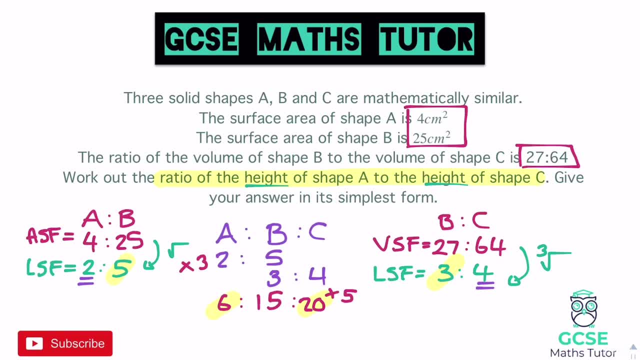 OK, that middle number is now the same. So actually the ratio of A to C, which, if I write over here A to C is 6 to 20.. OK, and it says: obviously, give it in its simplest form: 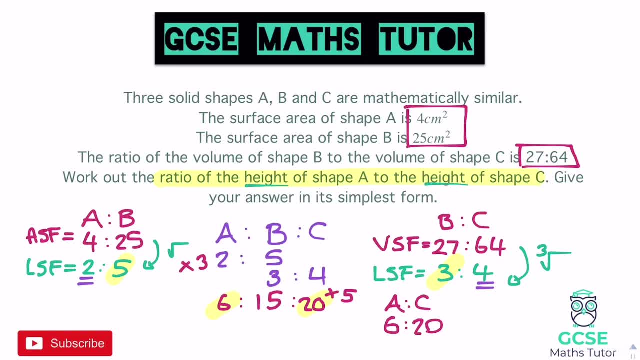 Both of those numbers divide by 2, so we can simplify the ratio: divide them both by 2, let's write that in and we get 3 to 10. And there is our final answer And there is the ratio of A to C.